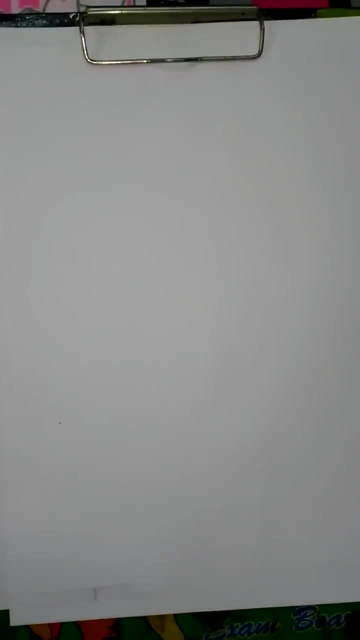 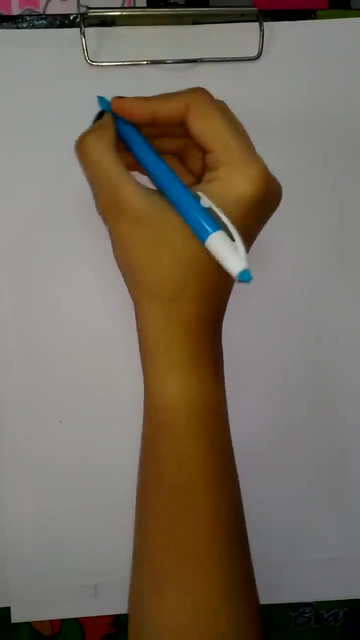 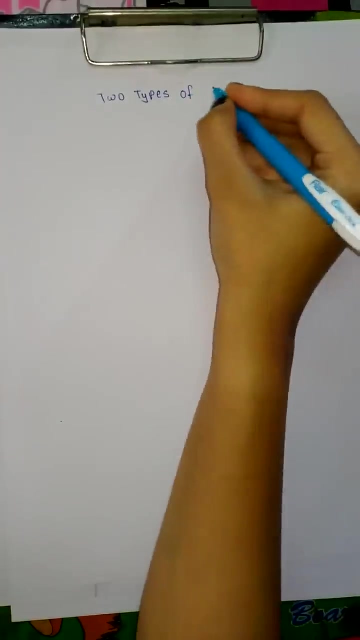 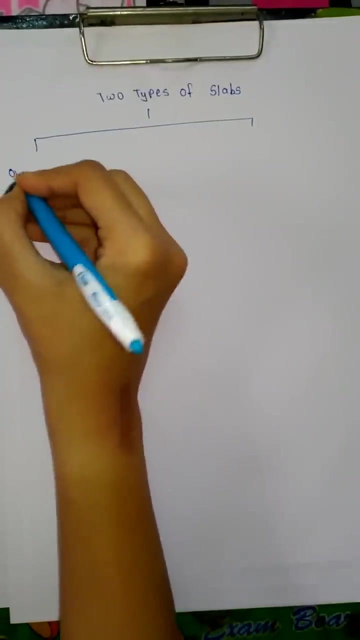 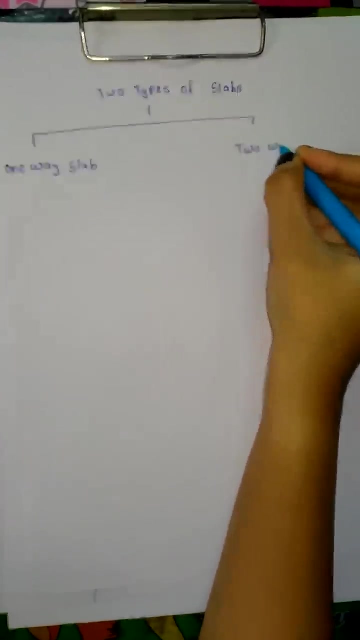 Hello friends, today I am going to talk about how the slab loads transfer to the beams. So to understand this, first of all, we have distinguish between types of slabs and we know that we have 2 types of slabs, And they are one way slab and two way slab. 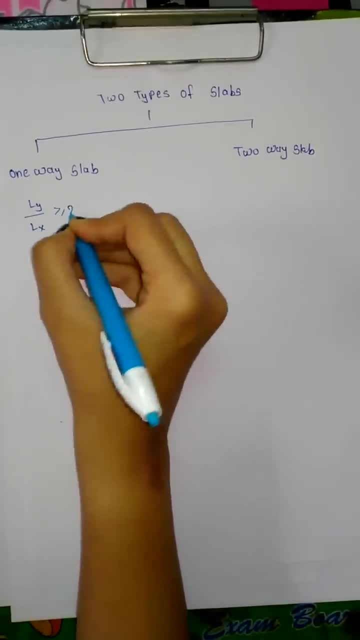 So if LY By LX is more than E, We have to reduce it by two. quería regime�� Ce 아이� arbeiten. we know that we have two types of slab and they are one way slab and two way slab. so if L Y by LX is more than, 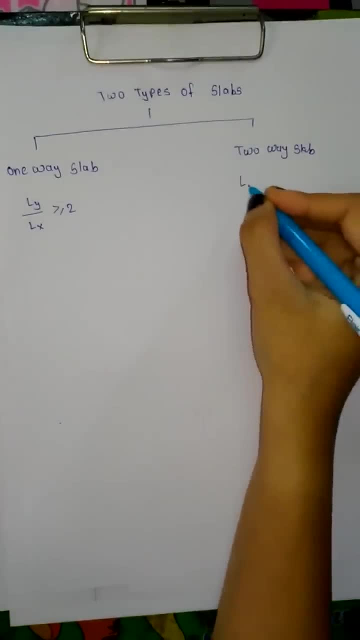 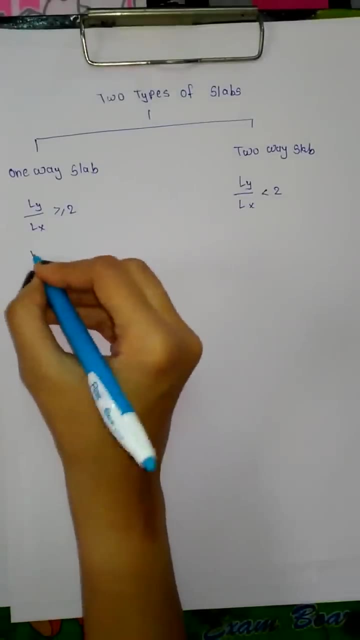 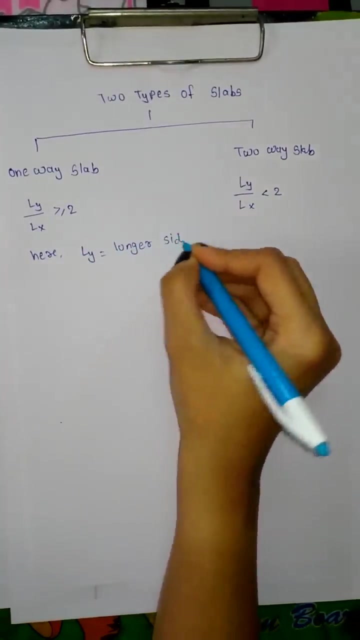 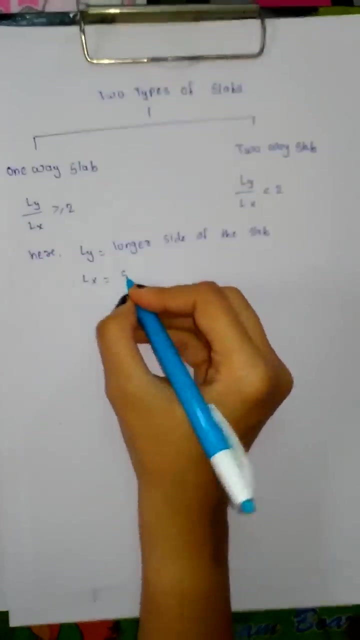 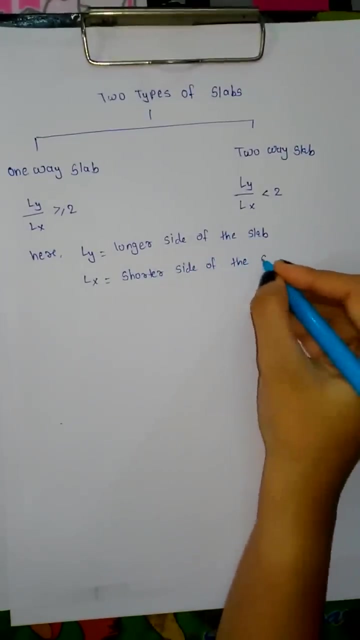 equal to 2 slab will behave as one way slab, and when Ly by Lx is less than 2 slab will behave as two way slab. So here you can see, Ly is denoted for the longer side of the slab and Lx will be denoted for the shorter side of the slab. Let's get understand with an. 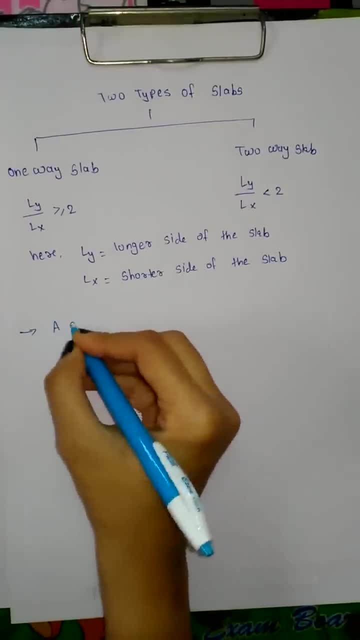 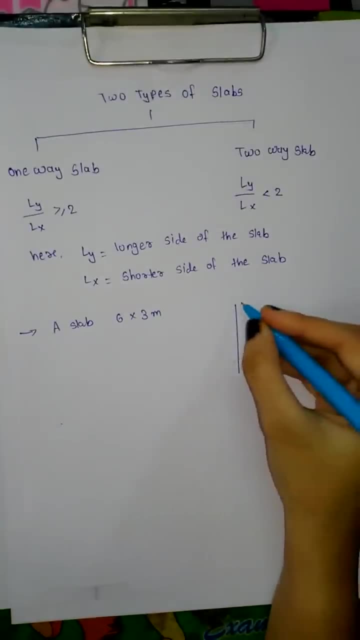 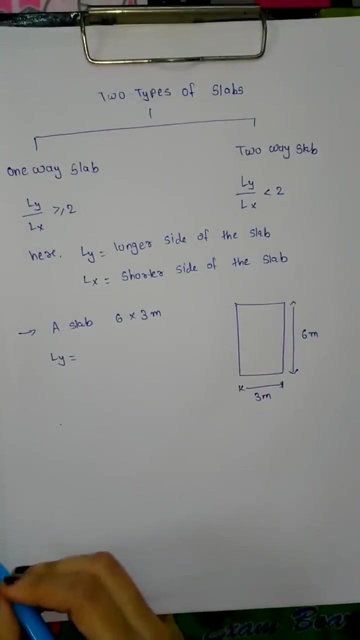 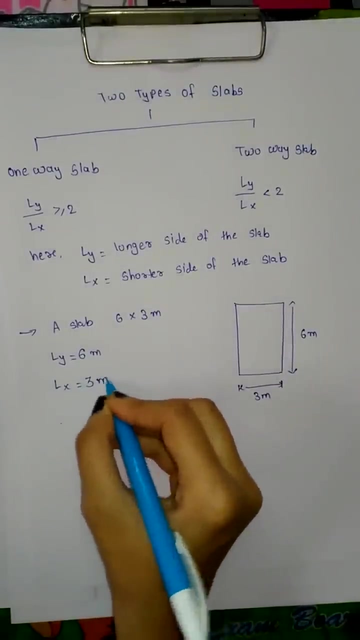 example, I have a slab having size 6 by 3 meter. Let us draw this so we have clear idea about it. This will be 3 meter and the longer side is 6 meter. So, as per the rules, we have to take Ly as a longer side- it is 6 meter- and Lx is a shorter side, so it is 3 meter. Now let's 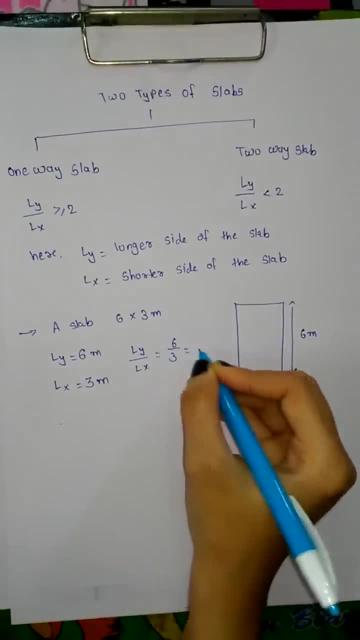 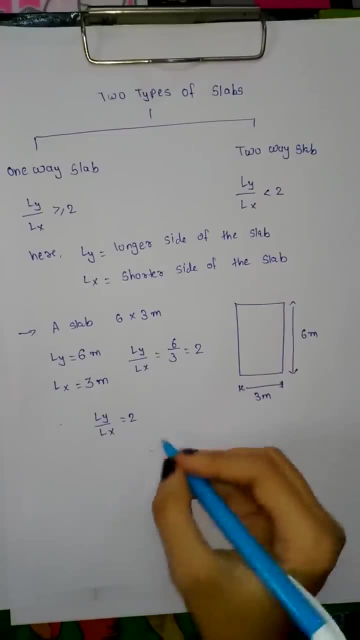 calculate Ly by Lx ratio: it is 6 by 3 and here it is 2.. So, as per our rules, Ly by Lx if it is more than equal to 2, here it is equal to 2.. So this slab will behave as one way slab. 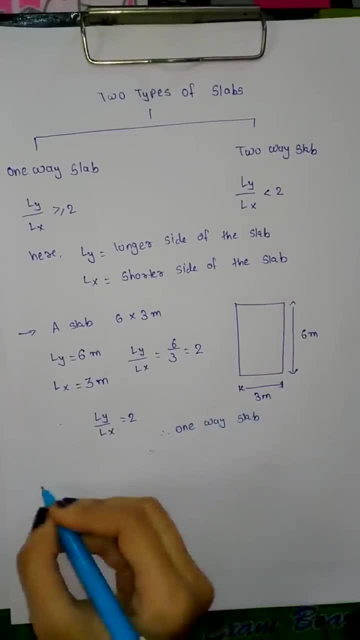 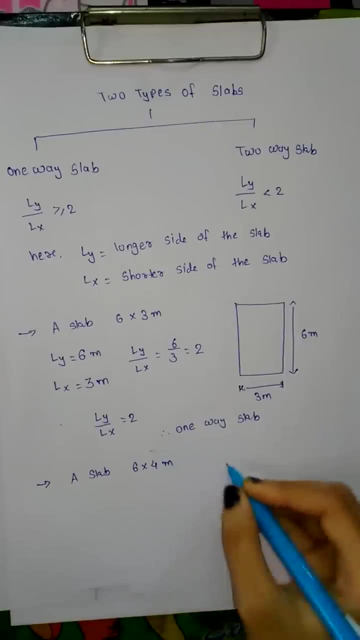 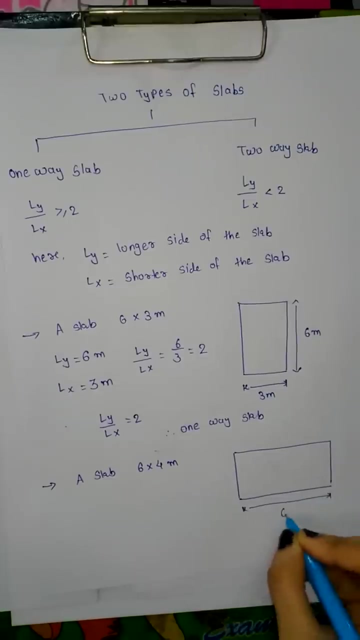 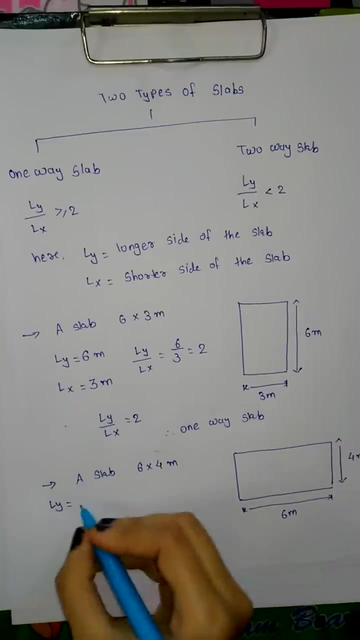 Similarly, consider a slab having a size 6 by 4 meter. Let's draw this, let's say: this is my side, 6 meter and this will be 4 meter. As per the rules, we have to consider the longer side as L, y and. 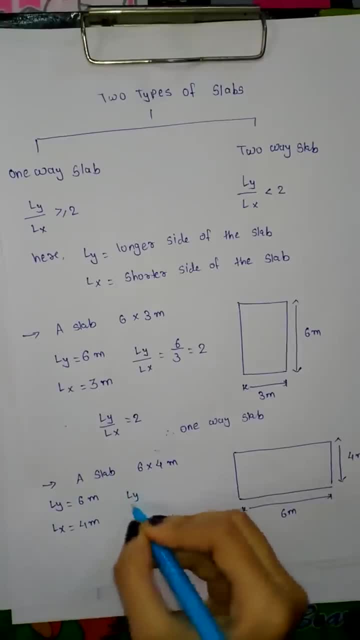 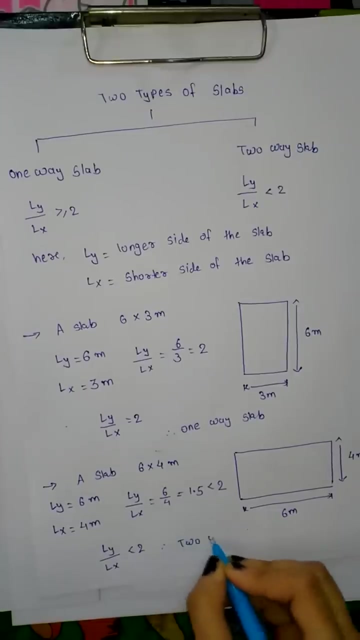 the shorter side as Lx Centre of these الأ. so let's calculate ly by LX ratio, which is 6 by 4 and it is 1.5. it is less than 2. so if our ly by LX ratio is less than 2, the slab will behave as two-way slab. 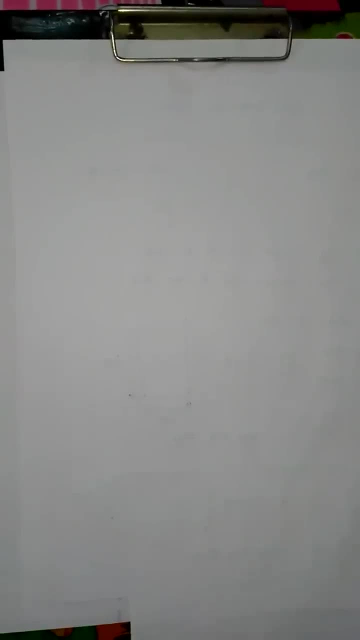 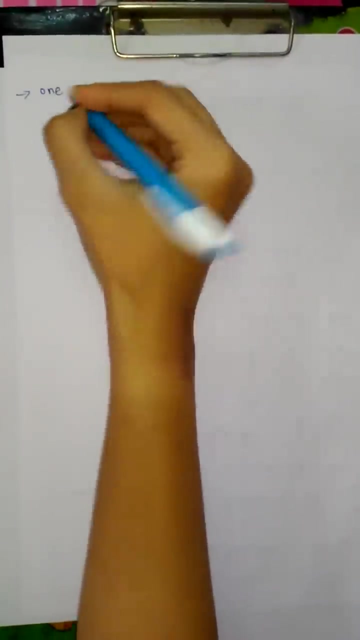 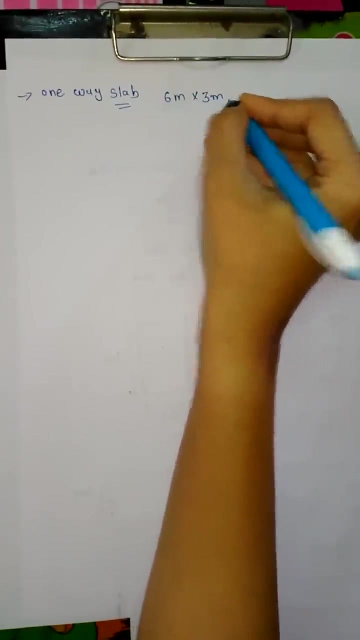 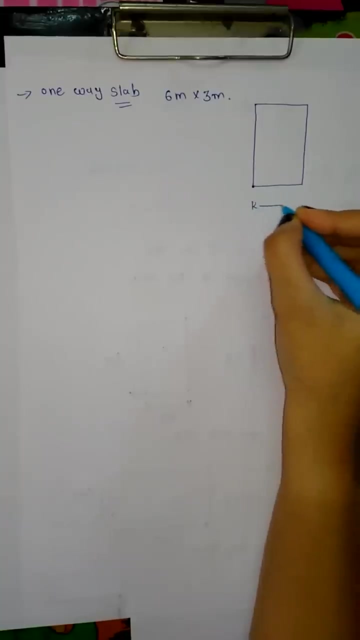 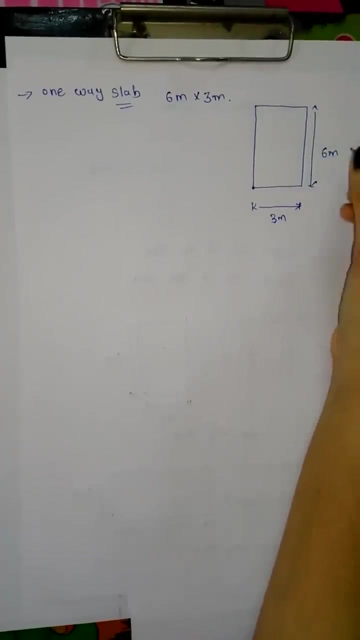 now let's get clear how the slab loads distribute to the beams. first let's understand for the one-way slab. as we have taken our one-way slab having size 6 meter by 3 meter, let's draw so the shorter side is 3 meter and our longer side is 6 meter, let's give. 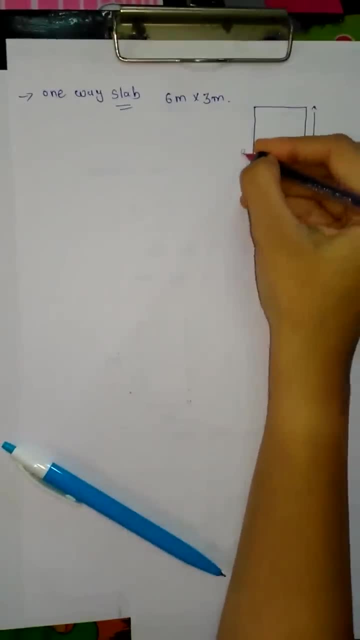 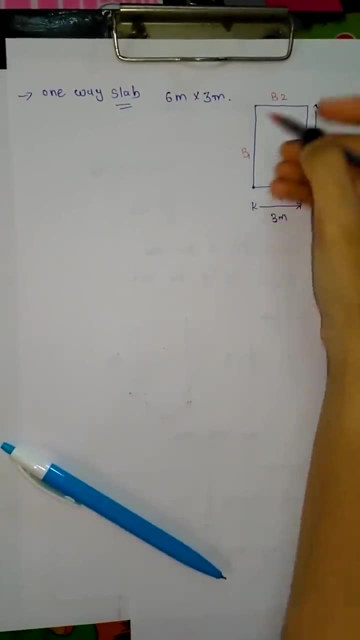 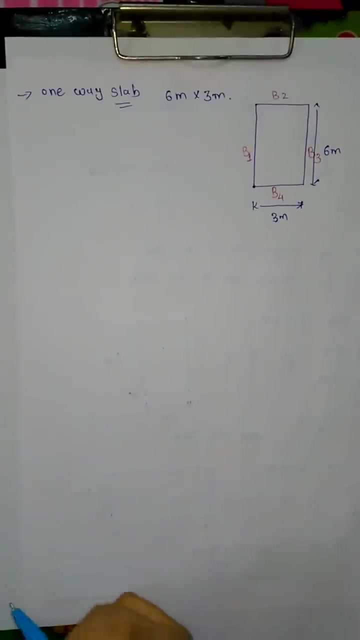 nomenclature for the beams. you can see B1, B2, B3 and B4. so this much portion will be behave as a slab. now we have to understand how this slab load, or we can say how this slab load will behave as a slab. now we have to understand how this slab load, or we can say how this slab load. or we can say: 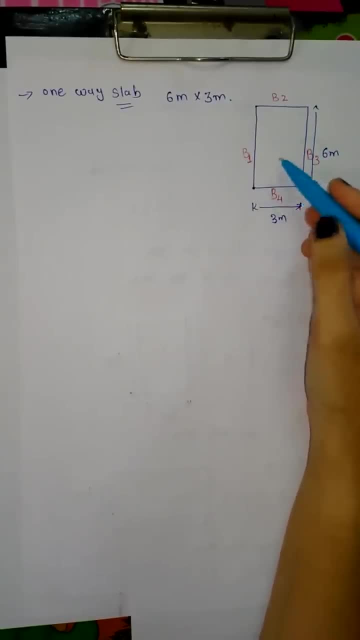 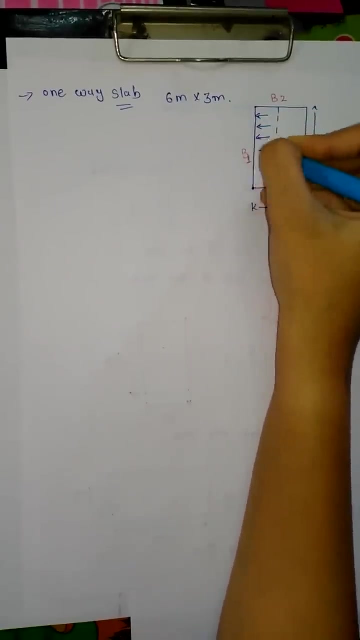 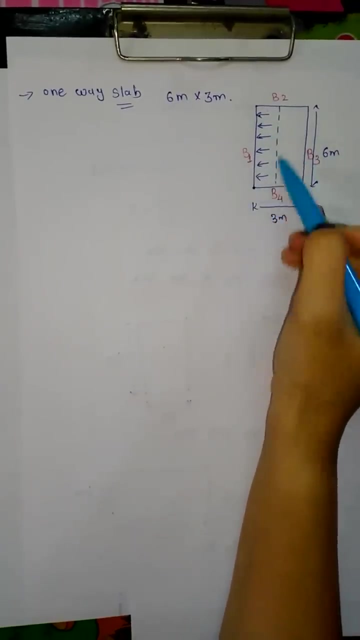 the self weight of this particular slab transfer to the each and every beam. so for the one-way slab, half of the slab load will be transferred to the either side of the beams. so you can see whatever I have draw for the arrows. so half of the rectangular portion of the slab load is transferred to the slab. 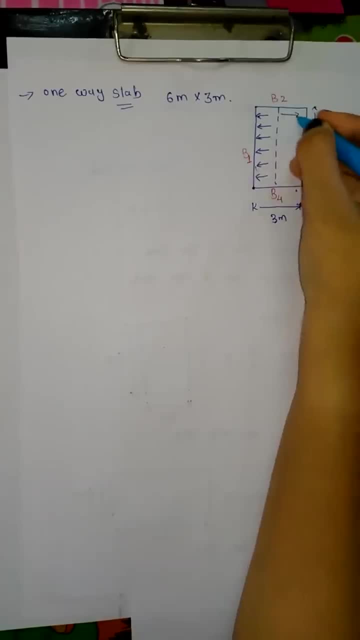 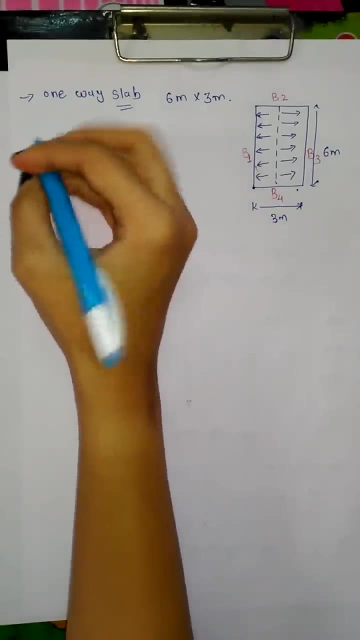 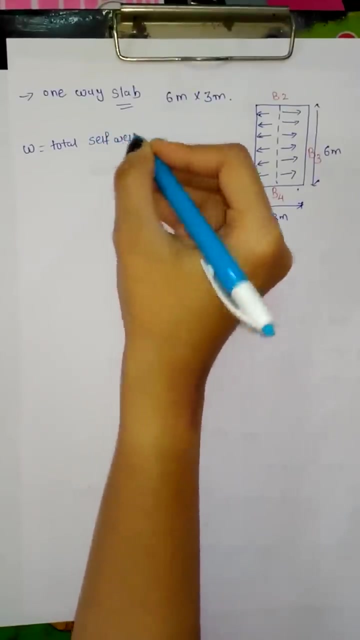 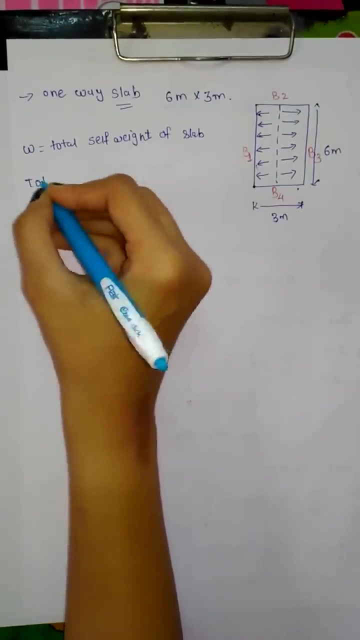 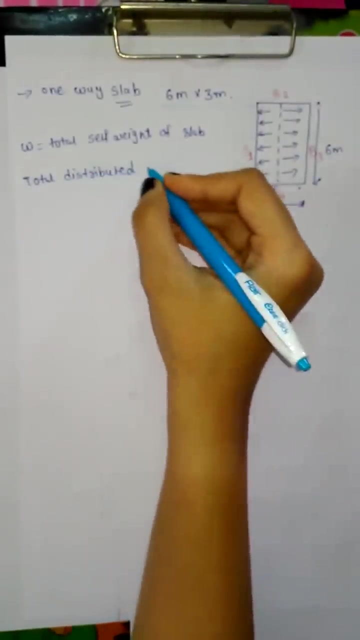 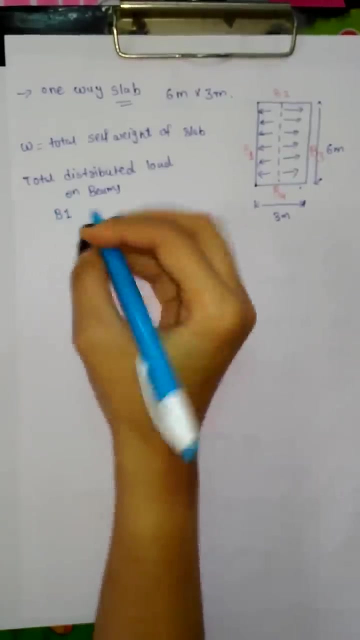 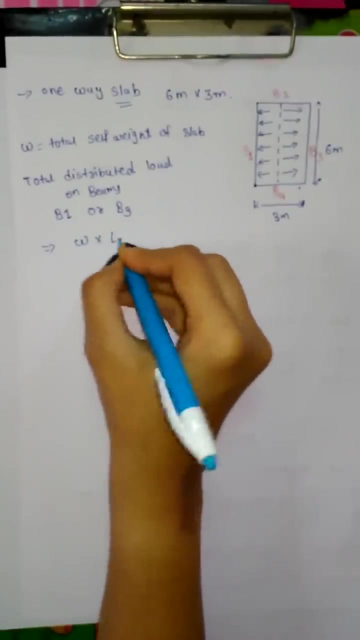 beam B1 and half of the slab load is transferred to the beam B3. now if we take W is total self-weight of the slab. so whatever total distributed load on beams and the beams, they are B1 or you can say B3. so if the total formula will be W multiplied by L of X, which is a shorter, 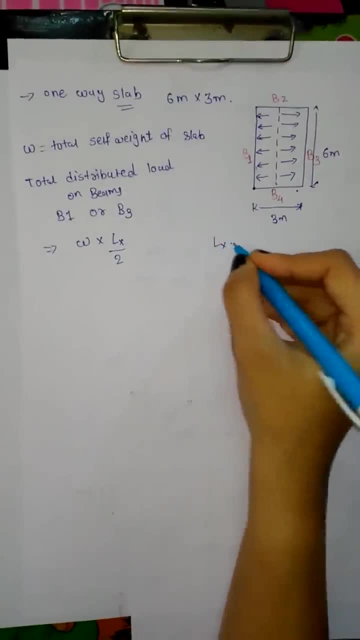 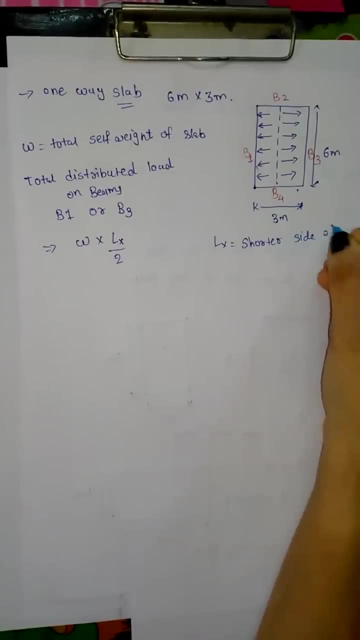 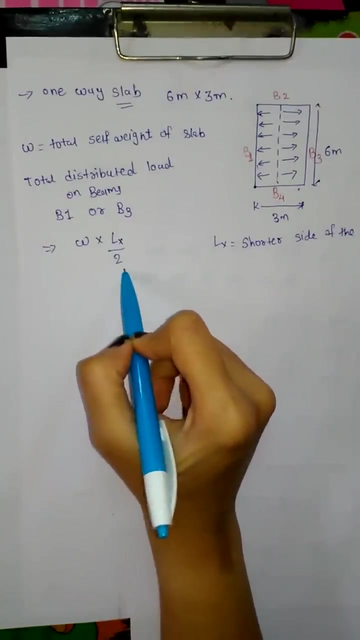 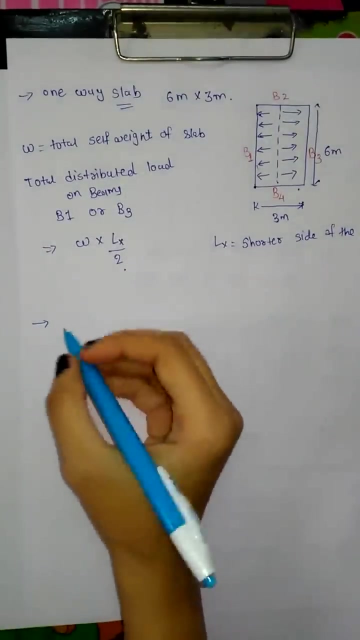 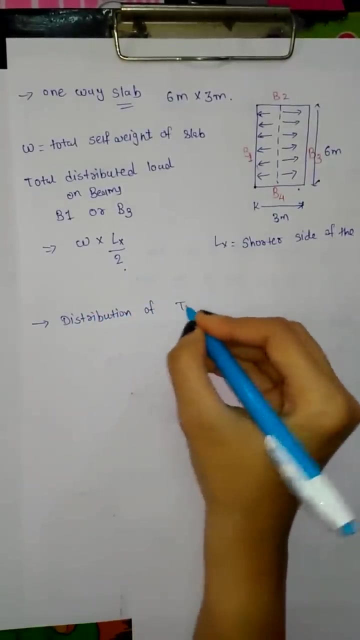 dimension of the slab. so let's write here: LX is a shorter side of the slab, so this is a formula for the total distribution of the slab loads on the beams. similarly, let's understand for the distribution of two-way slab, distribution of two-way slab as we have. 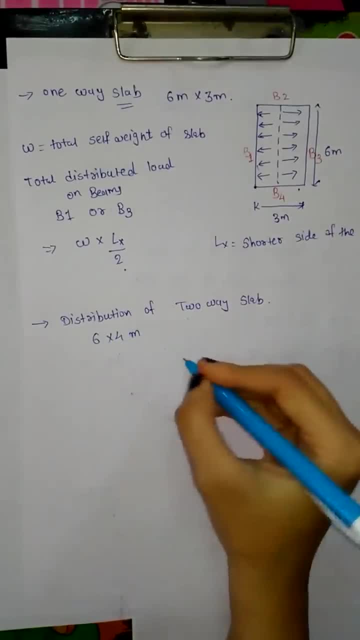 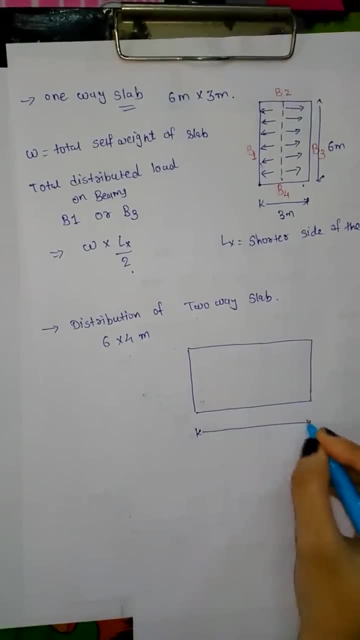 taken two-way slab, 6 by 4 meter, so let's draw it. the longer side will be 6 meter and the shorter side will be 4 meter. ok, now for 2x slab. it will be distributed itself weight in two shapes and they are trapezoidal shape and. 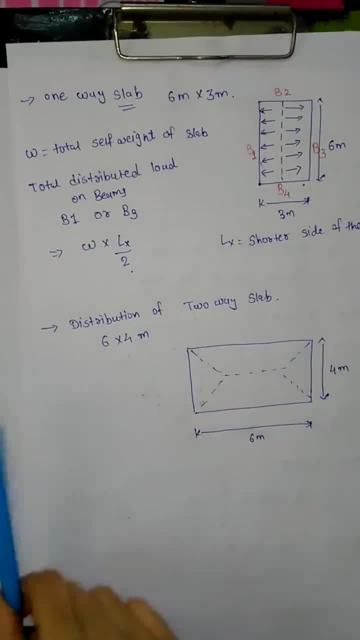 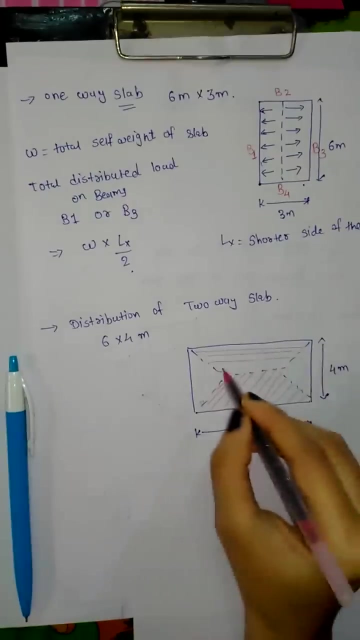 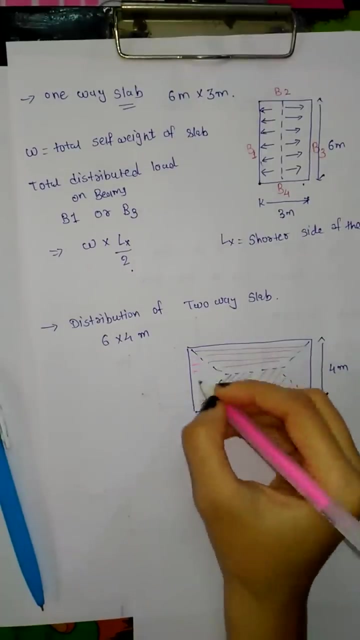 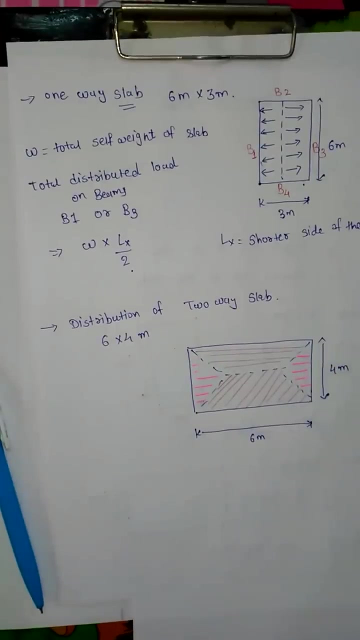 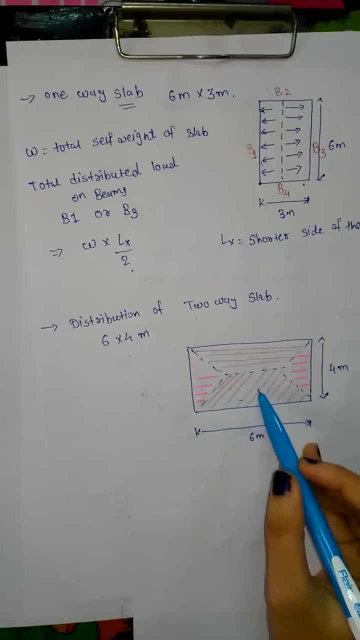 triangular shape. so you can see here these portion of the slab will behave as a trapezoidal shape and you can see this is the other slab side of the trapezoidal shape and the remaining portion is act as a triangular shape and these portion, these trapezoidal portion of the slab load, will act on this beam. let's understand. 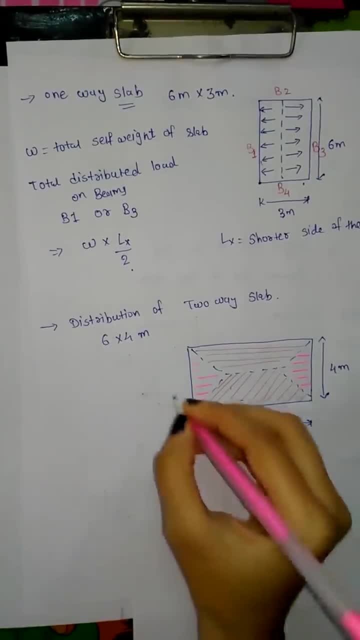 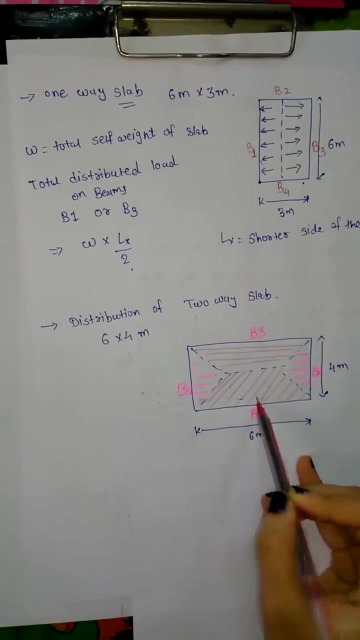 first give the nomenclature for the beams B1, B2, B3 and B4 so we can easily understand this. ok, so this much portion, so we can say trapezoidal portion- of the slab load will transfer to the load. sorry, beam B1 and this much the another trapezoidal load will transfer. 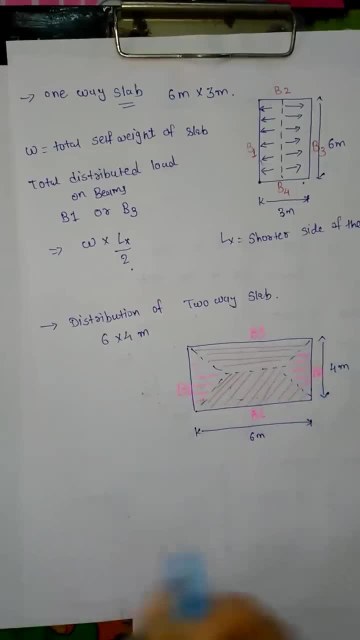 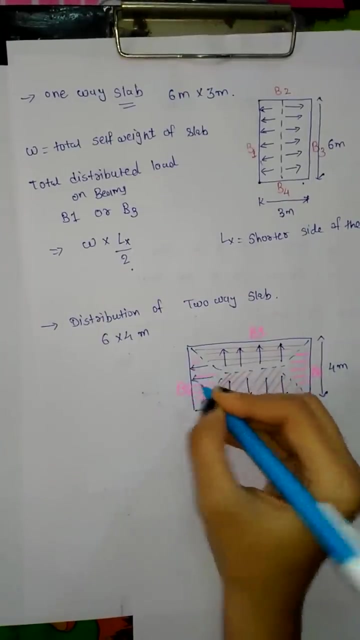 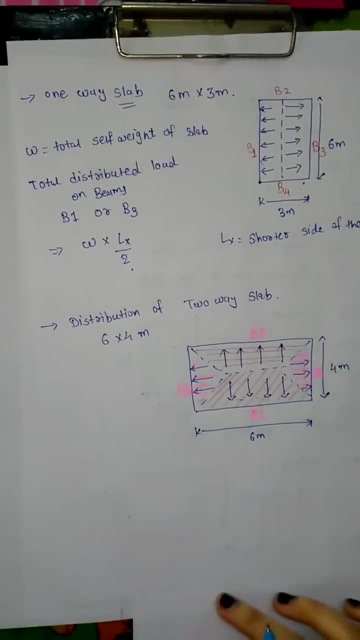 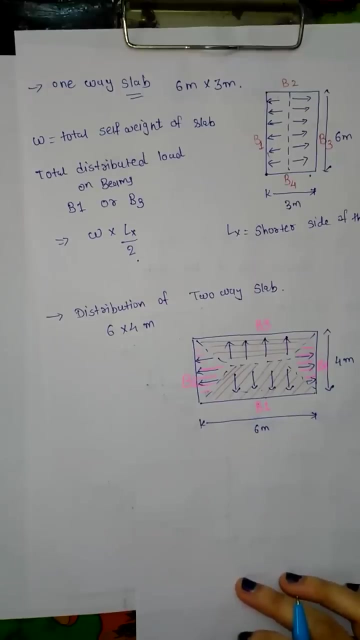 to the beam B3. You can say the direction of the slab loads. ok, like this. similarly, triangular portion of the slab load will distribute on beam B2 and same as for the beam B4. so we have to determine a formula for triangular shape of the slab load and for the trapezoidal shape of the slab load. 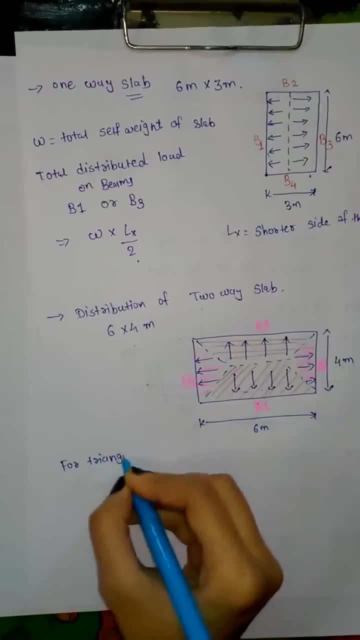 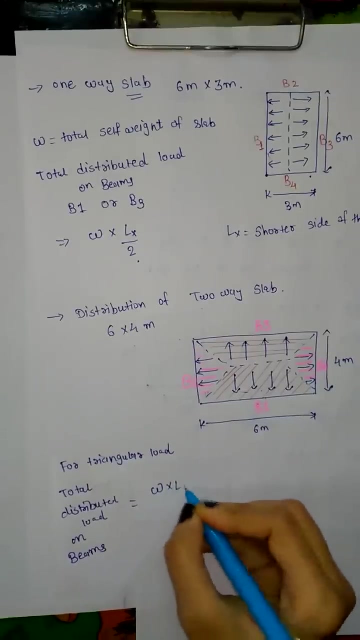 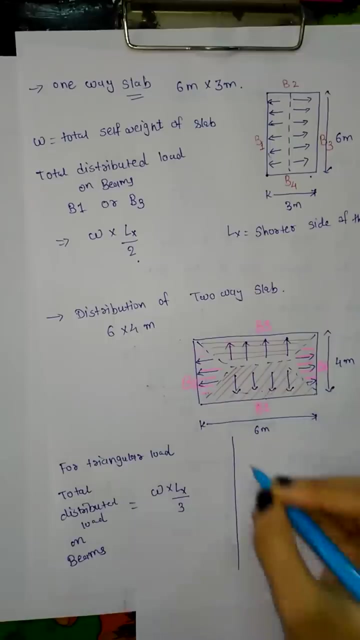 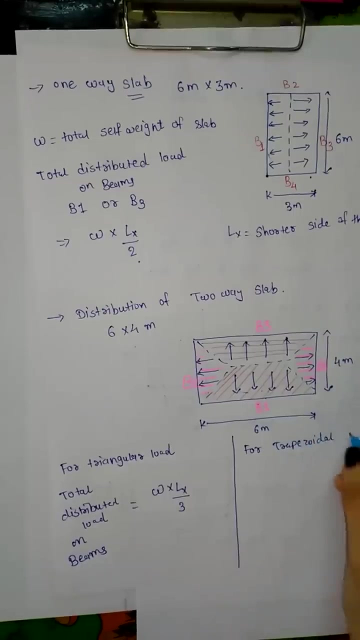 For triangular load, the formula is something like this: total distributed load on beams is equal to W, which is a self weight of the beam multiply by L of x divided by 3, and we know that Lx is a shorter dimension of the slab. Similarly, let's understand for trapezoidal load, and the total distributed load is W multiply. 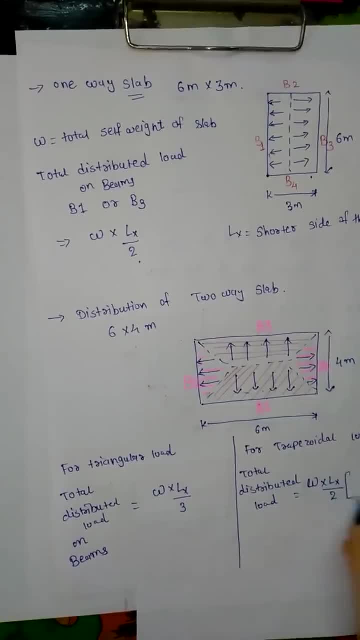 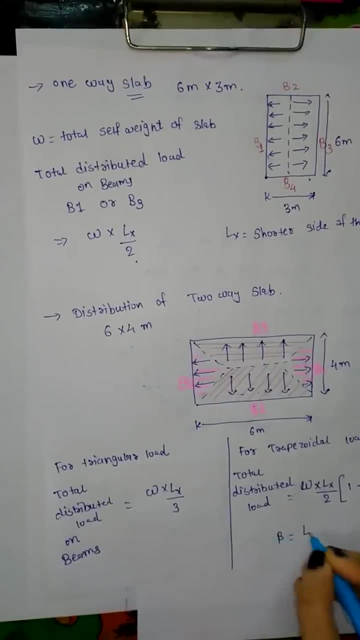 by L of x divided by 2.. 1 minus 1 of 2 beta. Now what is beta? 1 minus 1 of 2 beta, Beta is nothing but the ratio of Ly by Lx. So how this we understand how the slab loads one way and two way will distribute on the. 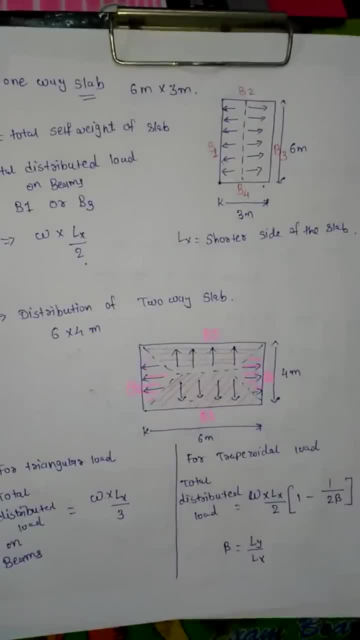 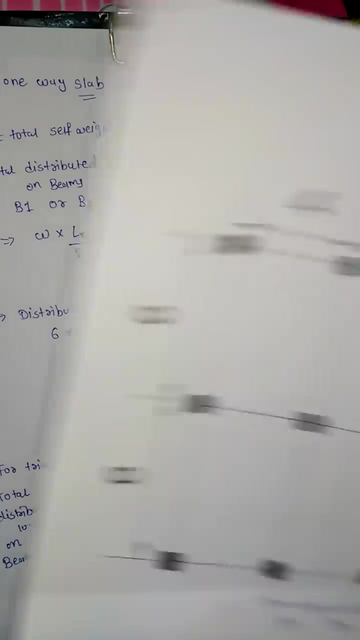 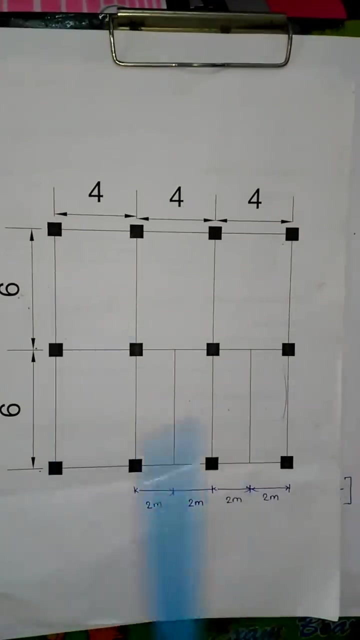 beams. So I think this distribution of the slab loads on the beam will be more clear with a simple example. Let's take a simple example For the plan of a building. here I am taking a plan of a building having beams and columns with a slab. 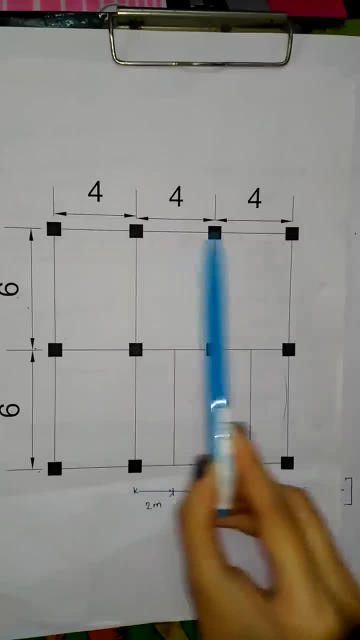 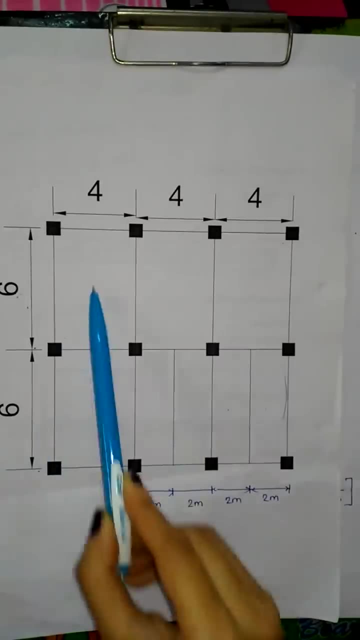 You can see, here we have longitudinal beams having length 4 meter and the lateral beams having length 6 meter. These 1, 2,, 3,, 4, 5, 6, 7, 8. We have total 8 number of slabs here. 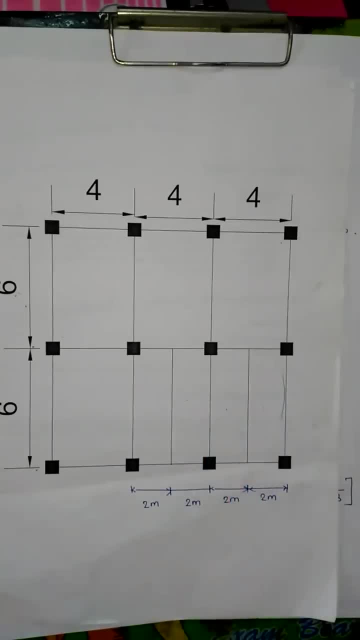 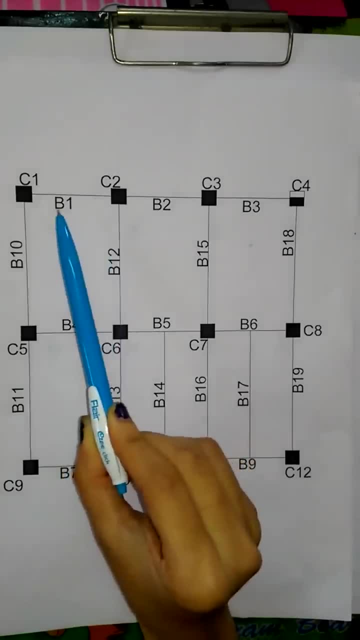 You can see the nomenclature for the beams will start with B1, B2,, B3,, B4,, B5,, B6,, B7,, B8, B9, B10 is here, B11,, B12,, B13,, B14,, B16,, B17,, B18,, B19,, B20,, B21,, B22,, B23,, B24,. 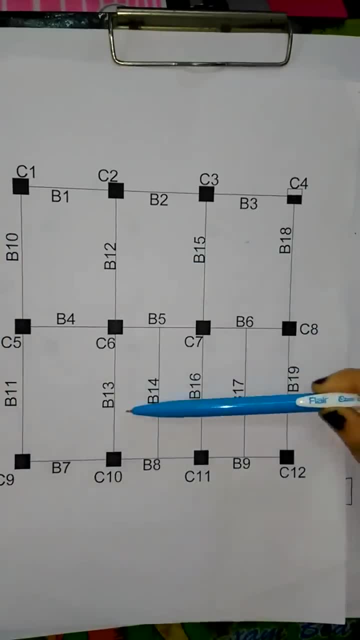 B25,, B26,, B27,, B28,, B29,, B30,, B31,, B32,, B34,, B35,, B36,, B37,, B40,, B41,, B42,, B43,, B44,, B45,, B46,, B47,, B48,, B49,, B50,, B51,, B50,, B52,, B52,, B53,, B54,, B46,, B49,, B50,, B50,, B51,, B52,, B50,, B50,, B52,, B50,, B53,, B14,, B14,, B16,, B17,, B18,, B19,, B19. 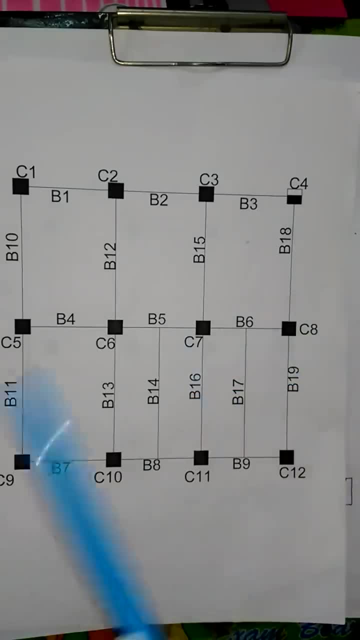 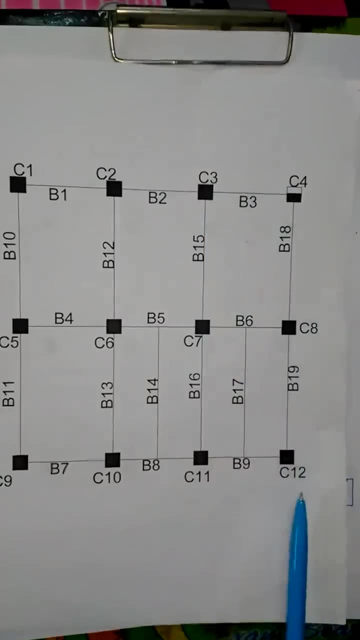 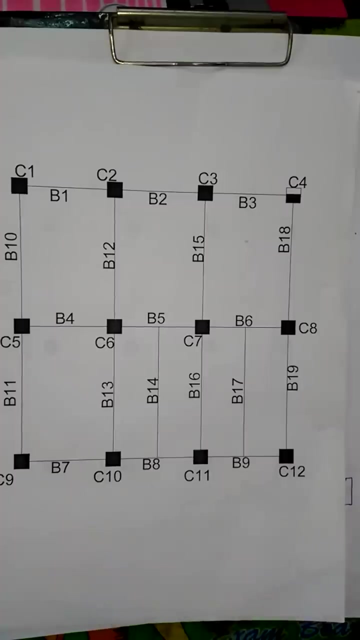 So we have total 19 beams here and similarly we have given nomenclature for the columns. You can see C1, C2, C3 upto C12.. So total 12 columns are here. First we have to understand primary beams and secondary beams. 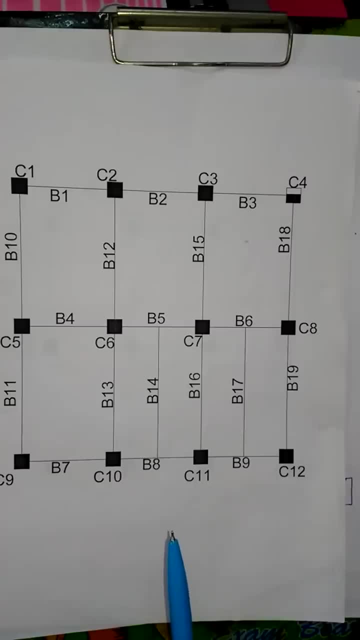 So we already know that when the beam are supported with columns from the both side, they are considered as a primary beams And the secondary beams are considered when these beams are supported either on walls or another beams. Basically, they are not supported with columns from both side. 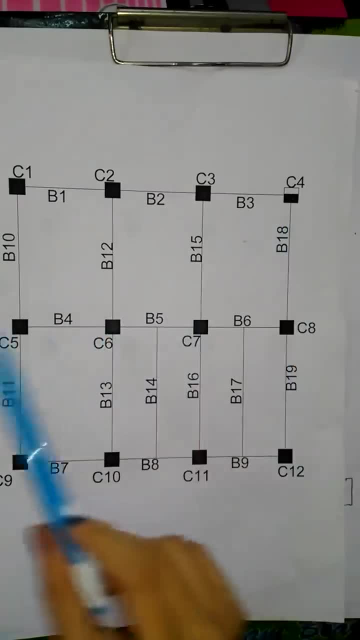 Ok, so you can see here this: B1, B2, B3, B4, B5, B6, B11, B12, B13,, B14, B15,, B16,, B17,, B18, B19, B20, B22, B23, B24, B25, B26 are the primary beams. 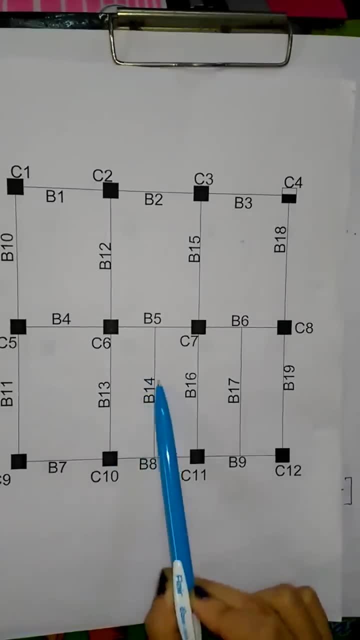 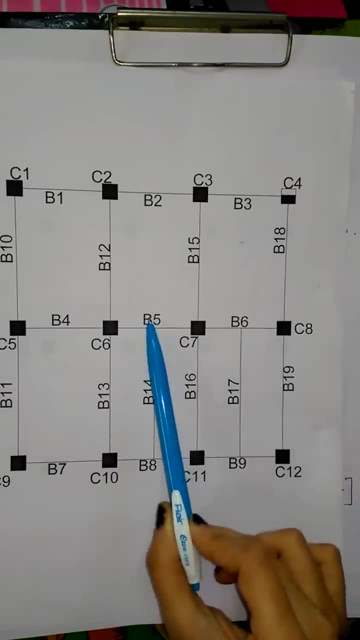 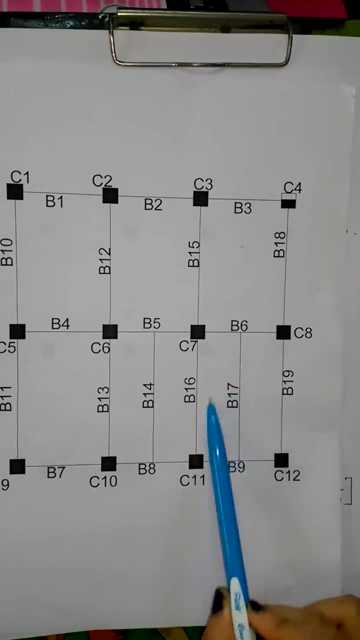 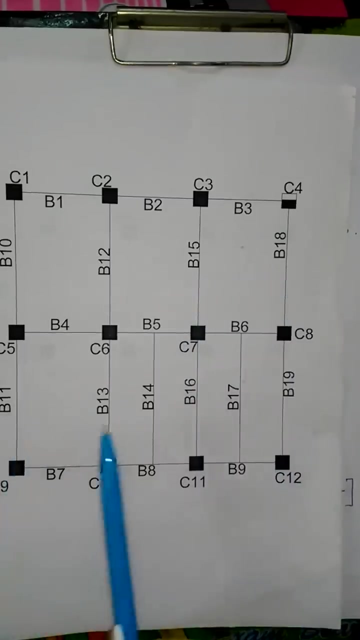 The only secondary beams are here. You can see B14.. B14 is supported from the both side, is B5 and B8.. The another secondary beam is B17.. B17 is also supported with B6 and B9.. Ok, And the other secondary beams are B10, B12, B15, B18, B11, B13, B16, B19. 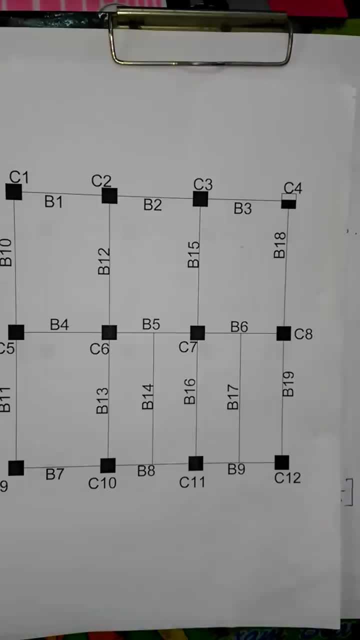 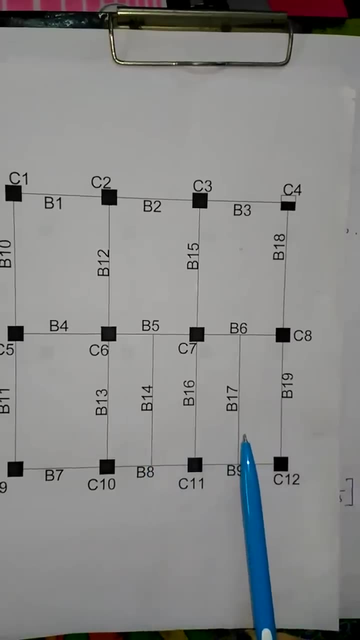 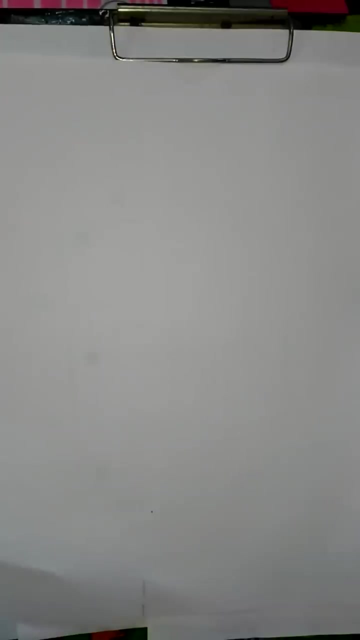 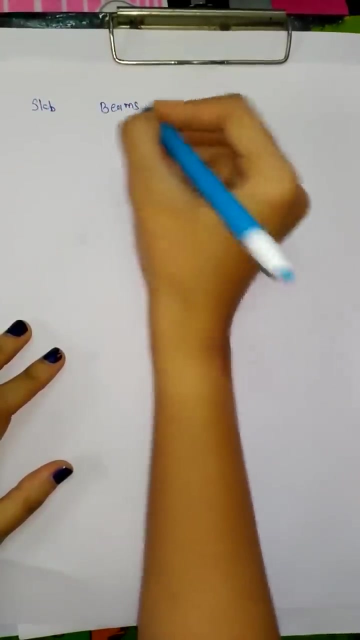 These all other beams are considered as primary beams. The only secondary beams are B14 and B17.. Let us calculate the self-fit of each and every structural elements. We know that here we have three different structural elements, And they are slab Beams and columns. 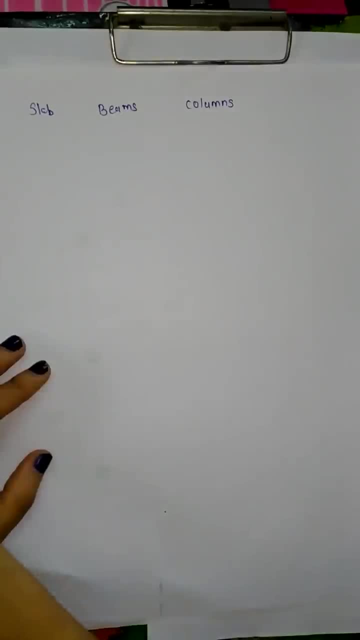 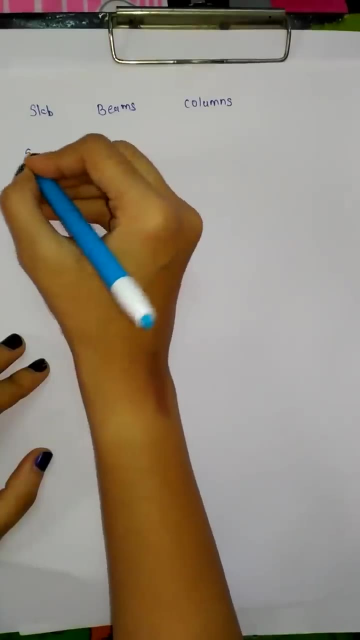 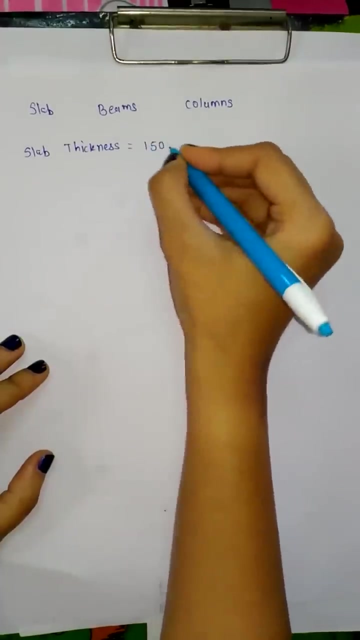 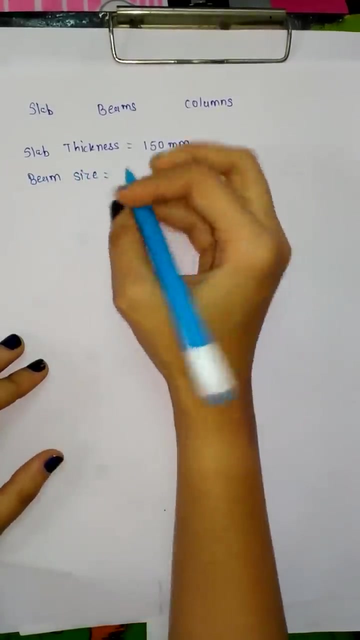 So to calculate the self-fit of these structural elements, first of all we have to assume the elements. Ok, So let us assume the slab thickness is 150 mm. Then let us consider beam size. Width and depth Is 230 mm by 600 mm. 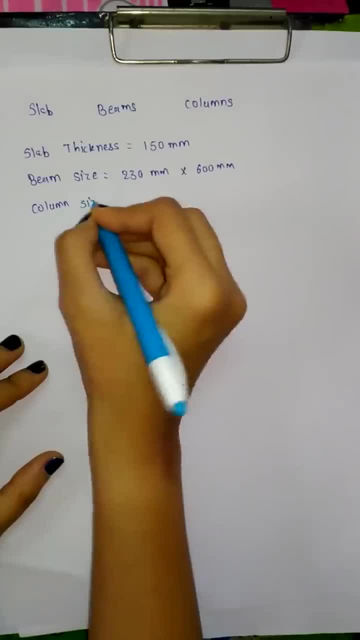 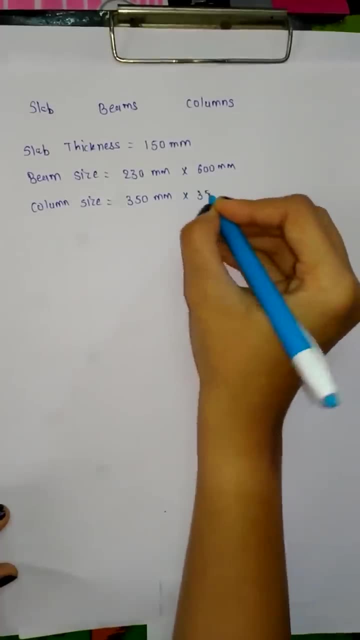 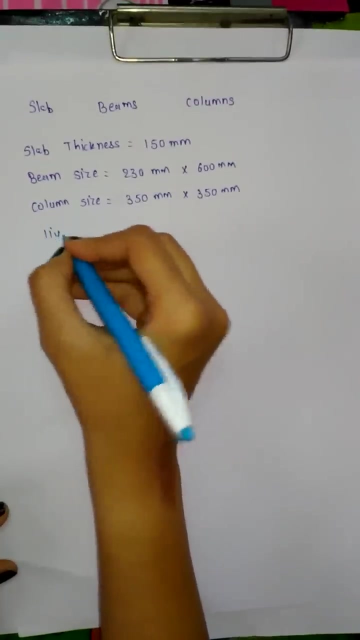 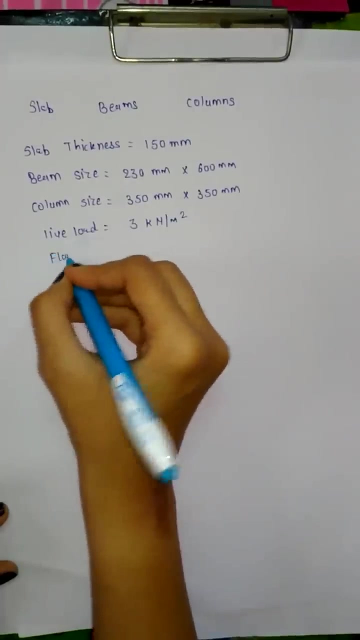 Similarly for the column. size, width and depth is 350 mm by 350 mm. You can see here I am considering a square column. We have considered live load is 3 kN per meter Square and floor finish is 1 kilo Newton per meter square. so let's calculate the 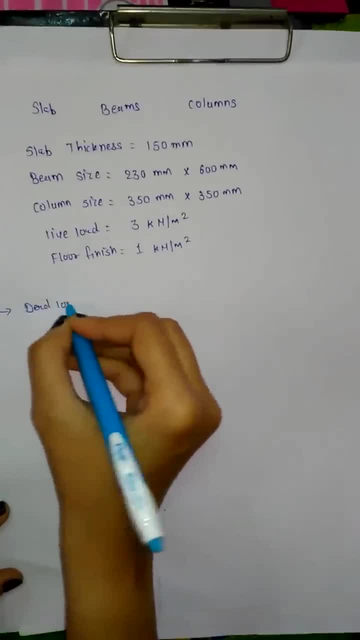 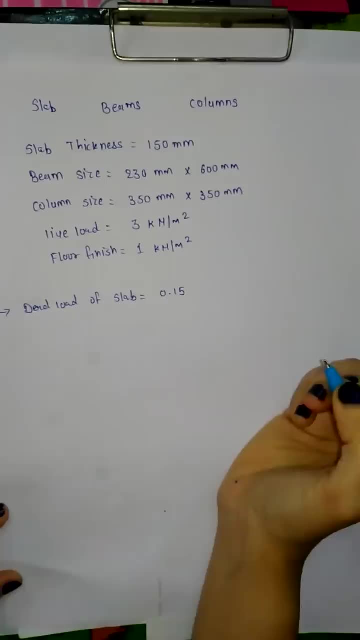 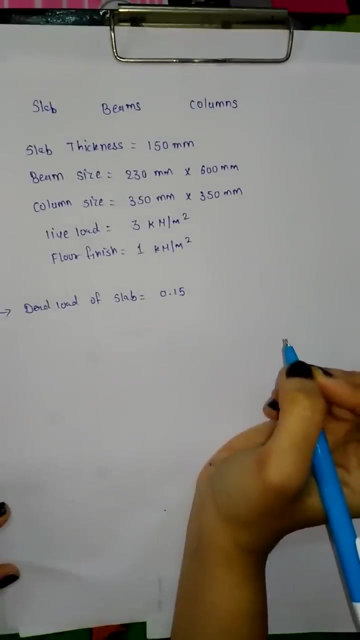 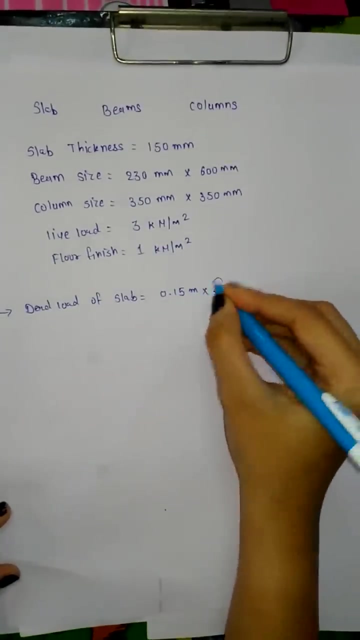 dead load of slab is so the thickness is 150 mm, and so the dead load for the slab is 0.50 meter. I'm just converting 150 to 1.50 meter. multiplied by 25, this 25 is nothing but the density of RCC. 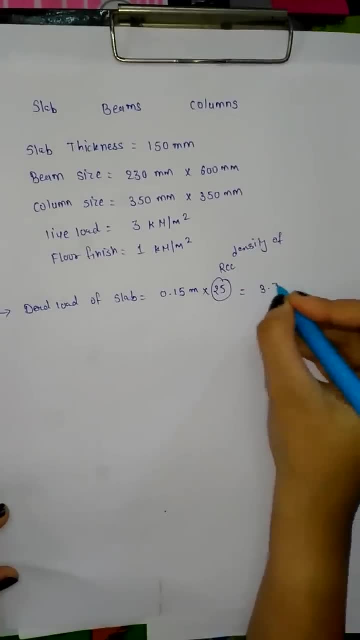 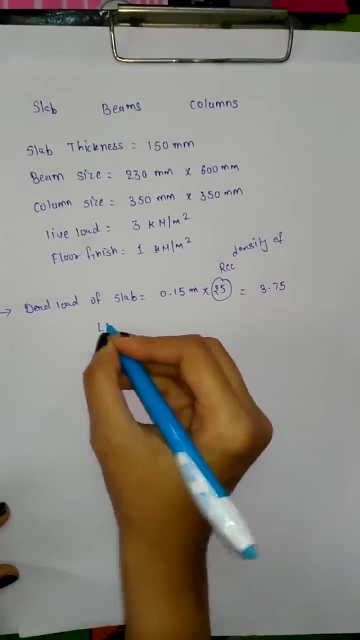 the value will be three point 75. now in dead load we have to add live load. we have already considered live load is three kilo Newton per meter square. Future value of The O'Hara будущa Frank materials saved in India. Here it is also forgot. 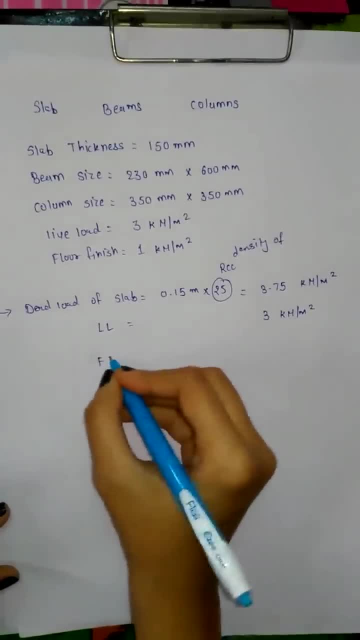 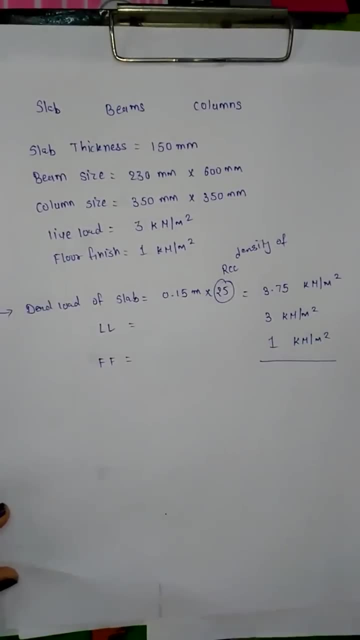 Kilo newton per meter square, And we also have to add floor finish, which is 1 kilo newton per meter square. Let's add all these three values And which is something 7.75 kilo newton per meter square. 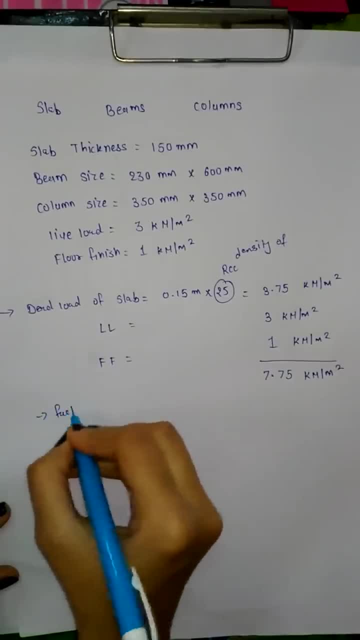 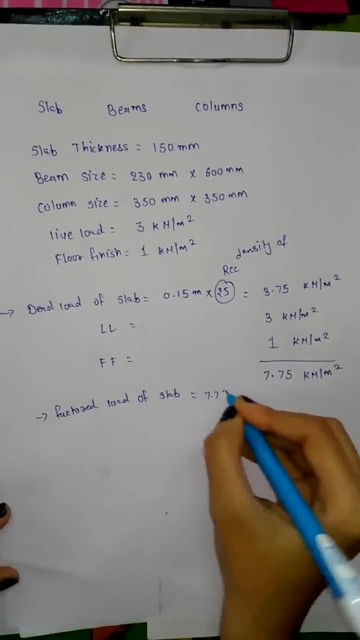 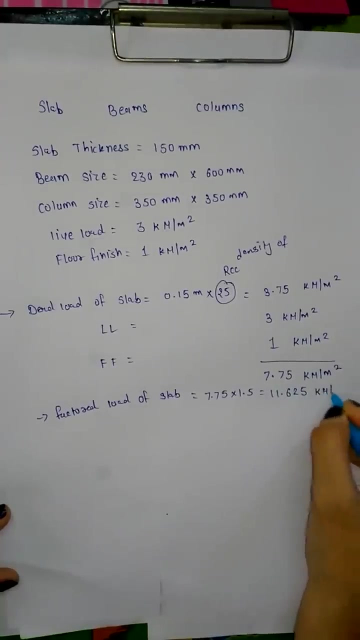 Now we also have to calculate factor load. Factor load of slab 7.75 multiplied by 1.5.. And the value will be approximate 11.625 kilo newton per meter square. Similarly, we have to calculate self weight of the beams. 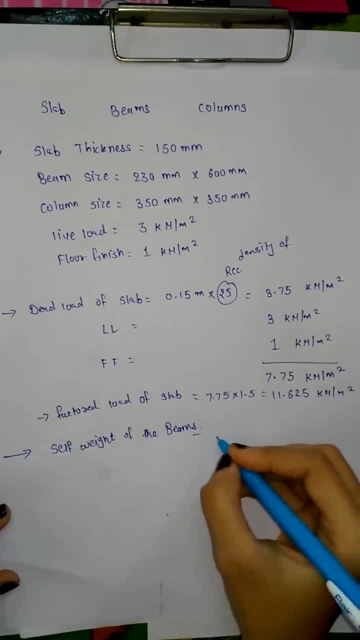 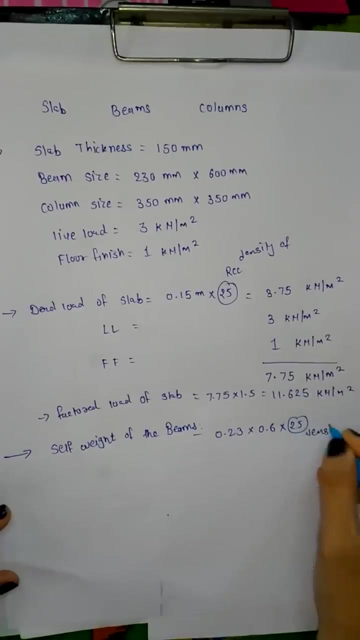 As the size of beam is 230 mm by 600 mm, So let's convert it into meter 0.23 by 0.6, sorry, And we have to multiply it With density of RCC, And so the value is something. 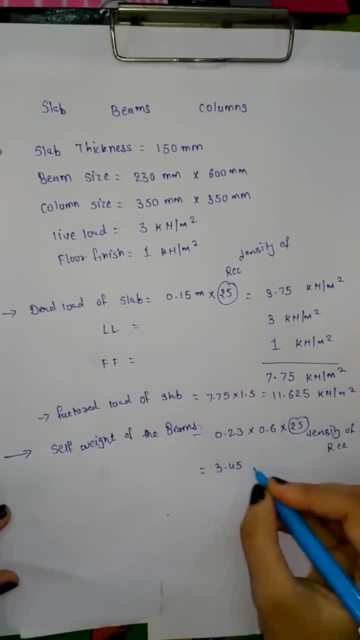 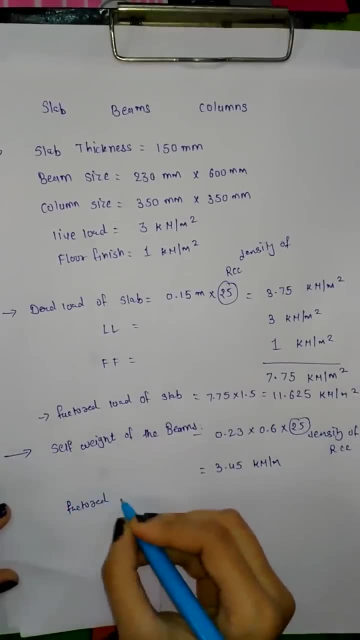 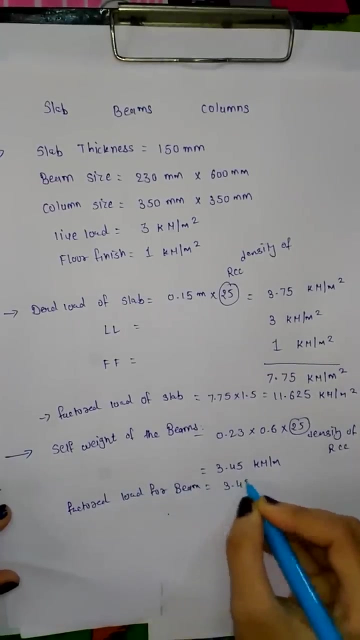 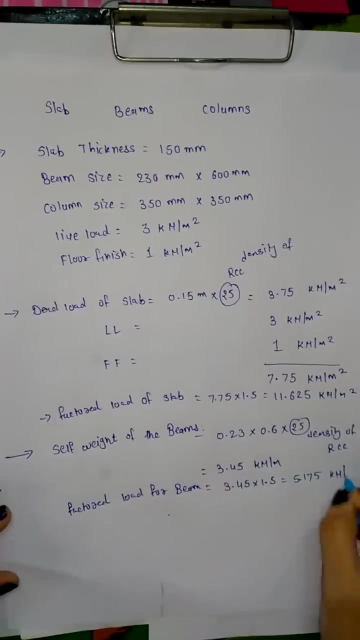 Okay, 3.45 kilo newton per meter. Again, we have to do factor this load. Factored Load for beam is 3.45 into 1.5. It is 5.175.. Kilo newton per meter. 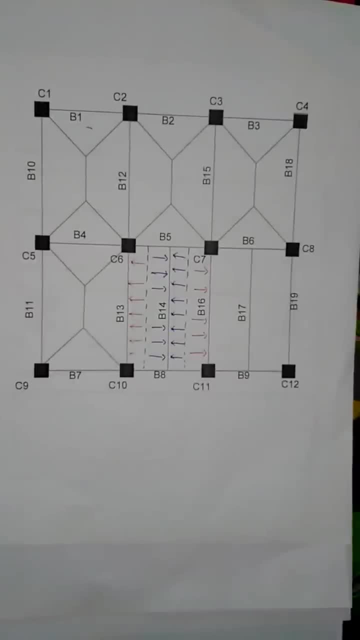 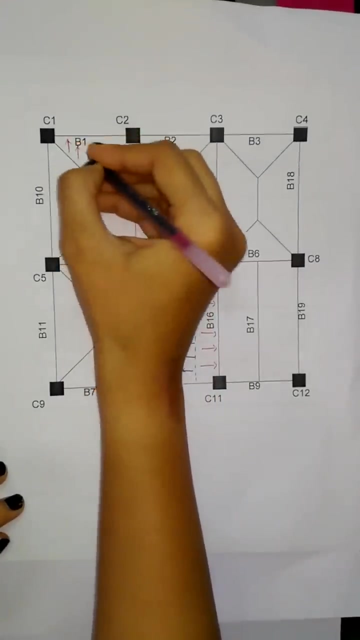 Okay, now let's go one by one with beams And calculate how much load is transferred from the slab. So let's take beam number 1.. You can see, beam number 1 is subjected with 1 triangular load plus its own self weight. 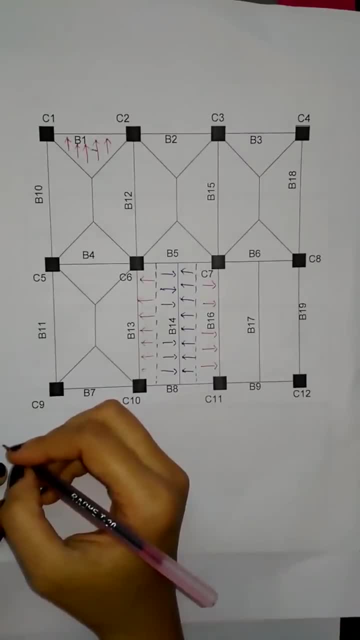 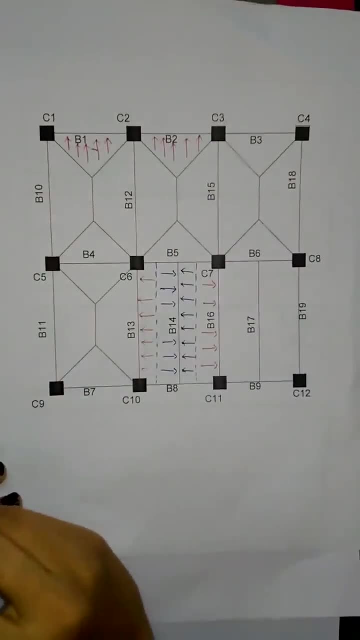 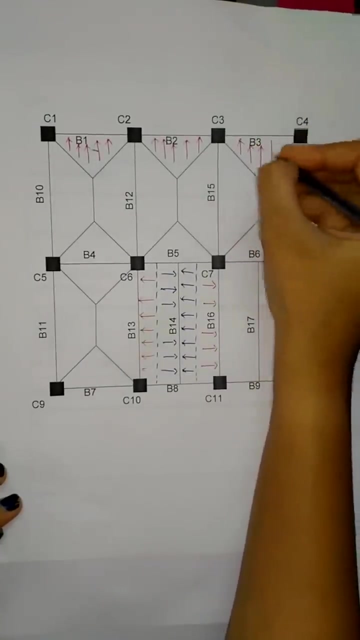 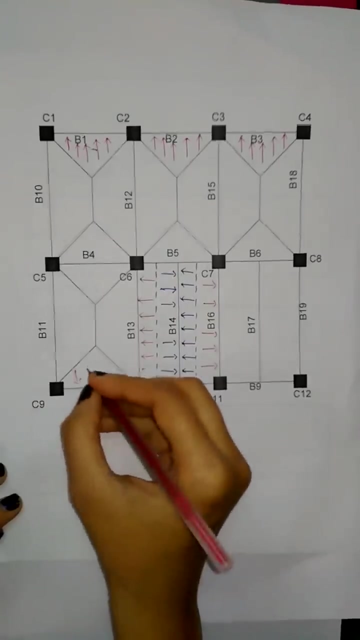 Similarly B2.. Beam B2: you can see it also Subjected with 1 triangular load and its self weight. Similarly, you can take as B3. It also subjected with 1 triangular load plus its own self weight, And same for the B7.. 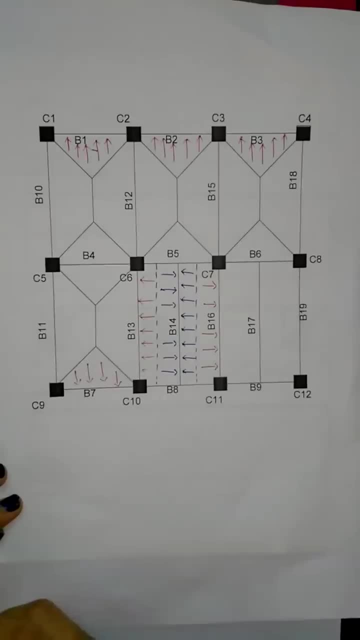 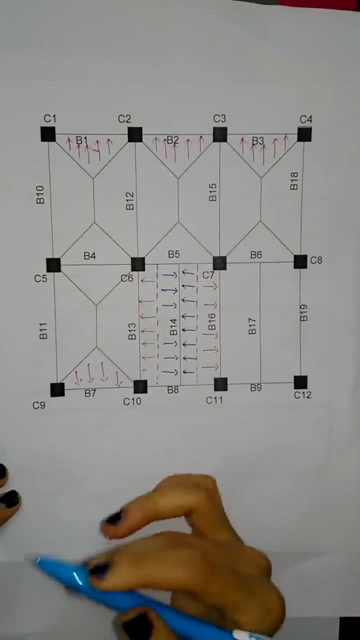 It also subjected with 1 triangular slab load plus its own self weight. So I think Okay. So I think these all- B1, B2, B3 and B7- will be subjected with similar kind of loads. So we have to consider different groups of the beams. 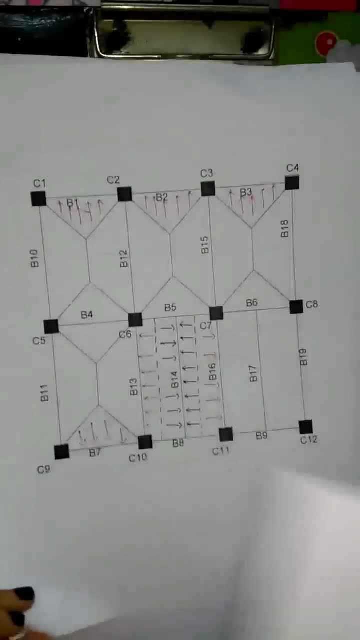 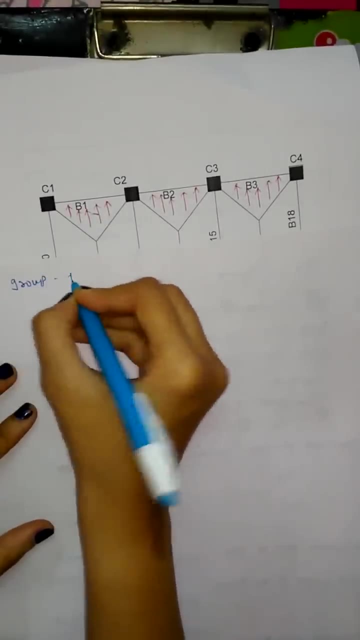 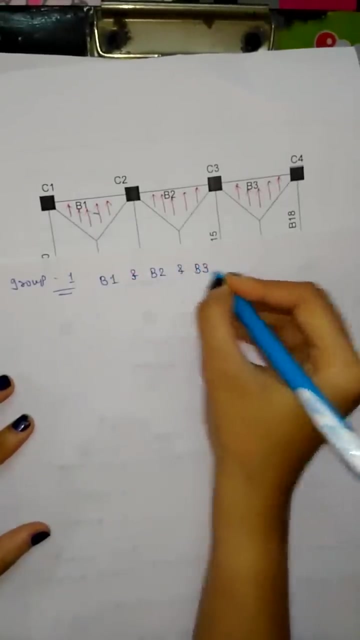 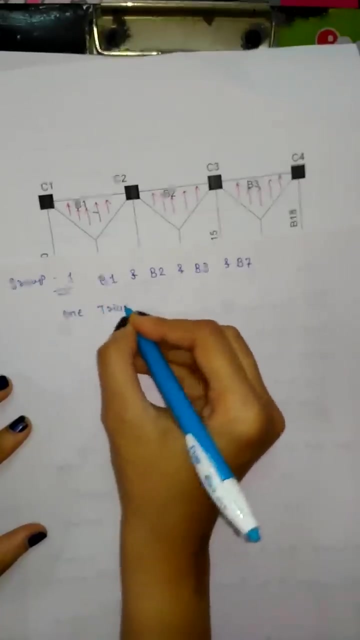 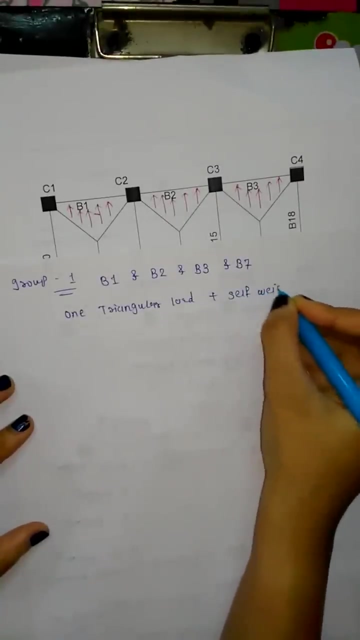 Let's calculate for this group of the beam. Let I am taking group number 1. And that is B1 and B2 and B3.. B3 and it is B7. Which is subjected with 1 triangular load plus self weight of beam. 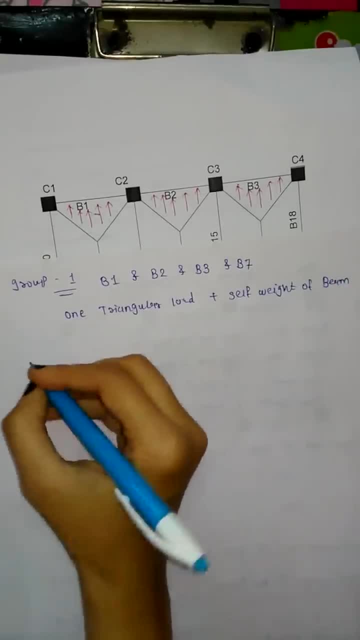 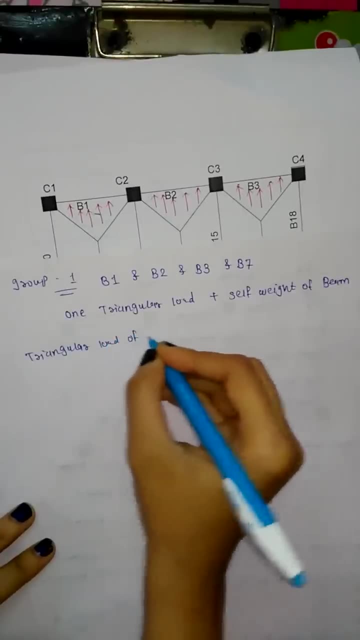 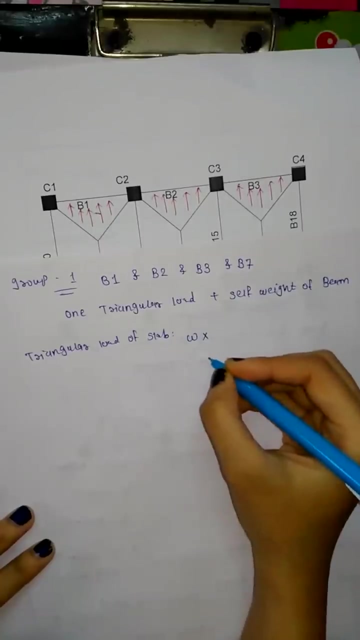 First of all, we have to calculate triangular load of the slab, As we have already discussed. What is the formula for triangular load? It is W, L of x by 3. Where L of x is a shorter dimension of the slab. So here, what is W? 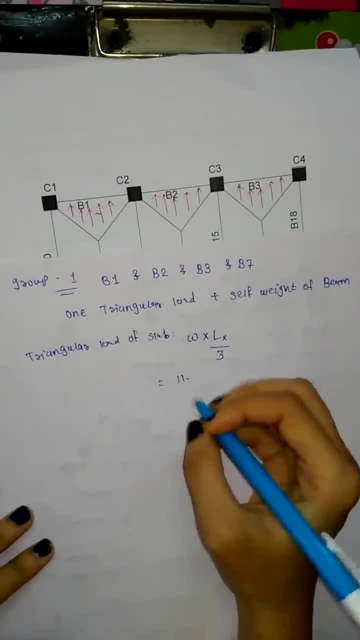 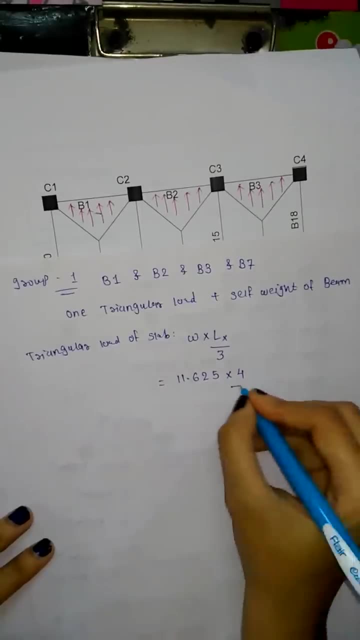 W is our total factor, self weight of the slab. So it is 11.625, which is already we have calculated. multiplied by 4 is a. Lx Is a shorter dimension of C. You can see this panel is a shorter dimension of C. 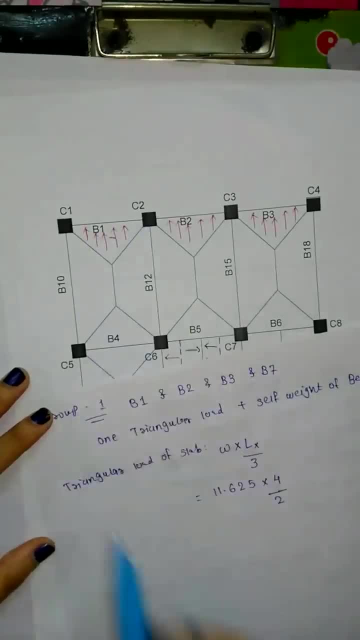 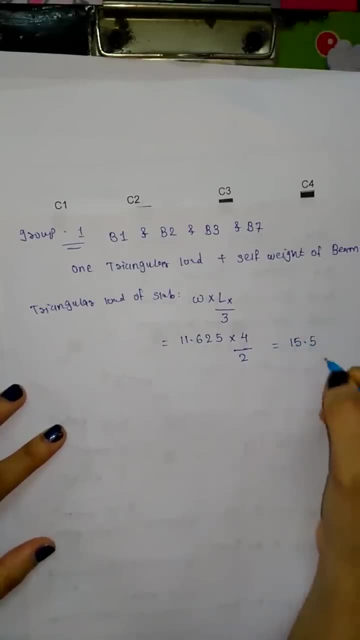 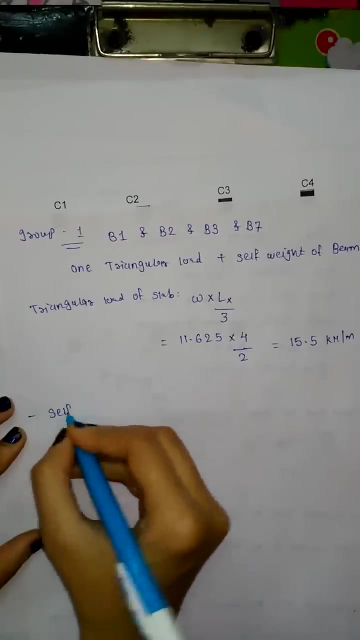 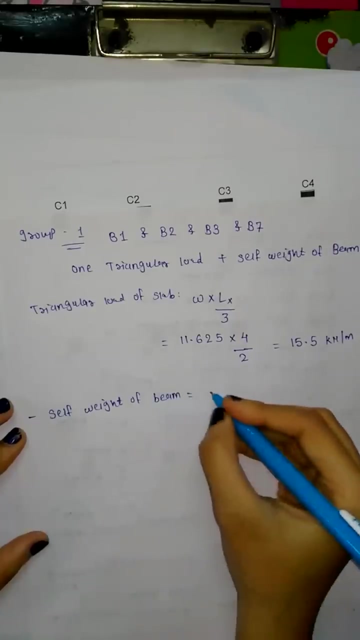 So it is a shorter dimension of this slab panel: 4 m x 2.. So the value will be, I think, approximate 15.5 kN per m And the self weight of the beam Factor. self weight of the beam is- We have already calculated- 5.175 kN. 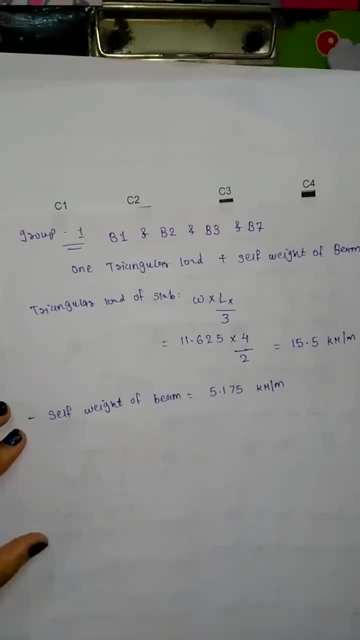 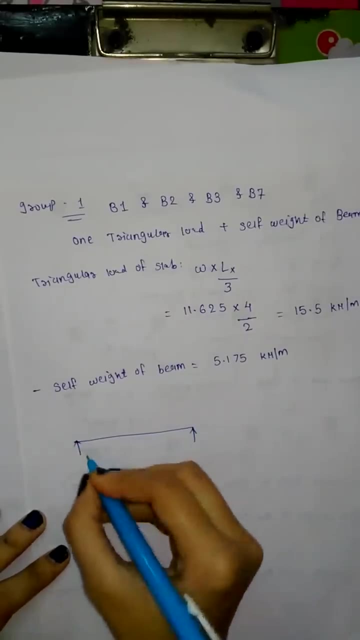 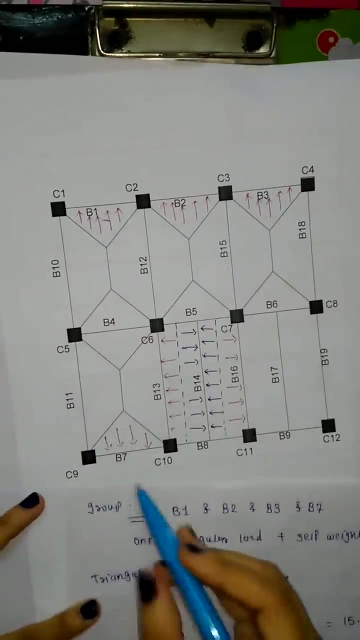 Per m. Okay, Now let's draw this. If we have 4 m of beam, As we know that this B1, B2, B3 and B7.. The length of the beam is 4 m And it is subjected with UDL. 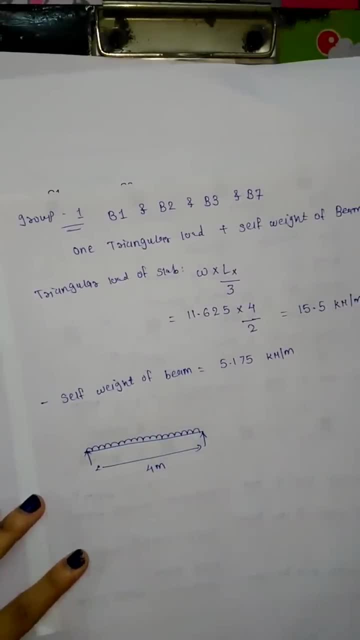 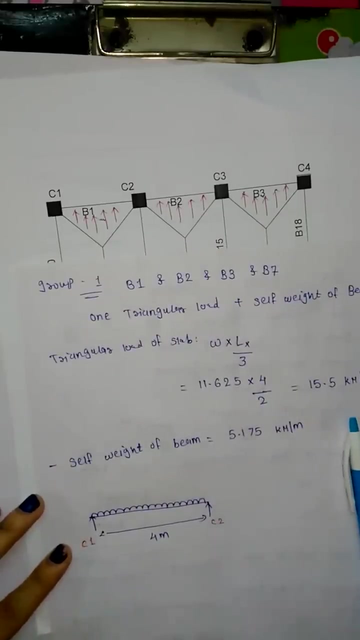 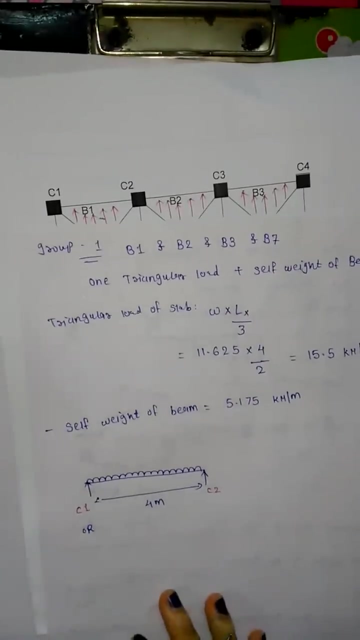 It is subjected with UDL Support will be Column number C1.. Column number C2.. If it is B1.. Now if we are taking B2.. The support will be right side. Sorry, left side is C2 and right side is C3.. 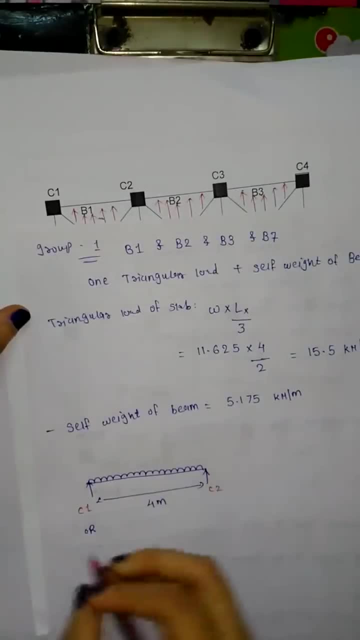 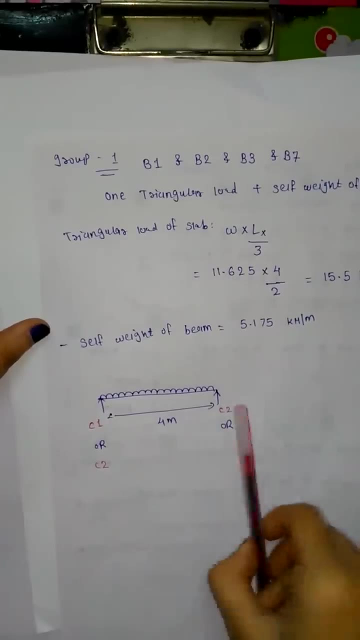 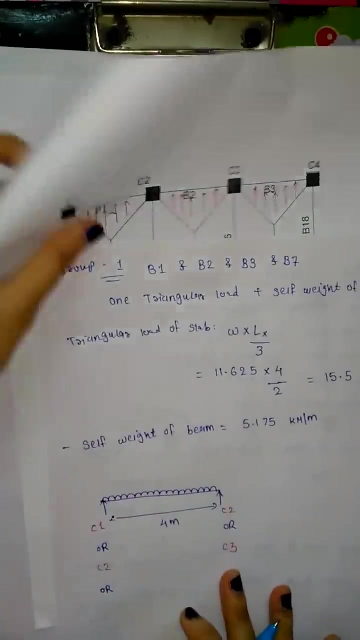 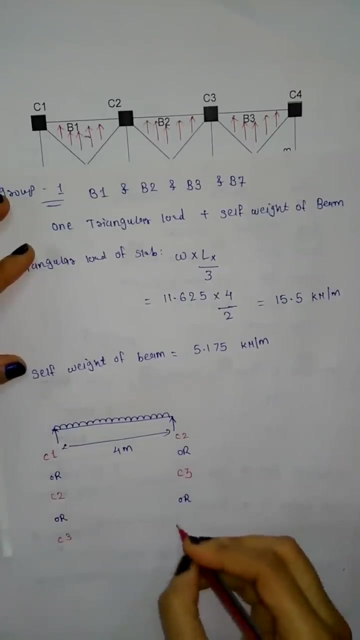 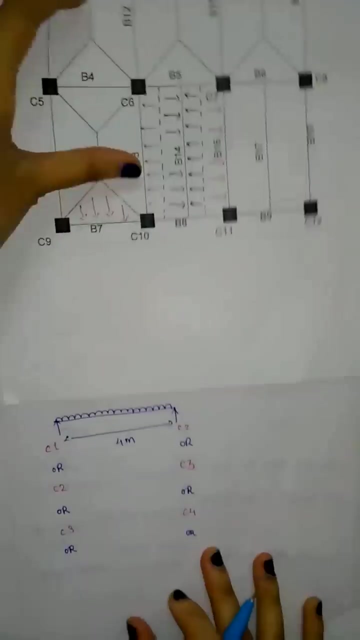 So it is here C2. And C3.. Similarly, if we consider beam number B3.. So you can see, The supports are C3 and C4.. Okay, Now if you consider Beam number B7. The supports are: 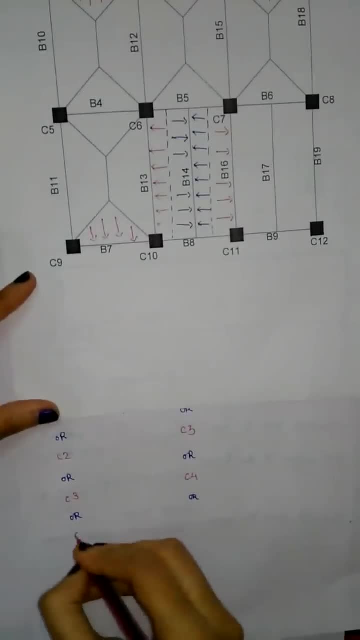 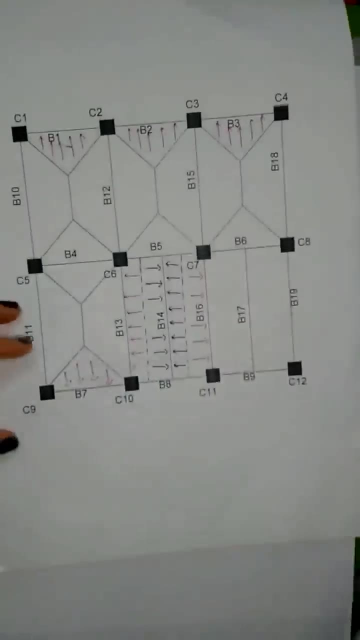 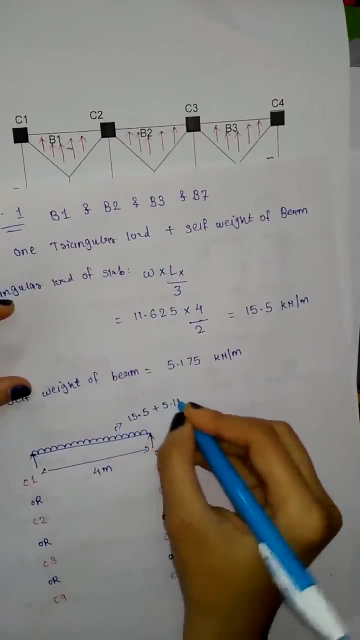 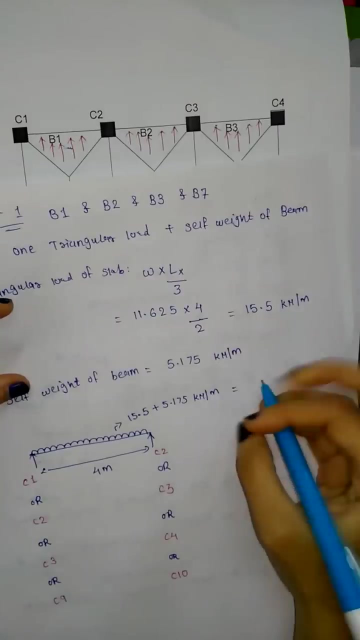 C9 and C10.. Okay, So now let's calculate the total load Here. the total load is 15.5 plus 5.175 kN per m. Right, So I think total will be Something 20.68.. 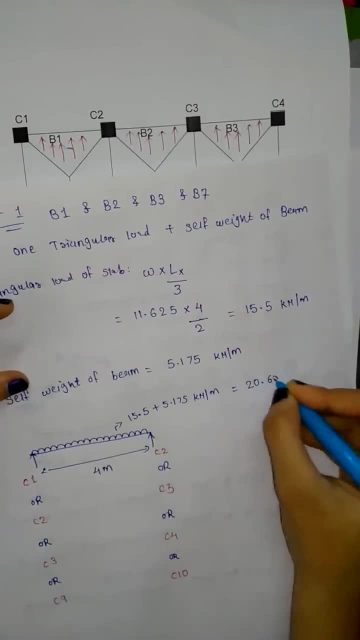 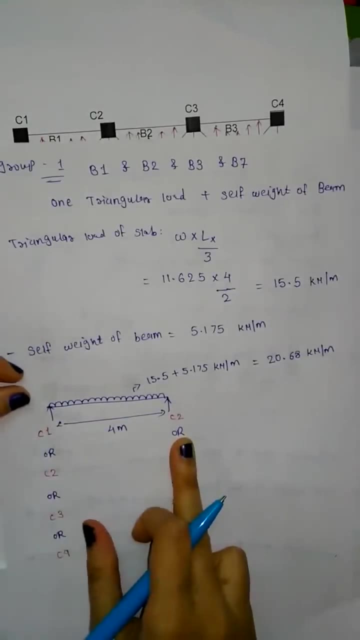 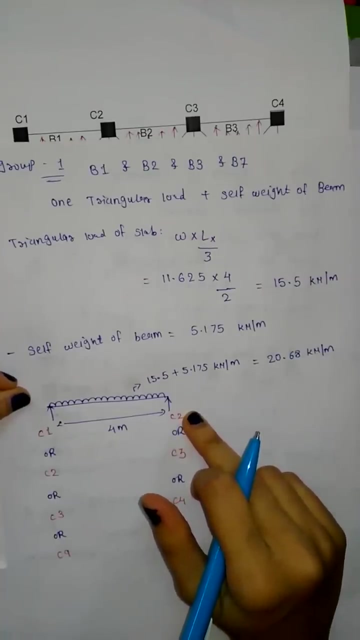 Kilo Newton Per meter. Now you have to determine the reaction For C1 and C2.. Having Beam simply supported UDL- Sorry, simply supported with subjected to UDL load. So I think the reaction will be something WL by 2.. 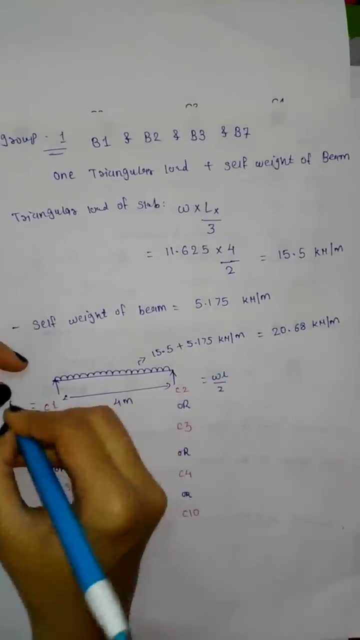 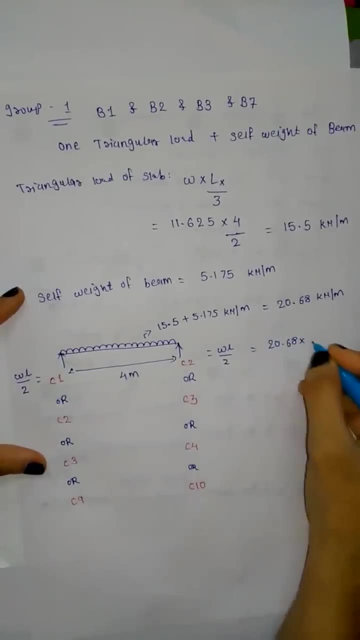 Similarly For the left side, WL by 2.. So here what is W? W is something 20.68.. Multiplied by L is 4 meter Divided by 2.. So the value is something 41.35 kN. 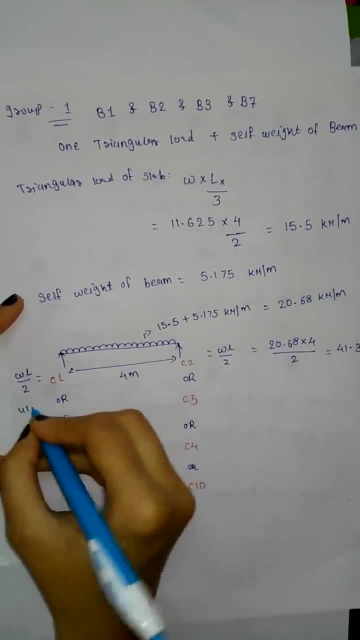 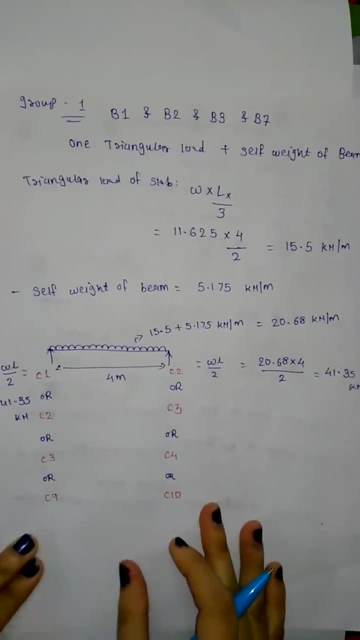 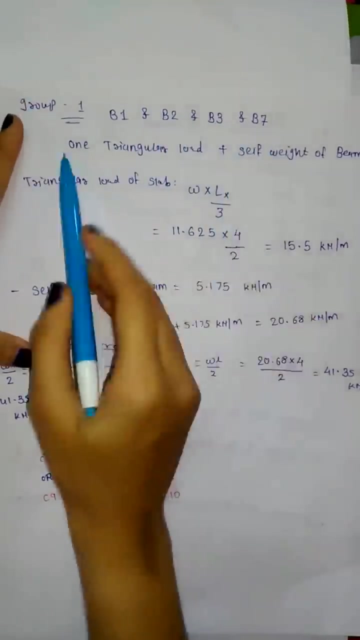 Similarly, here is 41.35 kN. Okay, So I think this is for group number 1. Having similar kind of load, Which is B1, B2, B3 and B7. Which is one triangular load Plus self weight of the beam. 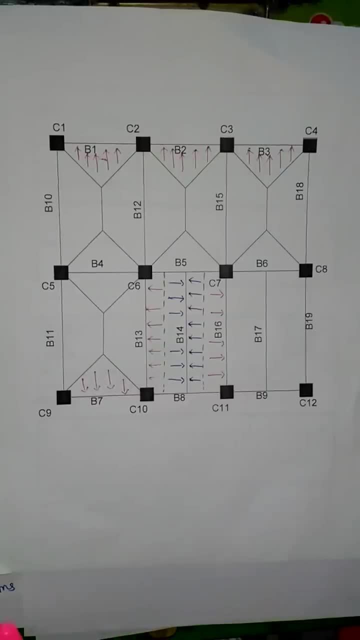 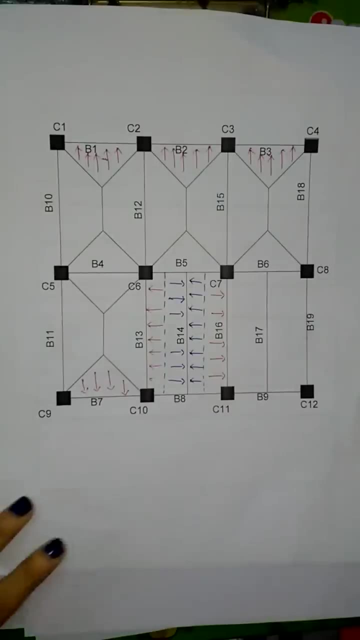 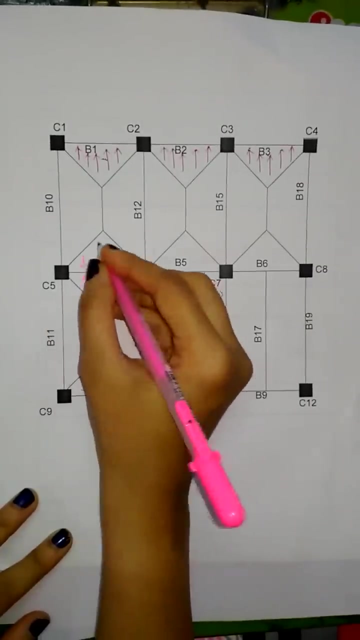 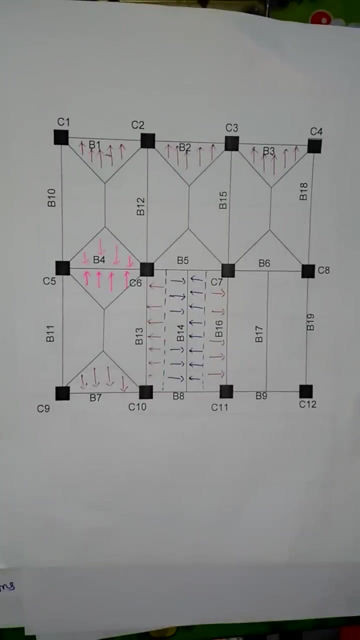 Now let's consider beam number B4.. So you can see beam number B4. Will be subjected with Two Triangular loads And you can see the Stretch Distribution. Sorry, it's a load distribution. Now let's calculate. 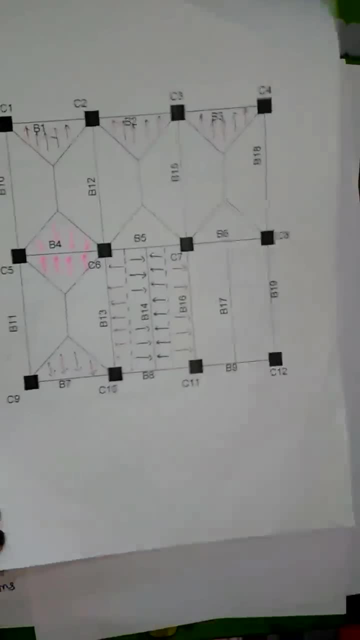 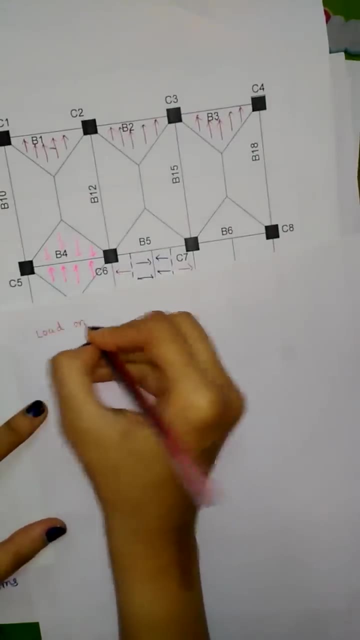 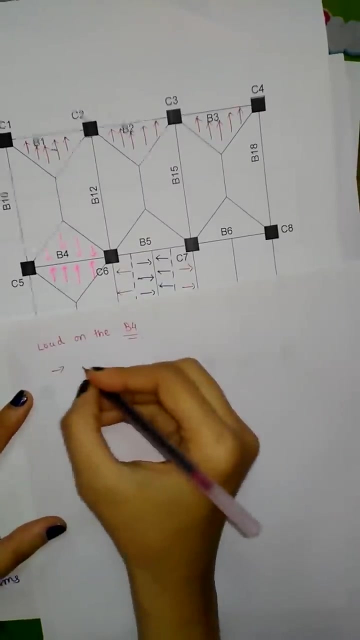 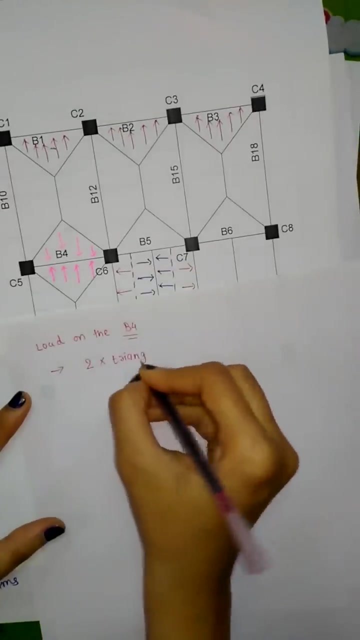 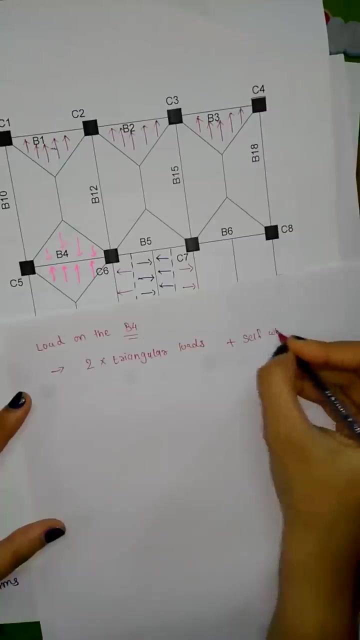 Now let's calculate load For the beam B4. Which Consider Which beam B4 is subjected with Two Triangular loads Plus its own self weight. You know that it is always be there. Self weight of beam. 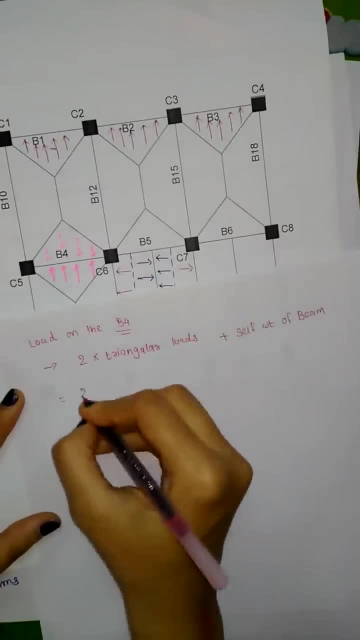 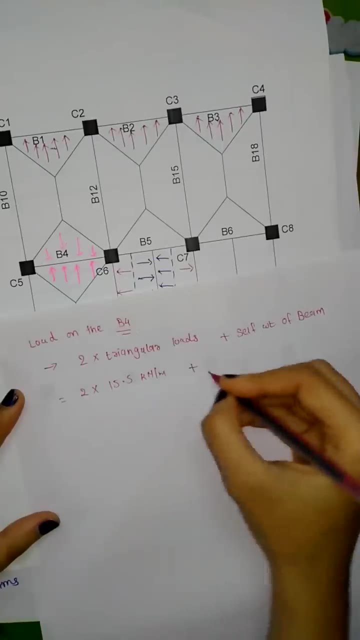 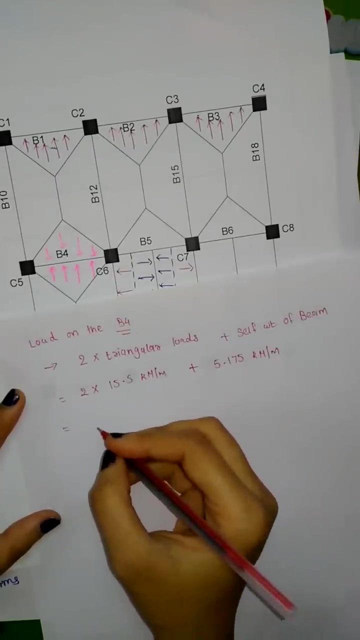 We already calculated triangular load, Which is 15.5 kN Per meter, Plus the self weight Of the beam Is nothing but 5.175.. kN Per meter. So if we calculate this Both, I think total. 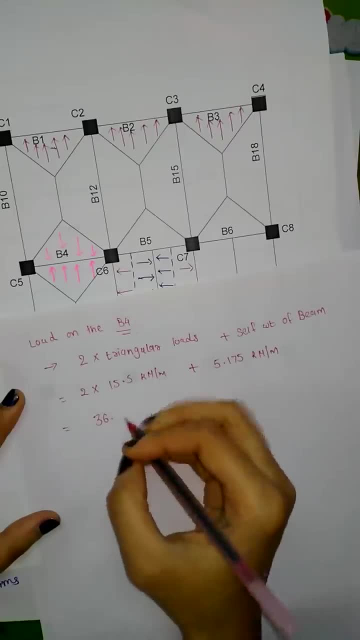 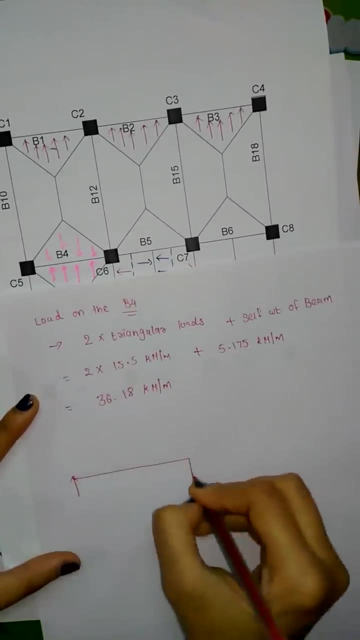 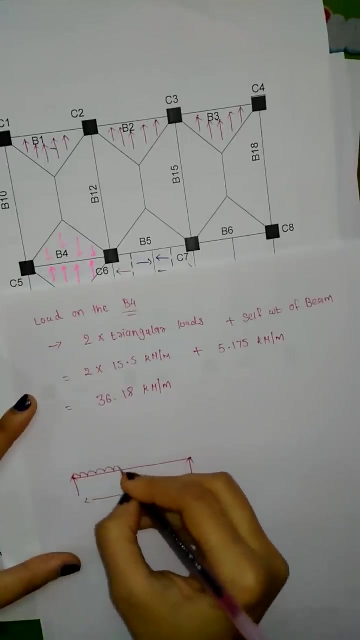 Value will be 36.18 kN Per meter. Now let's draw this beam, Beam number B4.. Having the length is 4 meter, It is subjected with UDL. Total UDL is 36.18.. 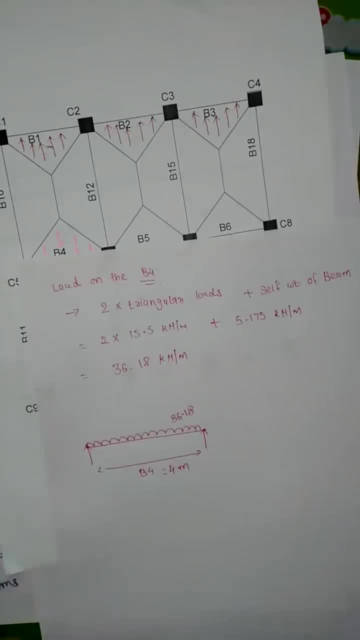 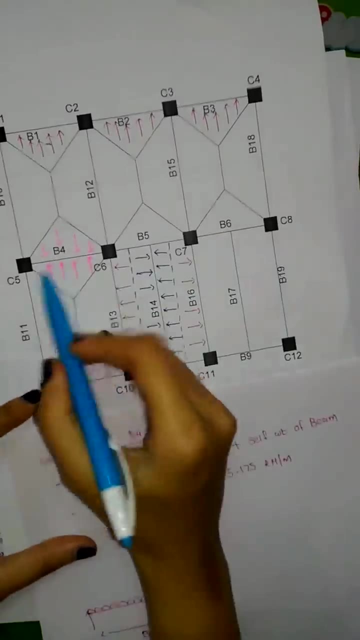 And now, if I want to consider, If I want to take Supports, The support You can see here. The beam number B4 is supported With two columns: C5. And C6. So you can write here C5. 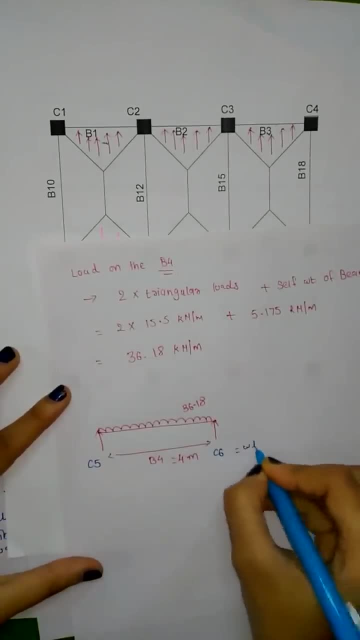 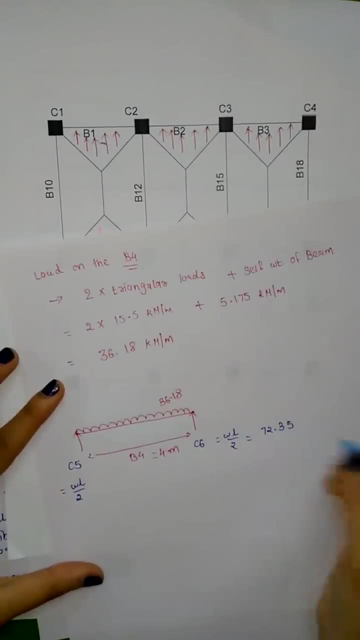 And C6.. So the reaction Will be WL By 2.. WL By 2. And the values are 72.35.. Which is This is kN Per meter And these are the kN. 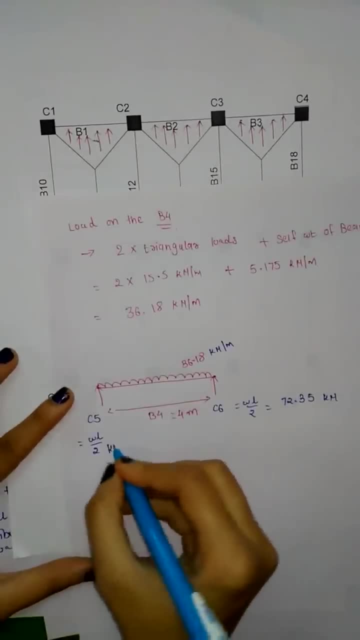 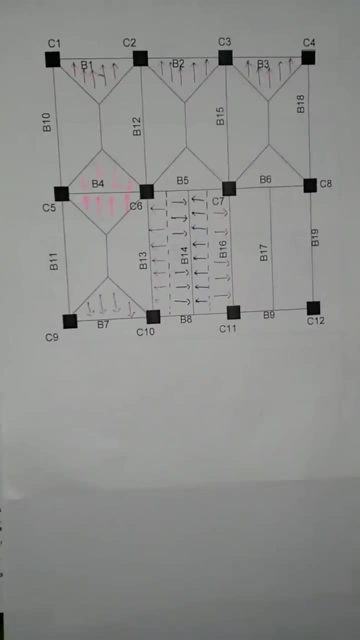 Okay, So this is, I think, Another type of the Group, Group number Two. Now let's take Other beams. Let's take B10., B11. And B 18.. Now you can see Beam number. 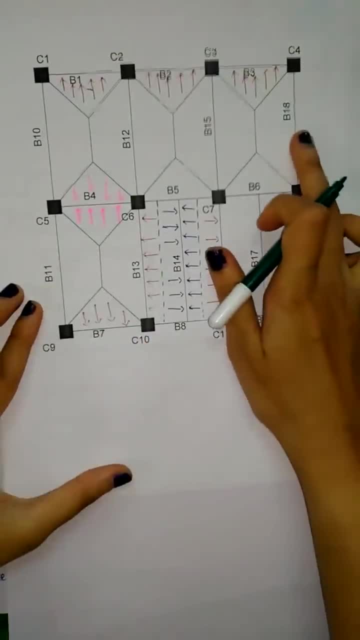 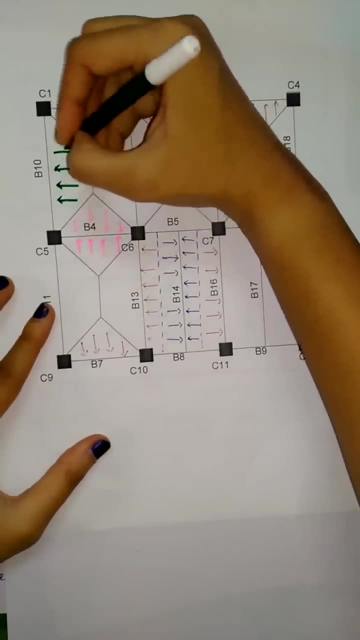 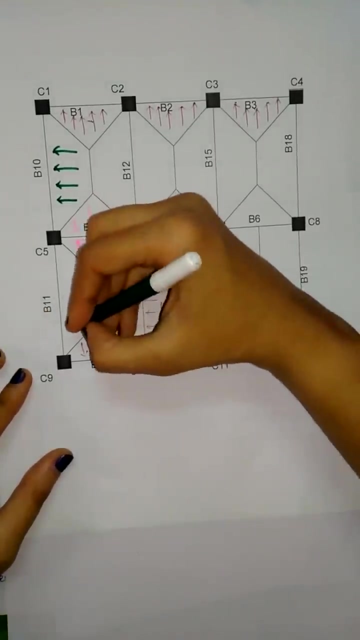 B10. Is subjected With One Trapezoidal Type of Load Plus its own Self weight. Similarly, B11. Is also having Same kind of Loading Distribution, Which is One Trapezoidal. 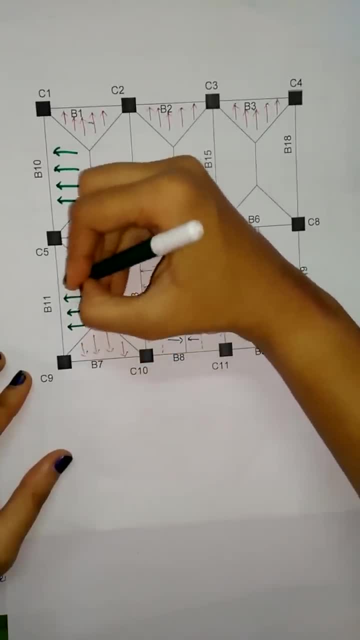 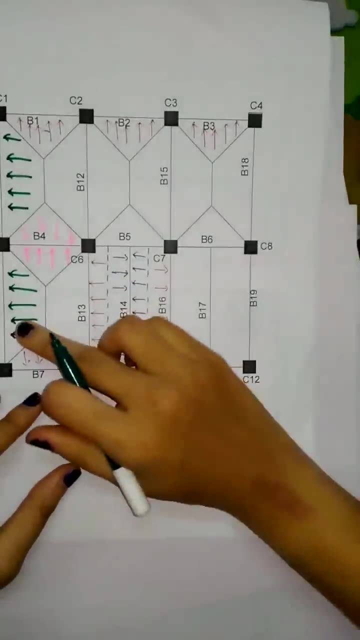 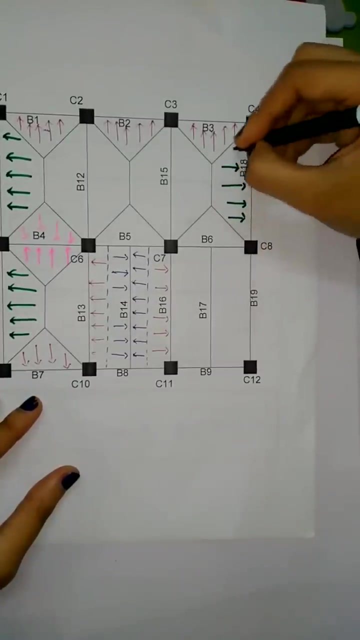 Load Plus its own Self weight. You can see The direction Also. Okay, With this Green Highlighted Lines And With B18.. It is also Subjected With One Trapezoidal. 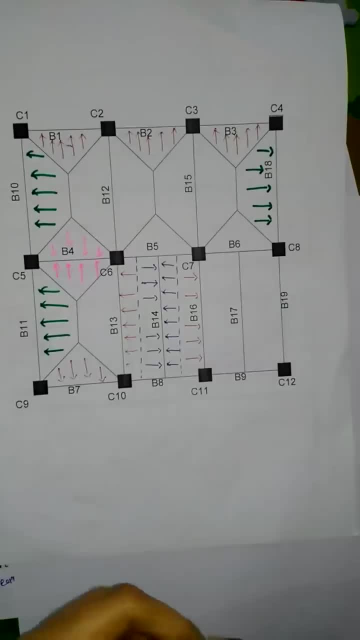 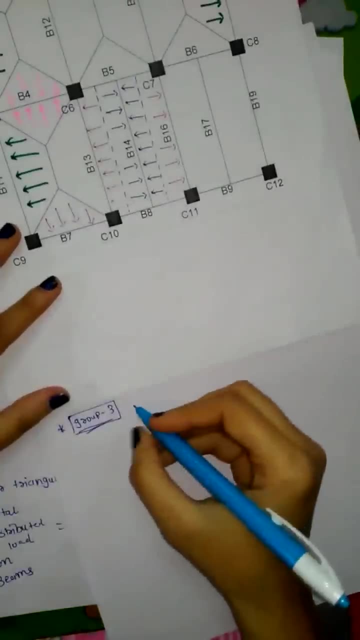 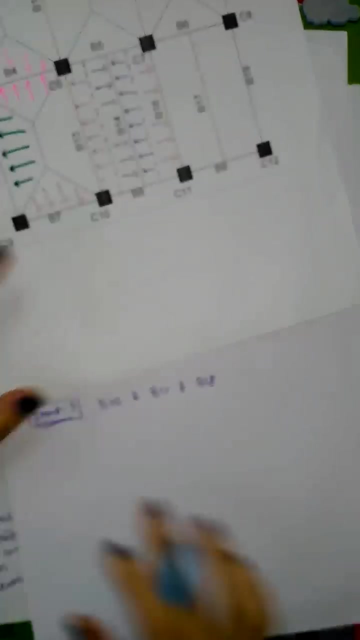 Load Plus its own Self weight. Okay, Now let's Calculate The loads, For I think It will be. The group Number Three Is B10.. B11. And B18.. So 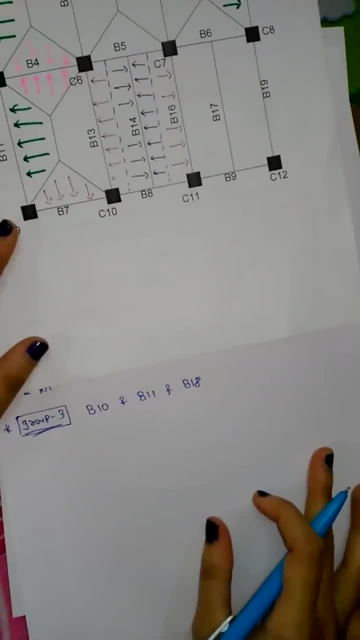 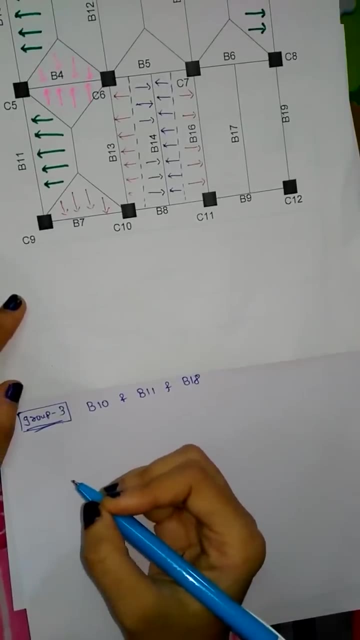 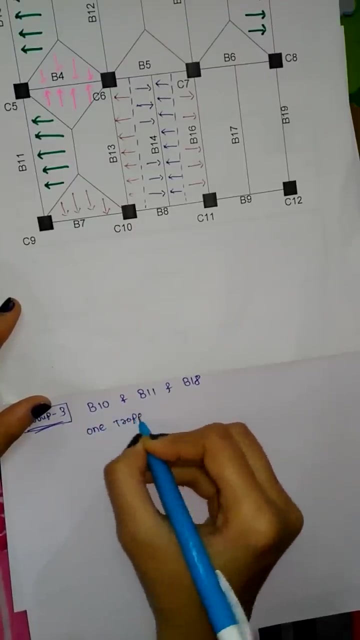 The group Number Three Is B10., B11. And B18. Which Is Subjected With One Trapezoidal Load Plus The Self Weight. So The group Number 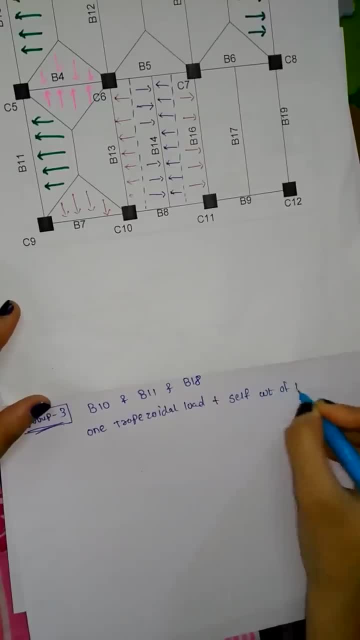 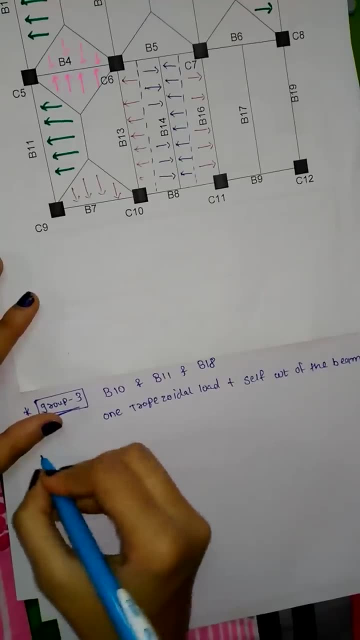 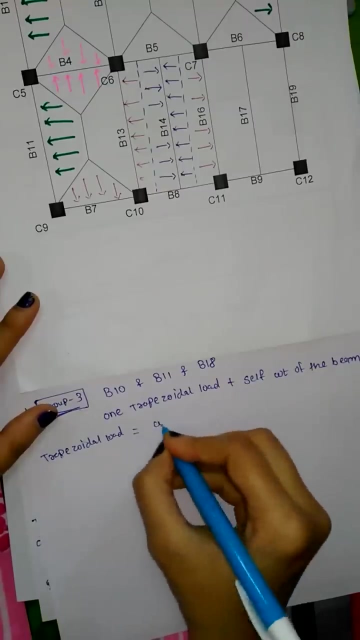 Three Of The Beam. I Think We Have To Calculate Trapezoidal Load As Per The Formula. It Is W LX By Two, One Minus. 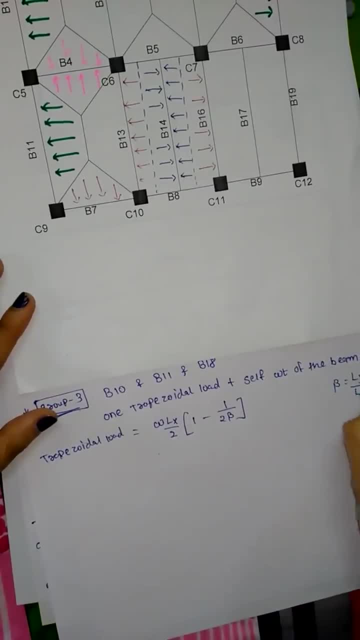 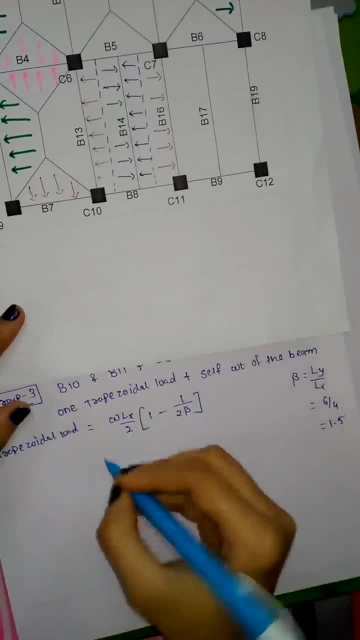 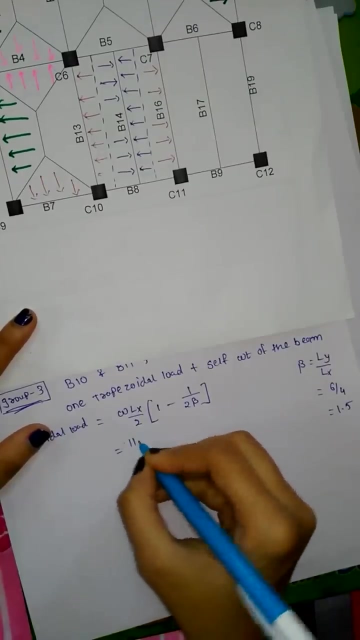 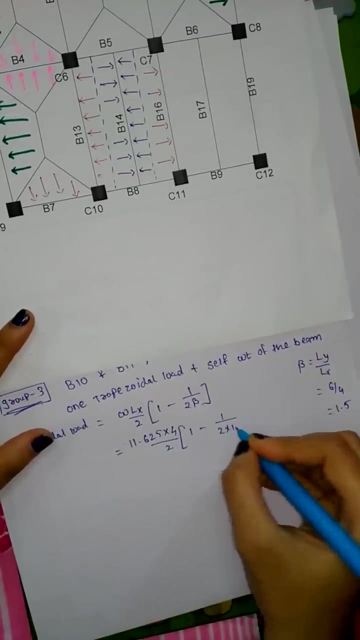 One Upon Two Beta, Which Is One Point Five. If I Put The Values, The W Is Total Load Of The Beam, Which Is Something Eleven. 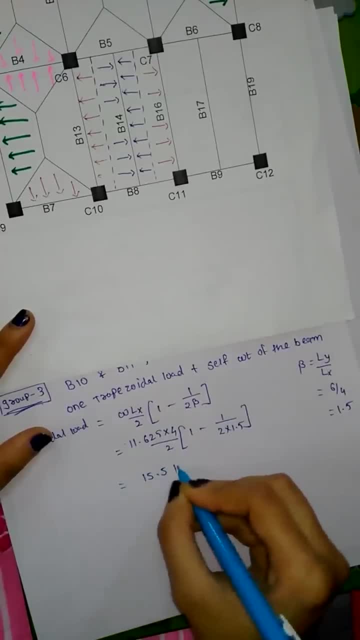 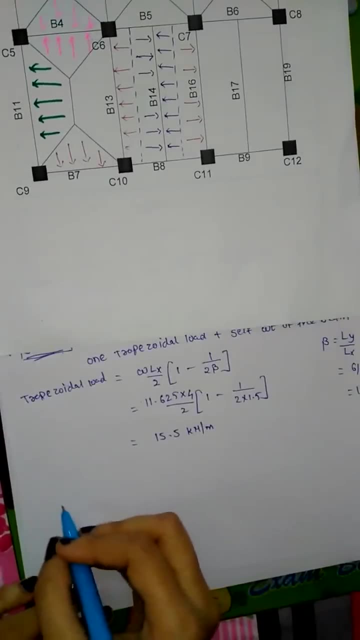 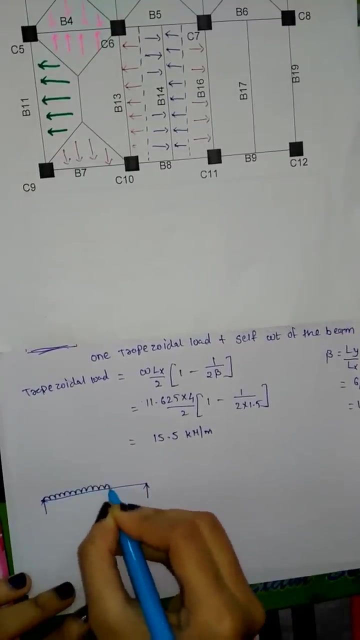 Point Six. Twenty Five Multiplied By Four, By Two Effective Beams Ten Eleven. Sixteen Having The Length Six Metre, Sorry Be number Ten Eleven. 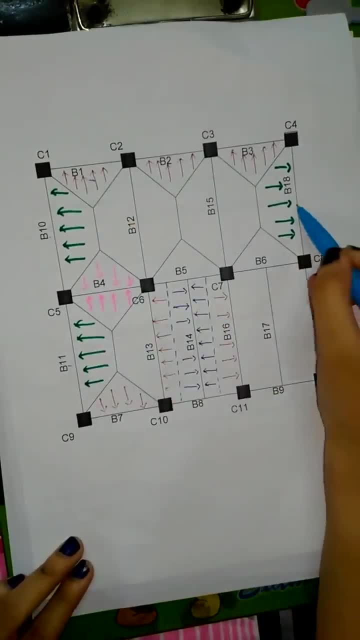 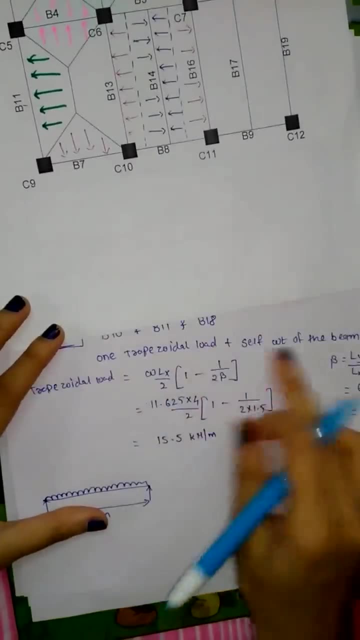 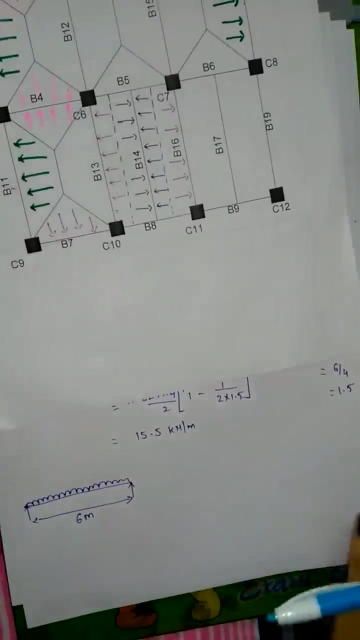 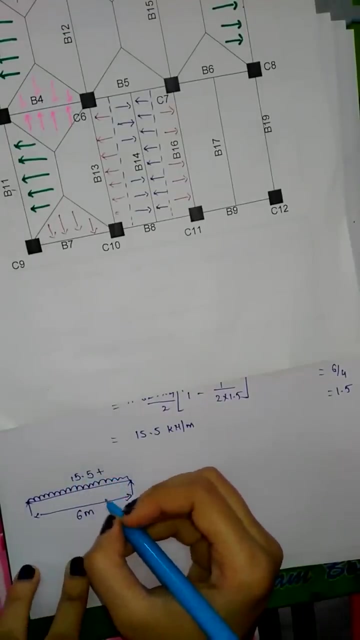 Number Eighteen. Having The Length Six Meter, You Can See Here It Is. Subject With One total, udl is 15.5 plus the self weight is nothing but something 5.175, so 5.175 it will be. total is: 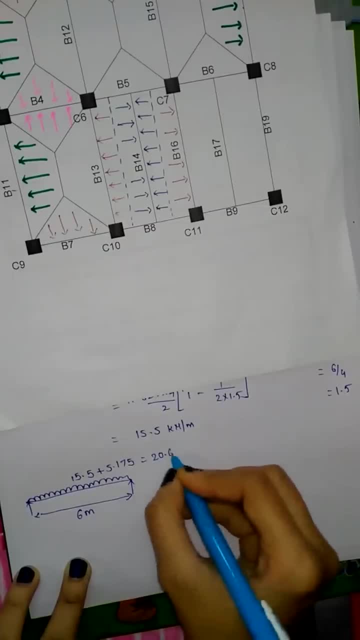 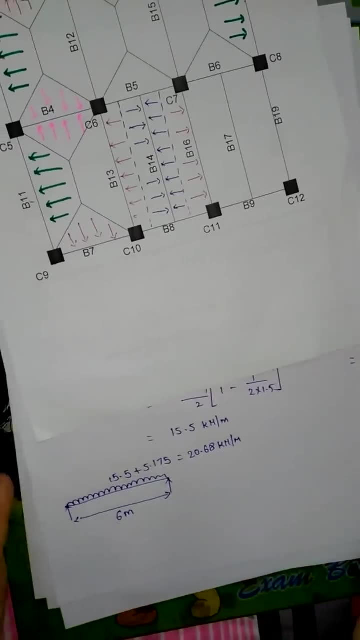 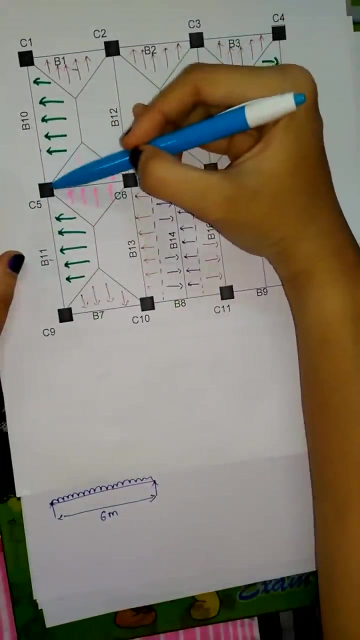 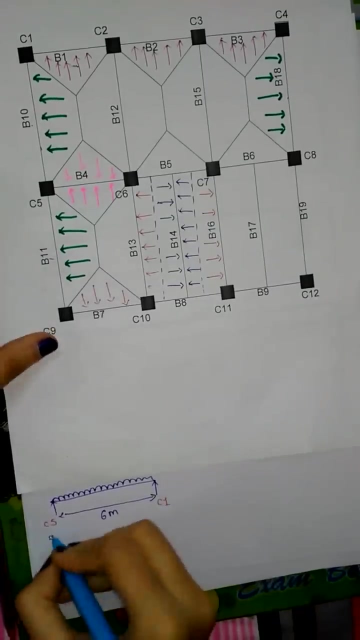 20.68. okay, which is kilo newton per meter, but we have to take care for the supports for the different beings. and if we are taking beam number b10, you can see the support is c5 and c1, so let's write c5- c1. or if i am taking beam number b11, with the supports will be c9 and c5. 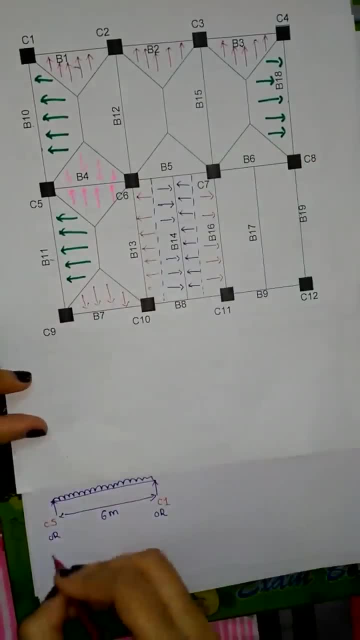 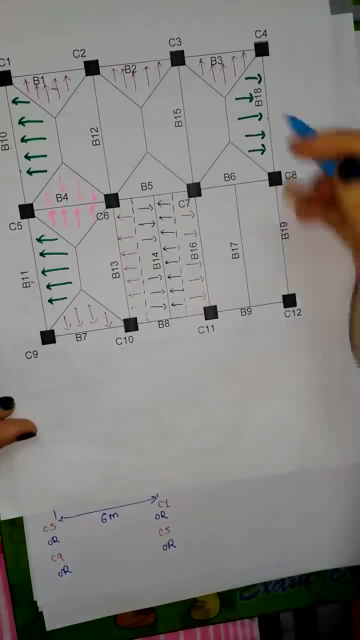 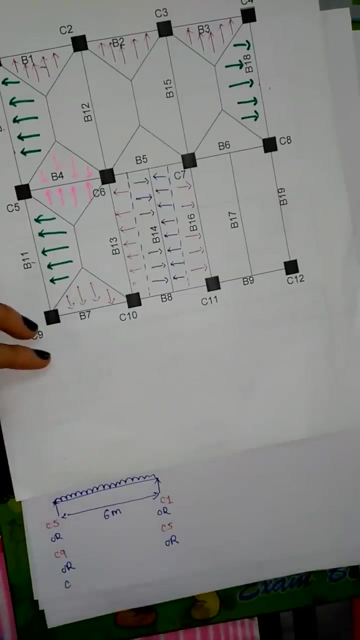 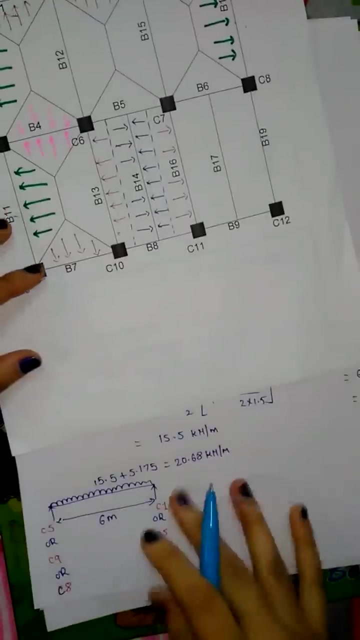 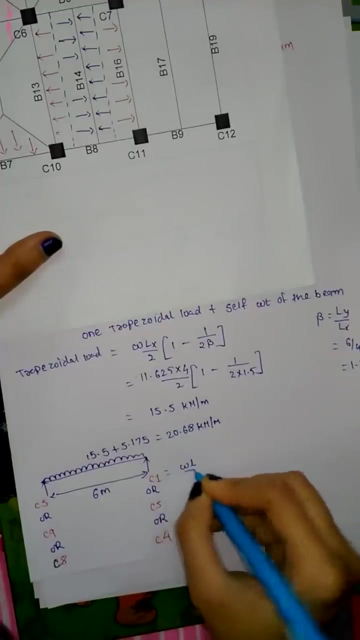 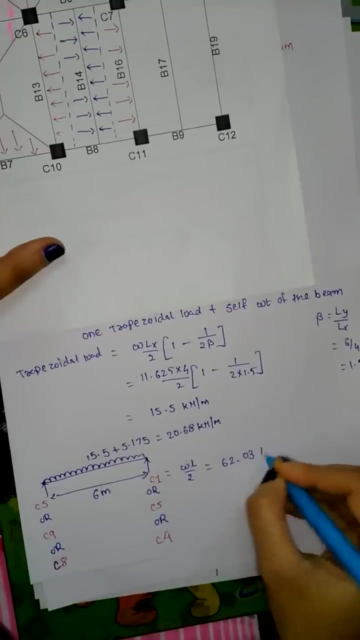 similarly, if i am taking b18 it's having supports c8 and c4. so if i have total load on the beam is 20.68. so the reactions will be wl by 2, wl by 2 and the value will be 62.03 kilo newton from the both side reactions. 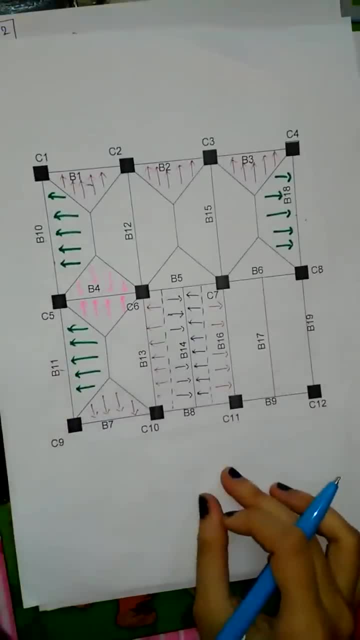 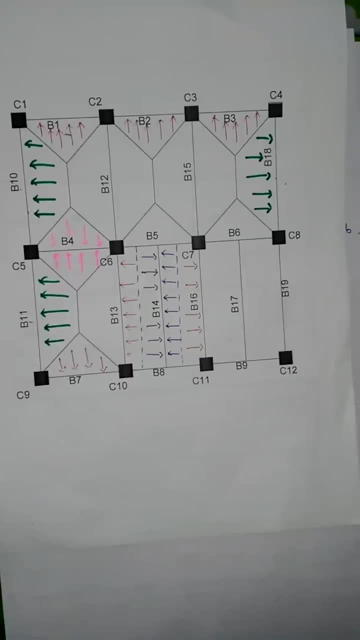 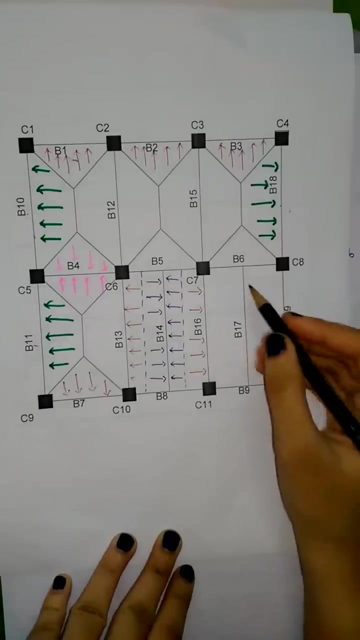 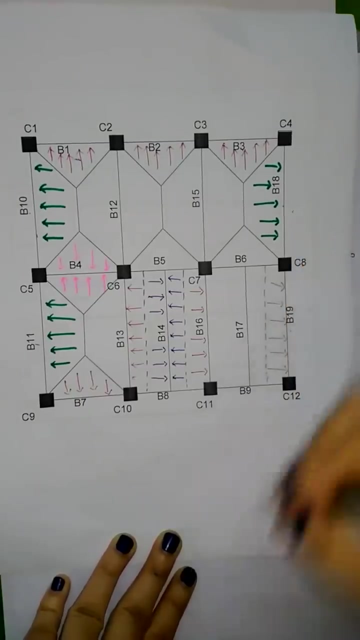 now consider beam number b19. you can see these slab panel is behave as one way slab. so beam b19 will be subjected with half of the rectangular load. remember谢谢 for watching this video- XOXO. the rectangular load from this direction plus its own self weight. okay, so let's. 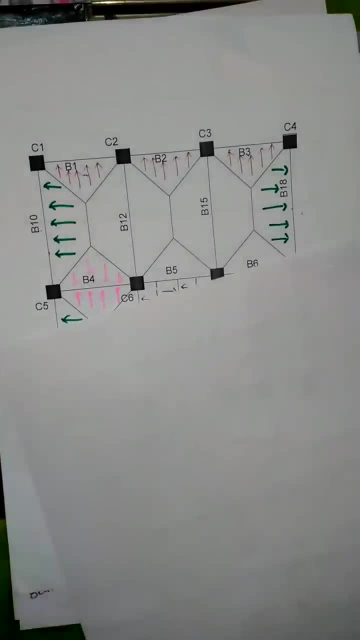 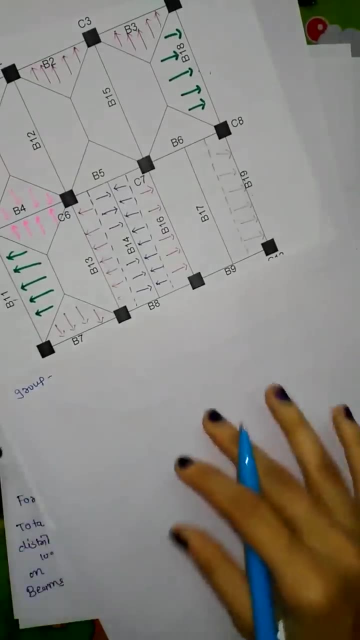 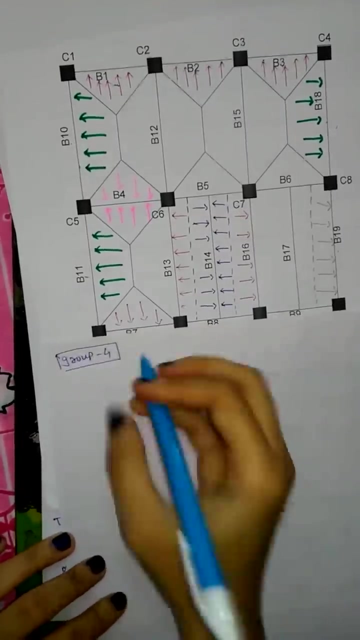 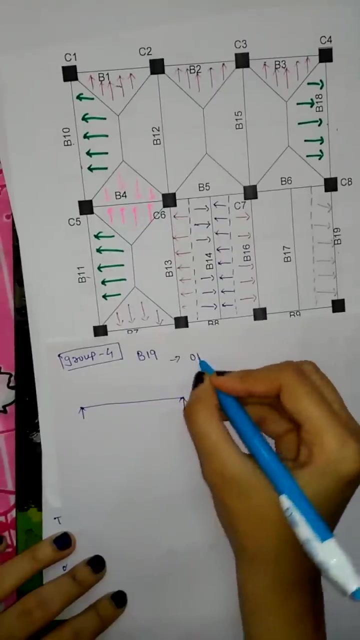 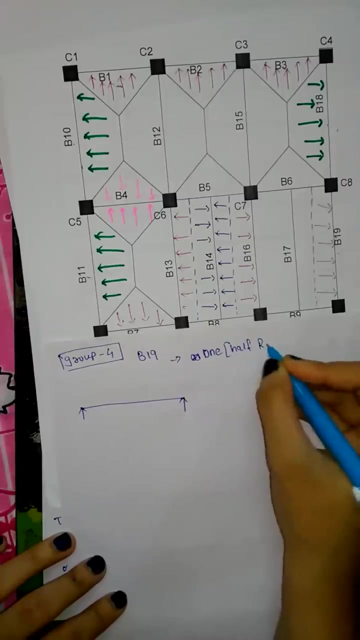 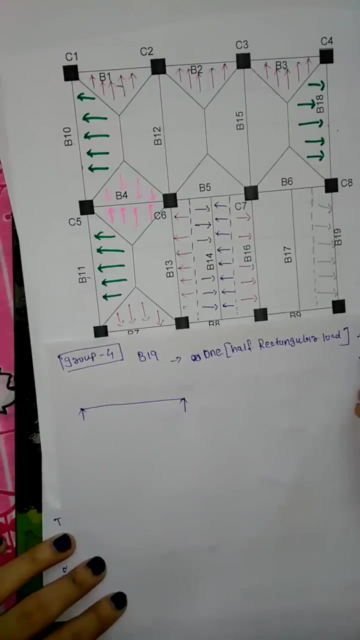 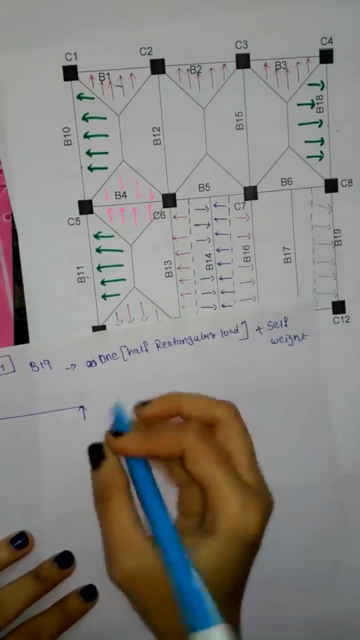 calculate load for the B19. I think it will be group number 4, which is B19. let's draw it. it is subjected with one but half rectangular load plus self weight. it is subjected with B19. let's draw it. it is subjected with one but half rectangular load plus self weight. 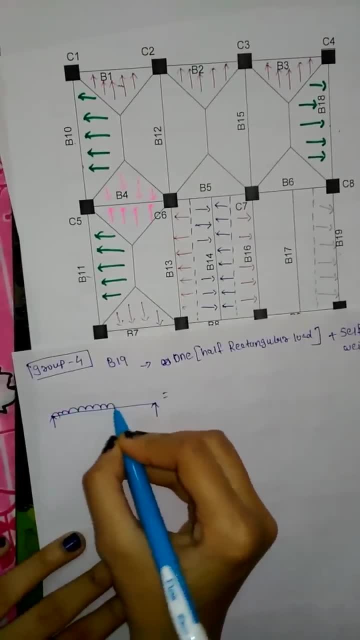 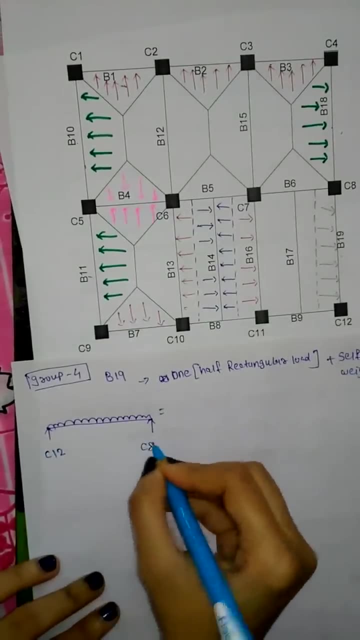 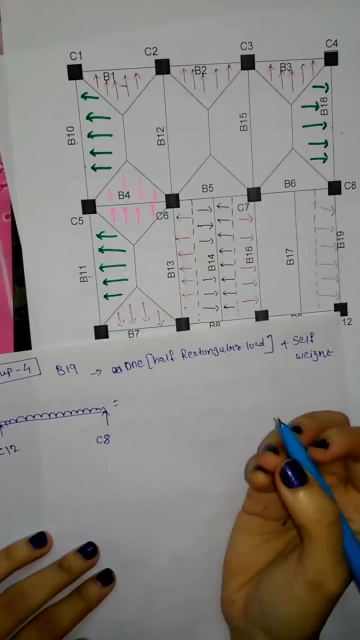 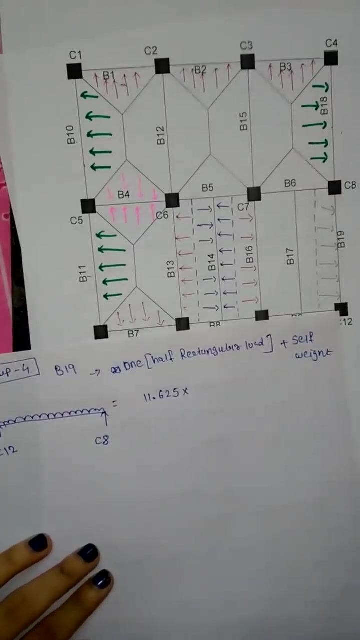 UDL and the support is C12 and C8. now calculate the UDL. so half rectangular load is, we know that to complete slab load is something 11.625. and if it is half of the load, multiply by LX, by 2, plus the self-fit of the. 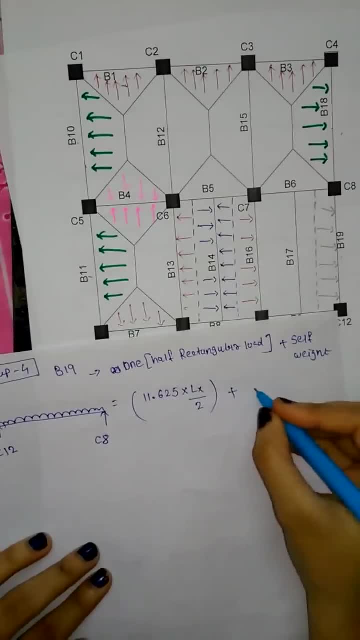 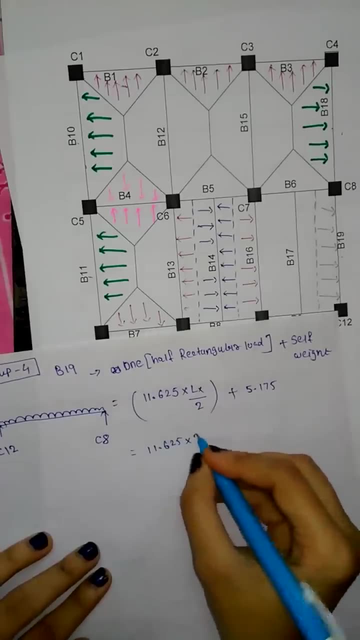 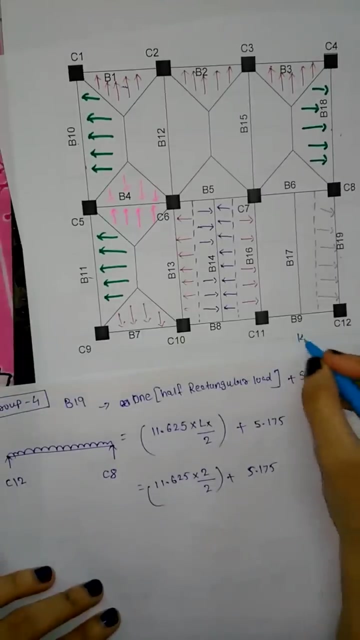 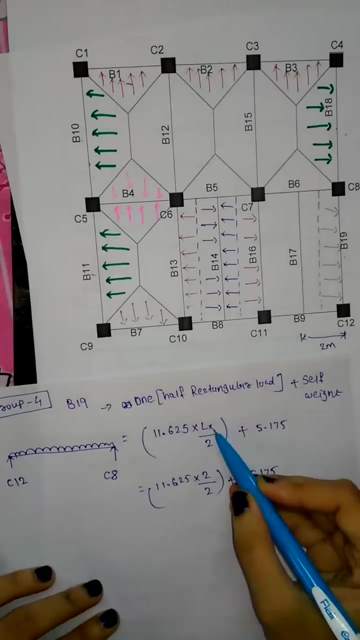 beam is 5.175, then 11.625 LX is 2 meter by 2 plus 5.175. you know that that complete slab length is 2 meter. so, if I can do, LX is 2 divided by 2 and the total value. 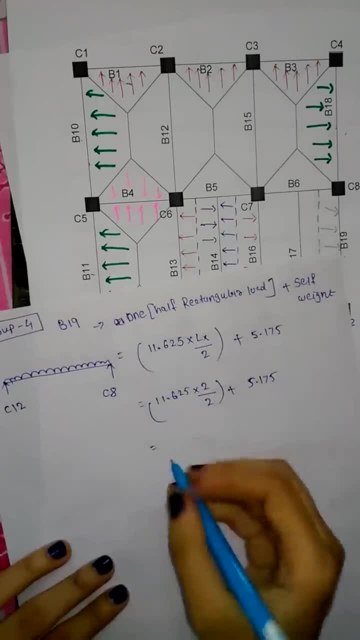 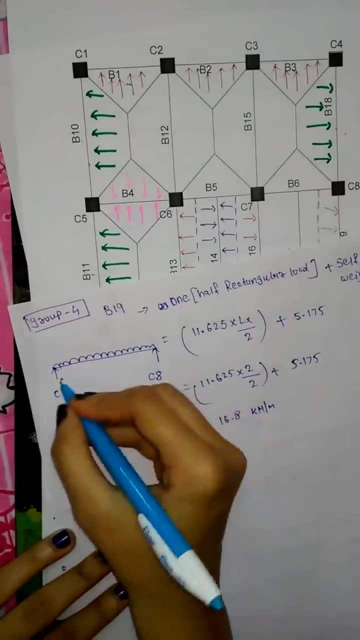 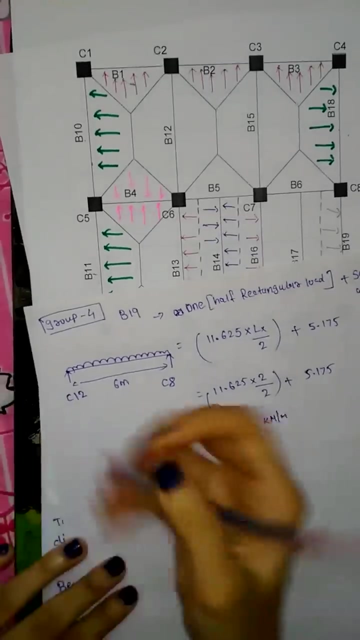 will be 16.8 kilo Newton per meter. so you can see that beam number B19, having a length is 6 meter, which is subjected with 16.8 kilo Newton, and the reactions will be WL by 2, WL by 2 and the values are: 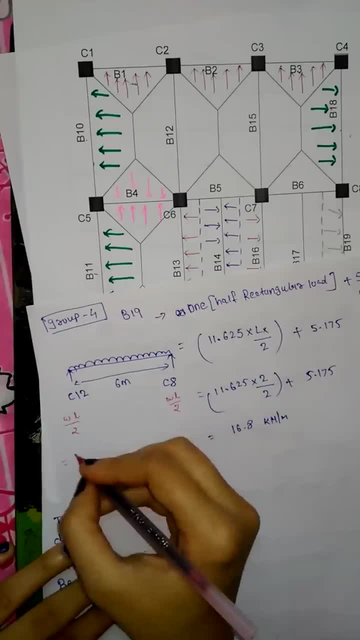 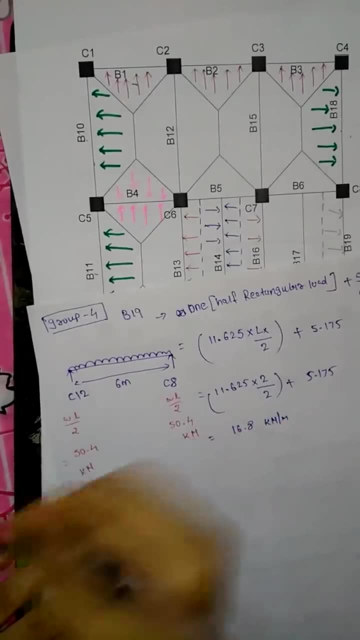 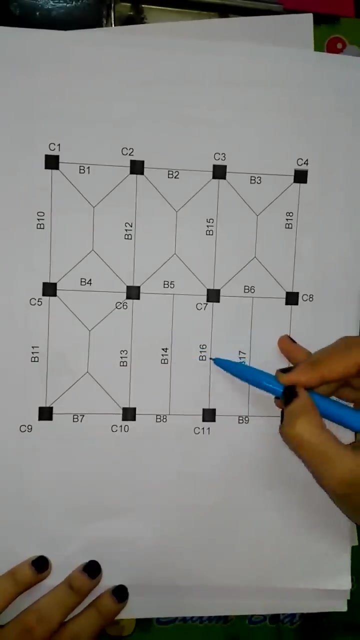 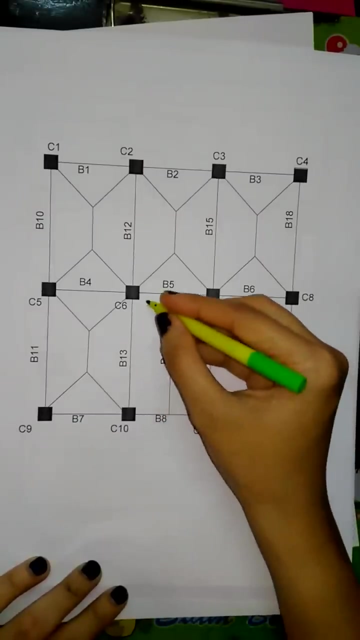 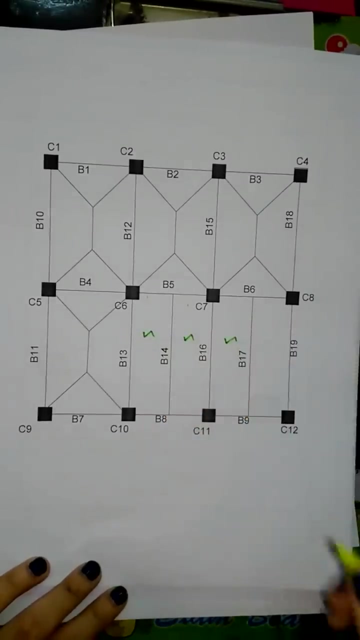 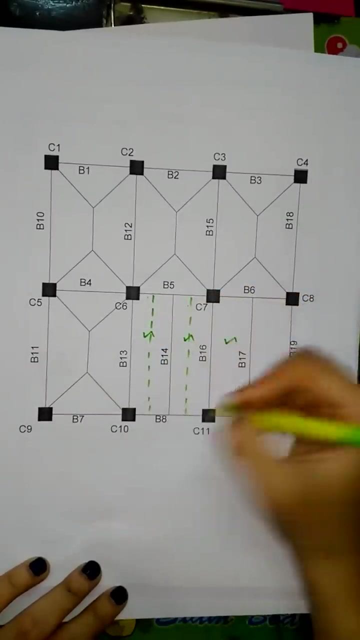 50.4, 50.4 for the both side reaction. similarly, consider for the beam number 14, 16 and 17. for that you know that these three panels are act as a one-way slab, so half of the slab load will be act on the beams, so half of the slab load will be. 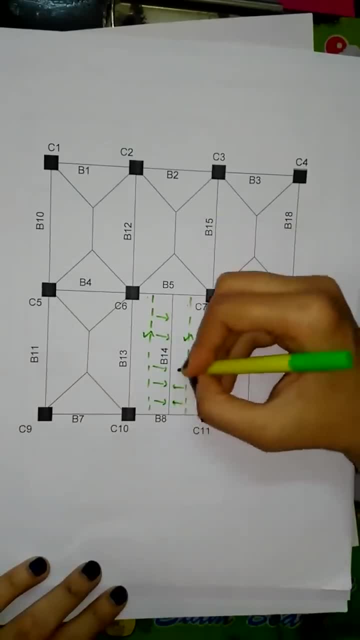 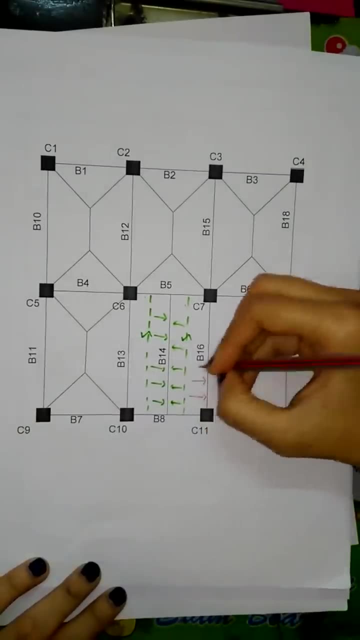 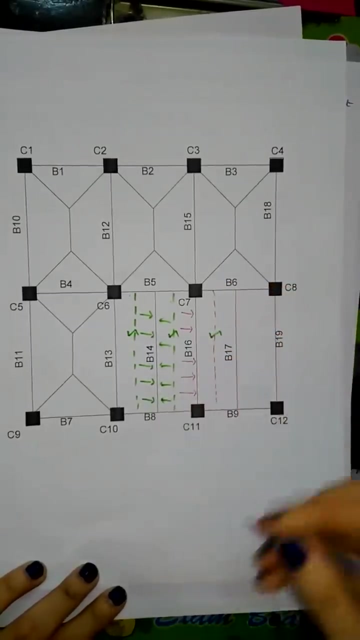 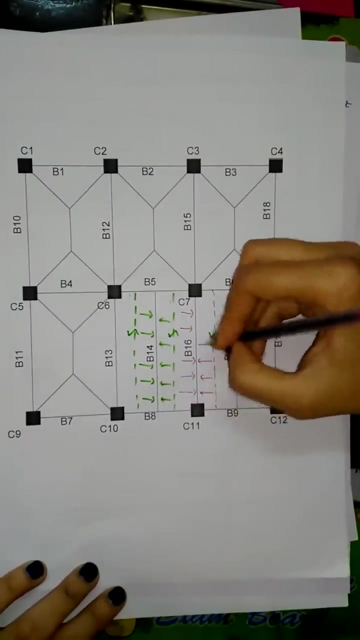 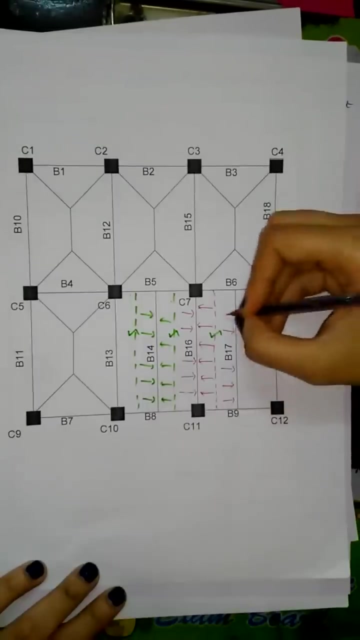 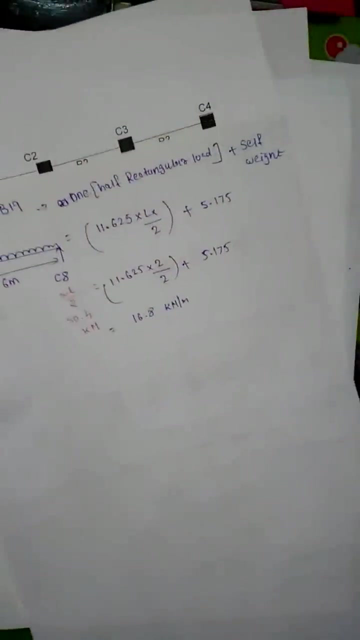 act on these beams. similarly, half of the slab load will be act on beam number 16, same as we have to divide this slab in two portions and half of the slab load will be subjected on the B16 and half on the B17. so if we want to calculate this, and this will be our group number 5 and the beams, 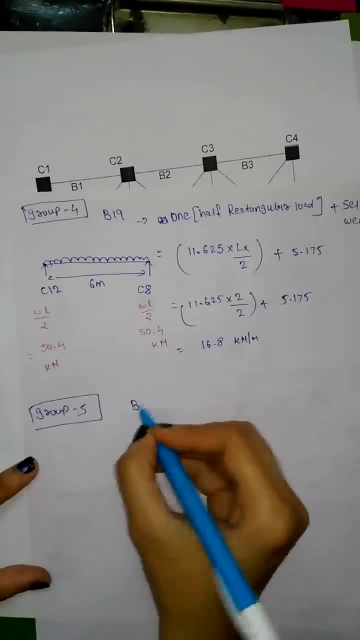 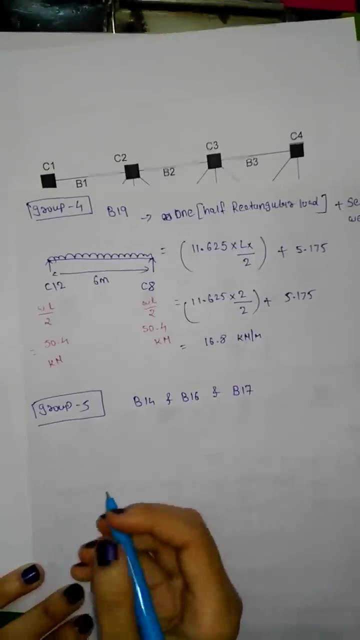 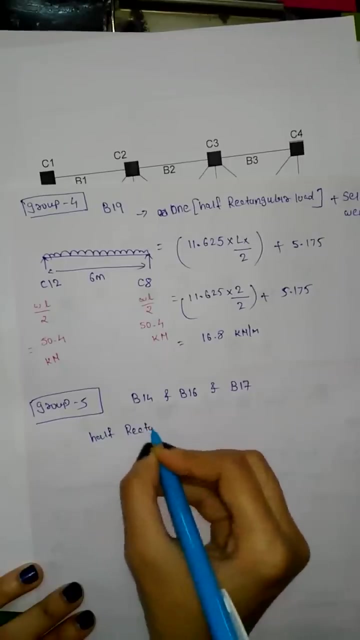 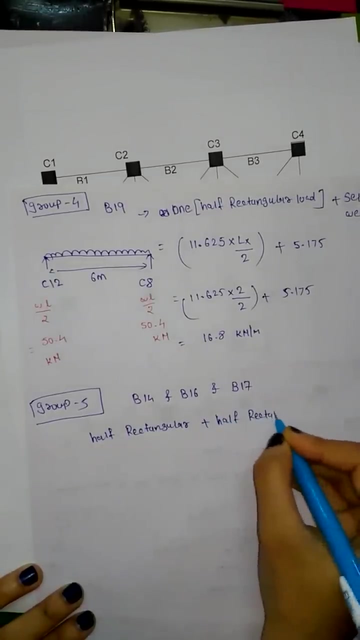 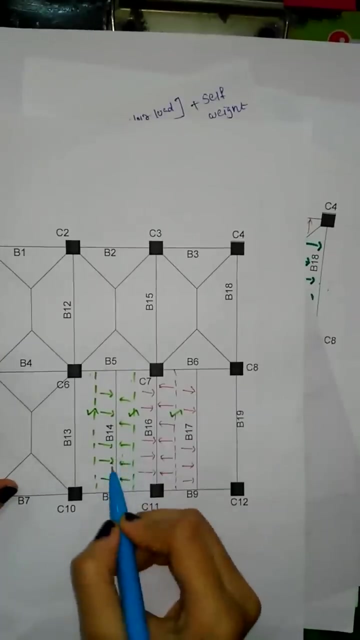 are B14, B16 and B17. it will subjected with half rectangular load plus half rectangular load. you can see these beams are subjected with two times half of the rectangular load. okay, half of the from the D slab and half from the D slab. so is half of the rectangular load plus half. 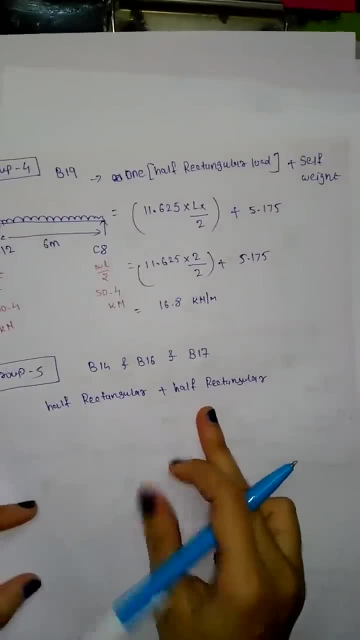 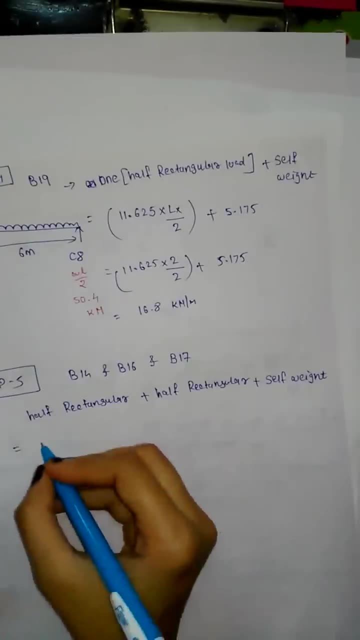 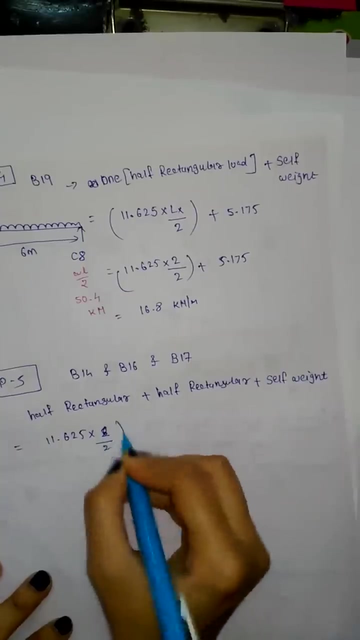 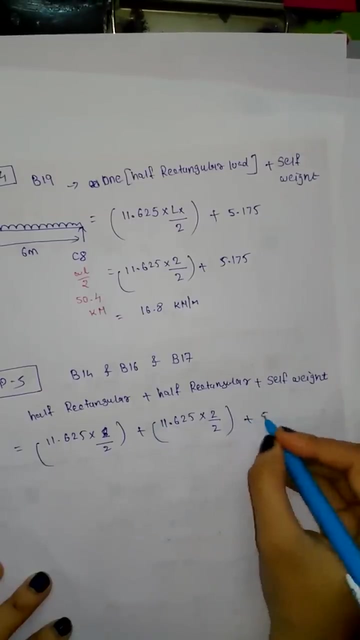 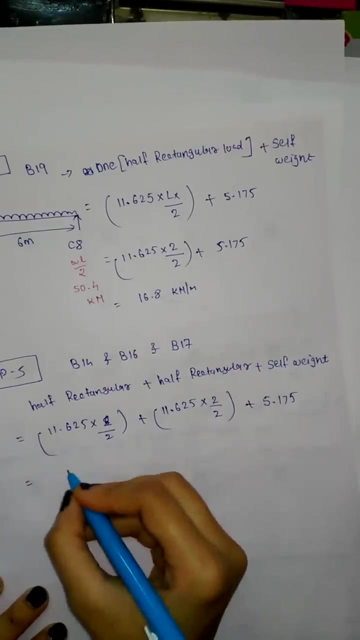 rectangular load plus self weight. so rectangular load, half of the rectangular load, are 11.625 x 2 by 2 plus 11.625 x 2 by 2 plus 5.175. so the total value is 28.43 kilo newton per meter. now lets draw with the supports. it is. 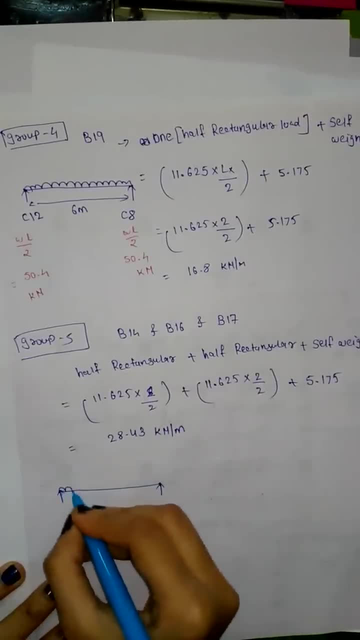 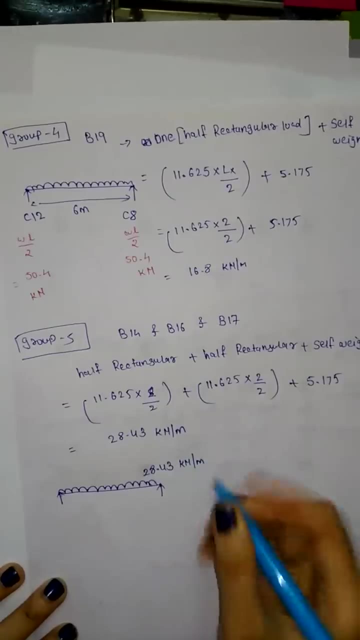 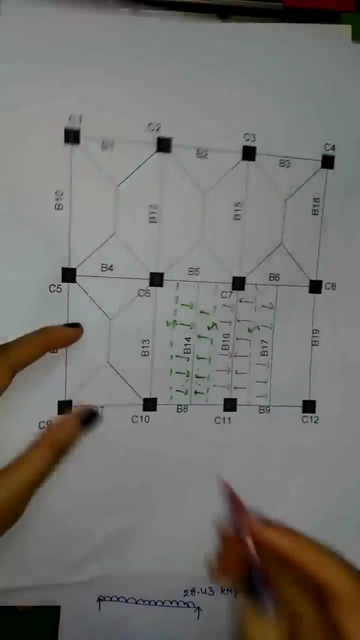 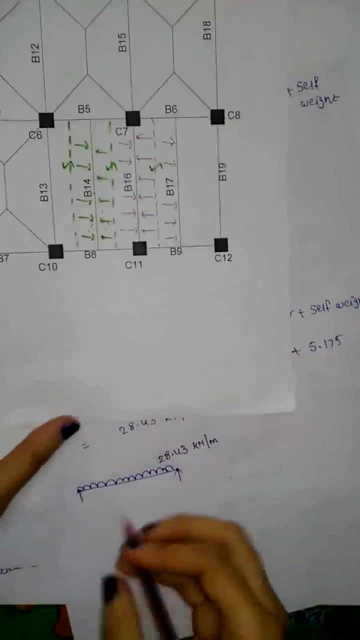 subjected with udl having value 28.43 kilo newton per meter. now, if I am taking beam number b14, you can see here: if I am taking beam number b14, The supports are B8 and B5.. If I am taking beam number 16.. 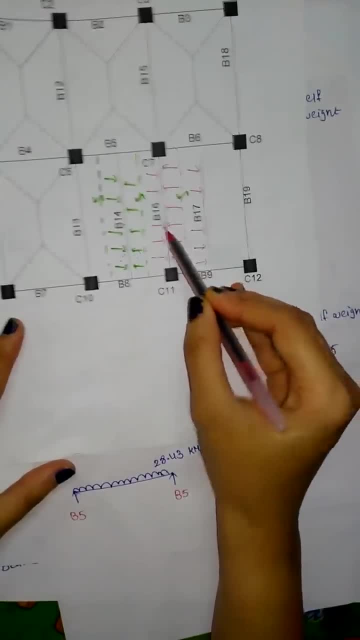 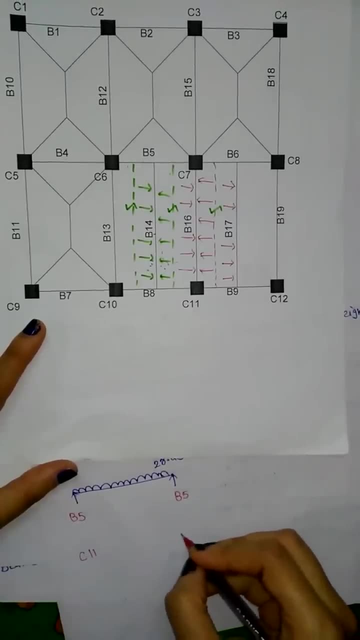 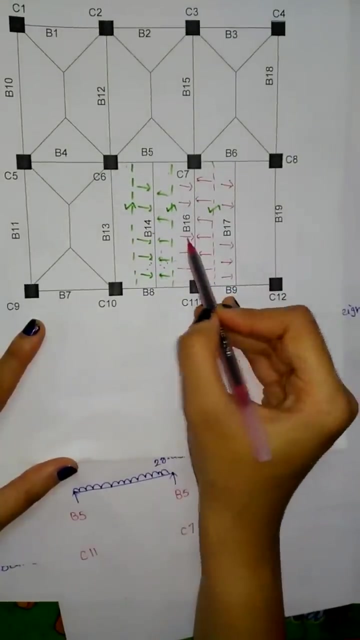 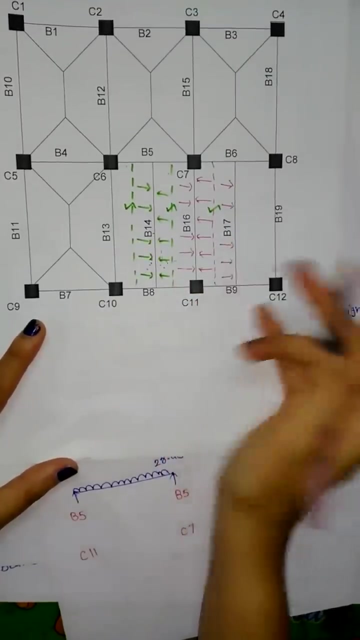 The supports are C11 and C7.. I think we already discussed about primary beams and secondary beams. So the beam number 16: here it is primary beam, But beam number 14 and 17 are the secondary beams. Now for the 17. the supports are B9 and B6. 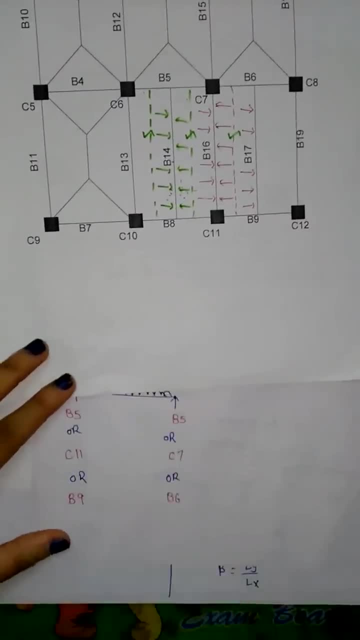 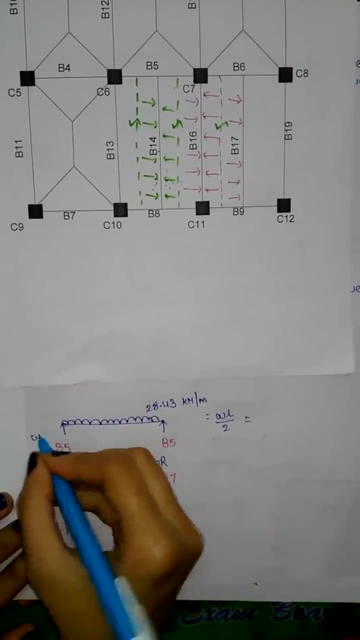 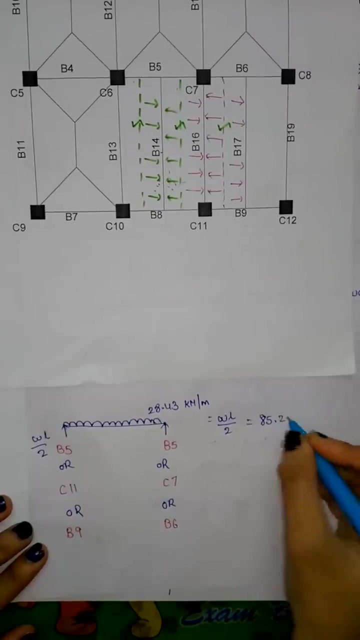 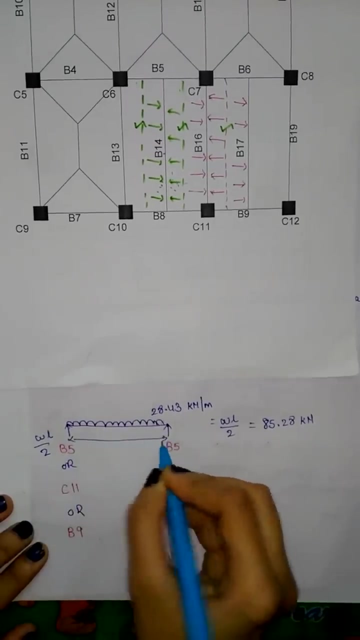 Okay, So the both reaction, both side reaction, will be WL by 2.. WL by 2. And the reactions are 85.28 kN. Okay, And the length of these beam is 6 meter. You can see, this length of the beams is 6 meter. 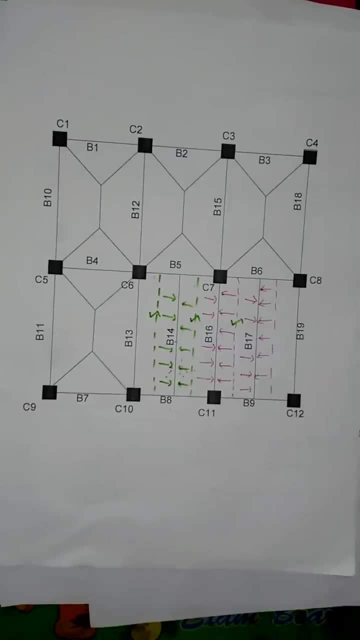 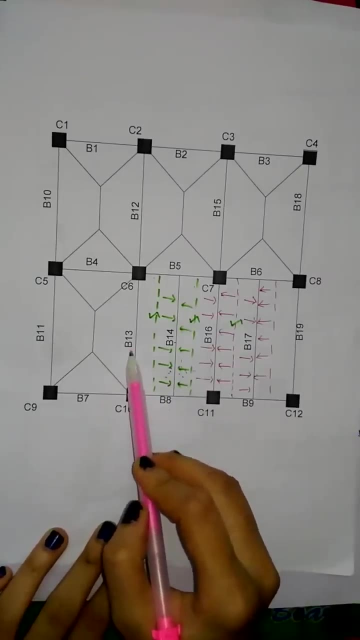 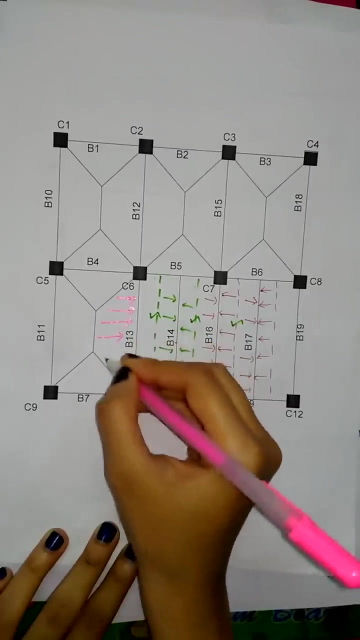 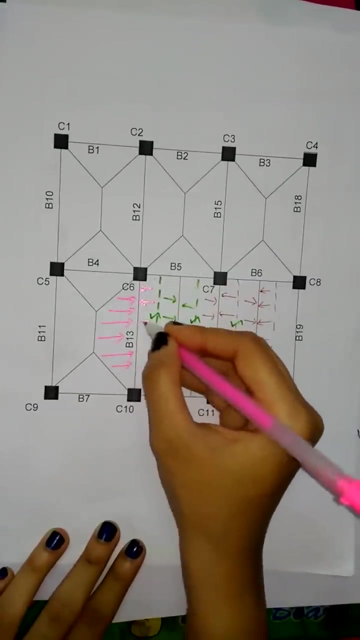 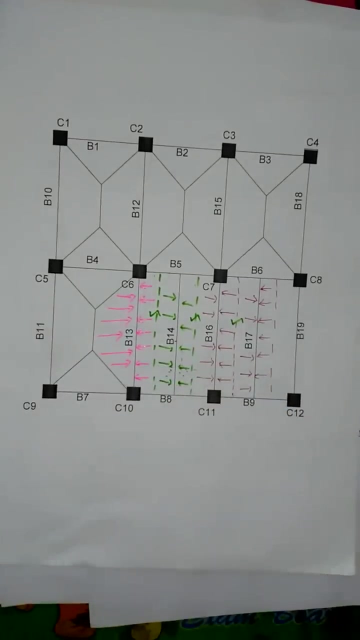 Now consider beam number 13.. Beam number 13 is subjected With one portion from the D-slab subjected as trapezoidal load, and from the either side it is subjected with half of the rectangular load You can see here. So plus self weight of the beam. 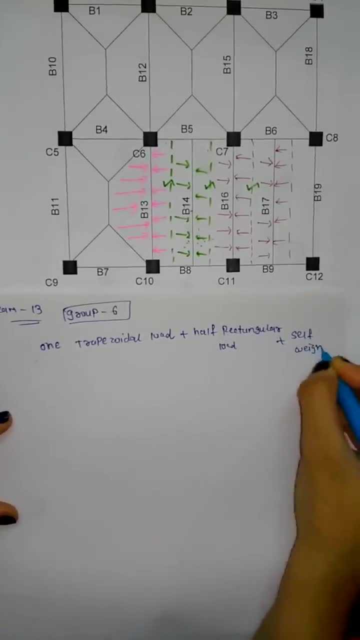 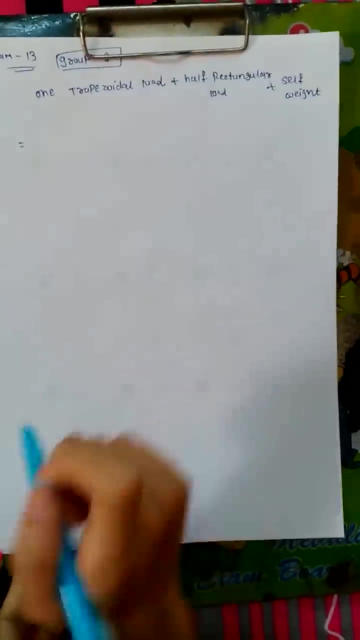 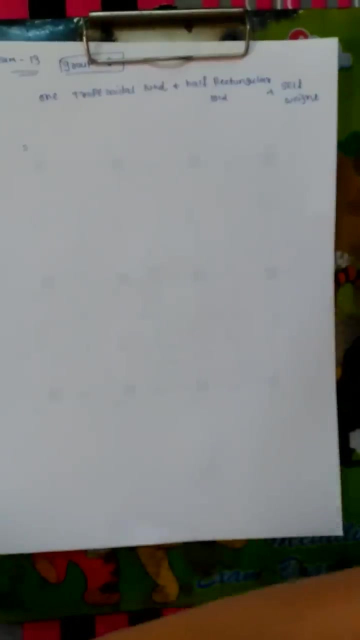 Now let's take beam number 13. it's a group number 6 and you can see here this one trapezoidal load plus half rectangular load plus its own self weight. Let's understand with the figure. okay, here is a beam number 13, you can see, and it is. 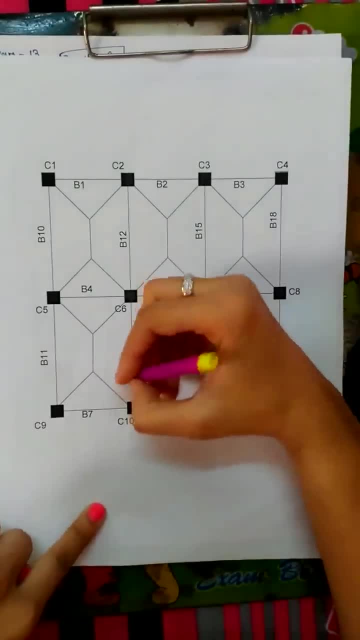 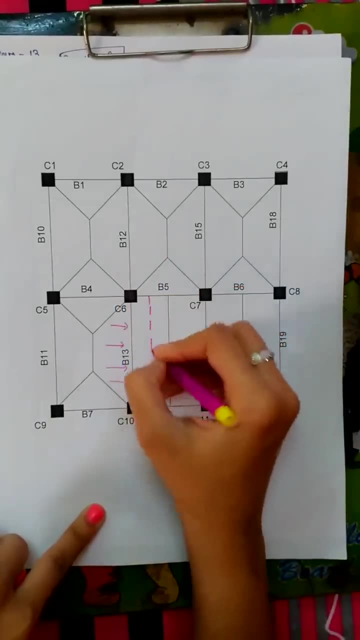 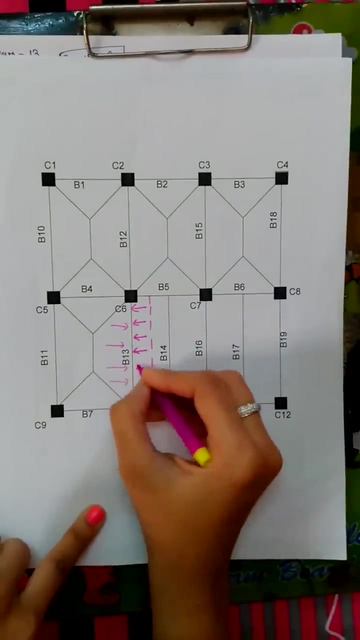 subjected with one trapezoidal load and the other side it is subjected with half of the rectangular load. You can calculate with the help of these two numbers. We have one trapezoidal load value That is 13 per meter. So you can see this: one trapezoidal load is 16 per meter and that is total. 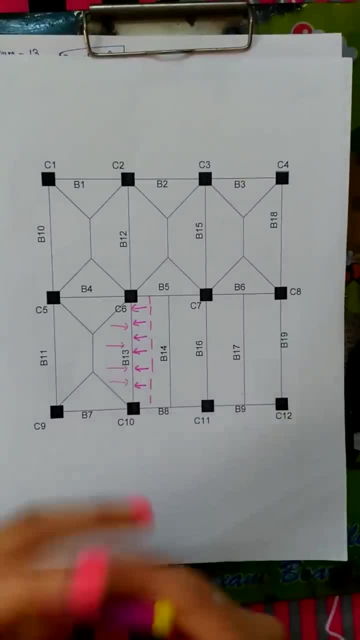 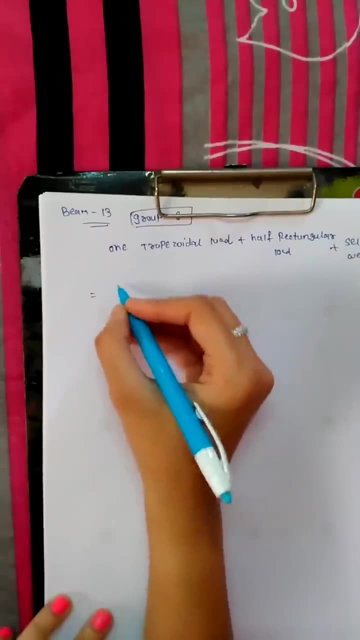 And then on the other side, this is total load from the other side And this one trapezoidal load, And this one trapezoidal load has a load value of 12.5 kilo Newton per meter. And now let us calculate. 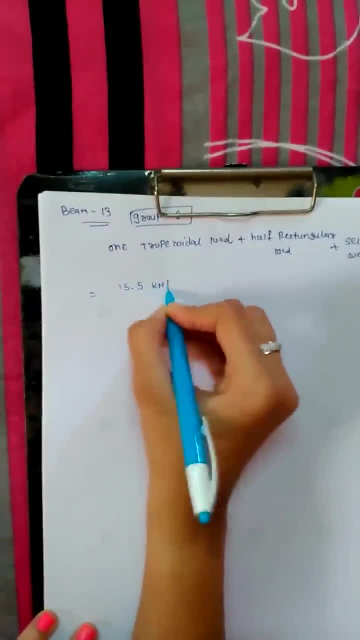 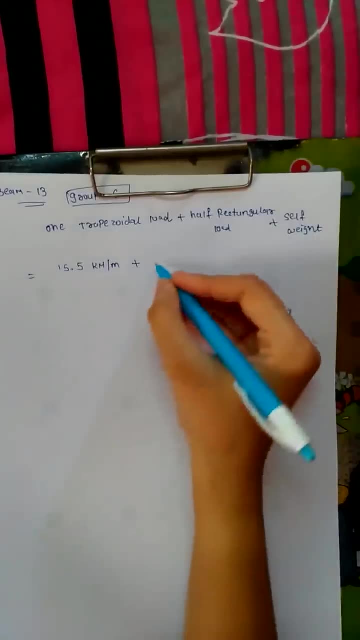 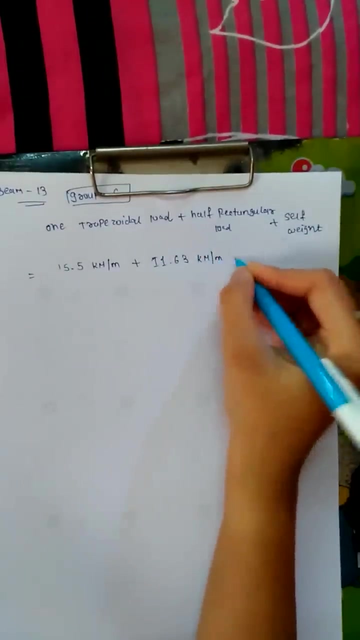 So our 1 trapezoidal load value is 15.5 kilo Newton per meter, plus rectangular load is something 11.5 kilo Newton per meter. 63 kilo Newton per meter plus its own self weight of the beam is 5.175 and it. 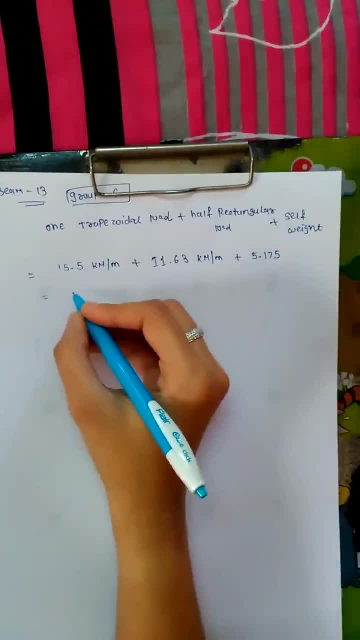 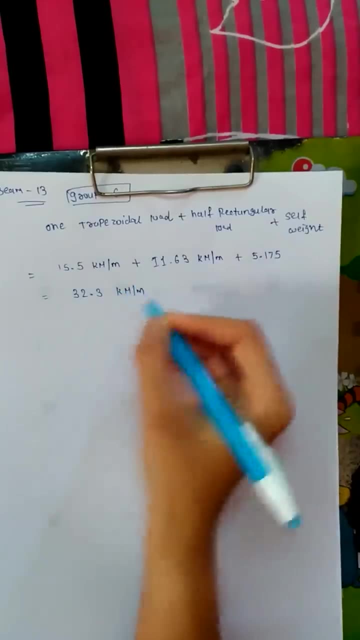 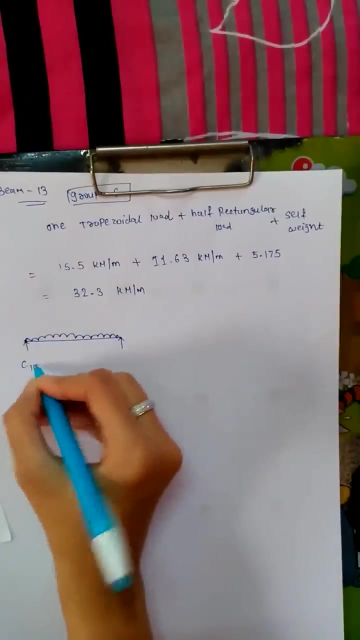 is the summation of the total. UDL is 32 point 3 kilo Newton per meter and if we are taking its beam, number 13 having supports. you can see here it is C 10 in C 6. so I'm just writing here: C 10, C 6, and both of the reaction will be W L by 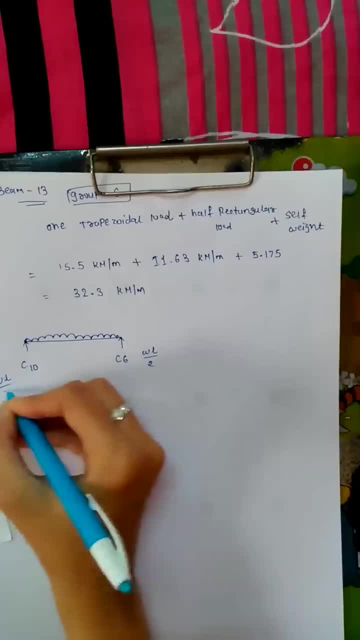 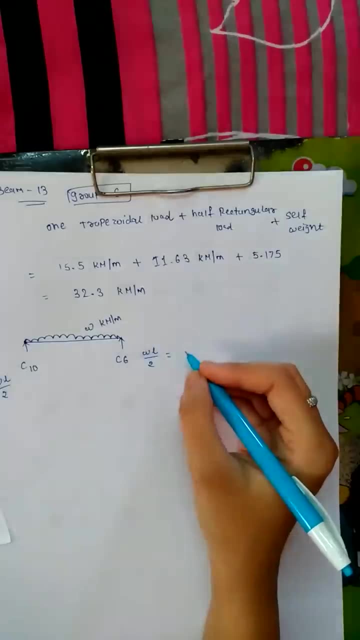 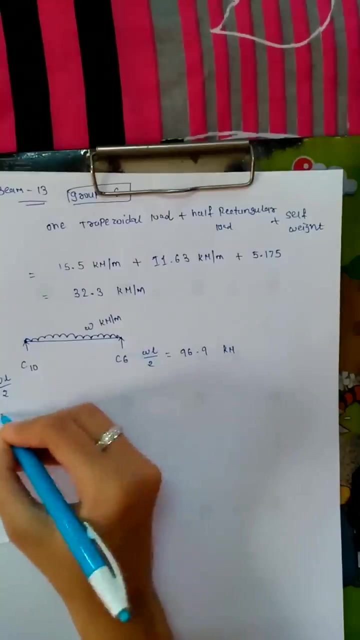 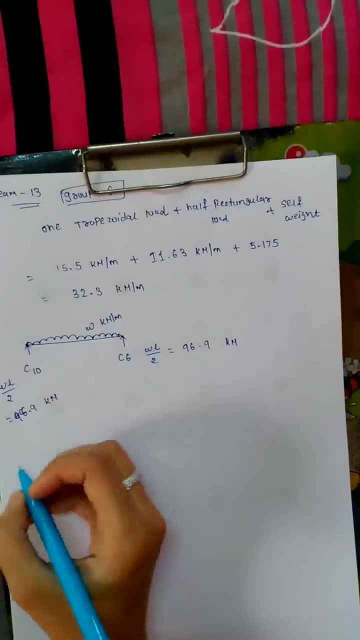 2 W L by 2, here it is total W kilo Newton per meter. so the reaction total will be ninety six point nine kilo Newton, same for the ninety six point nine kilo Newton. now let's take beam number five, beam number five having load with one. 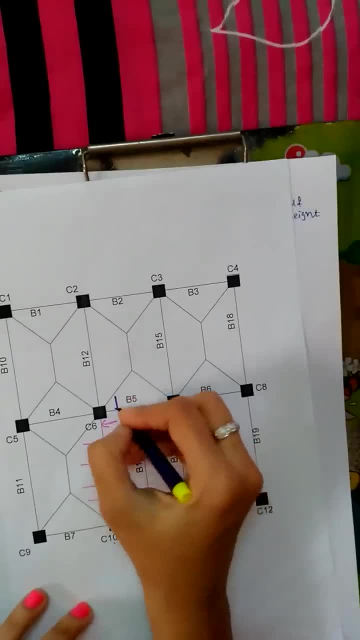 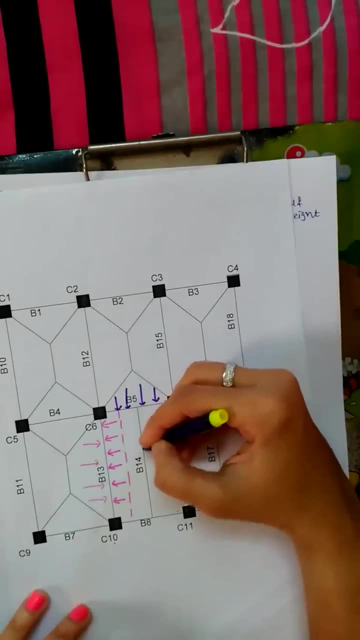 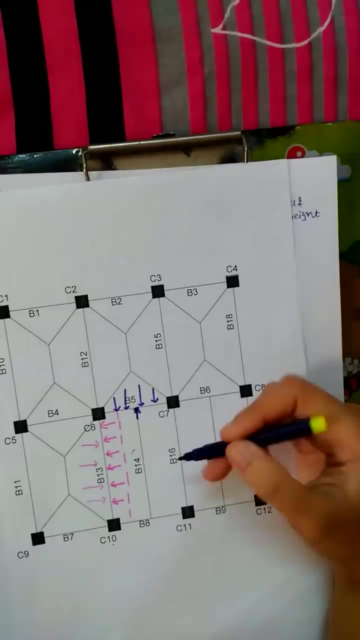 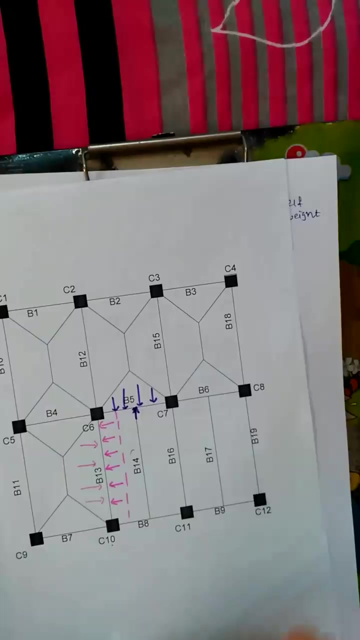 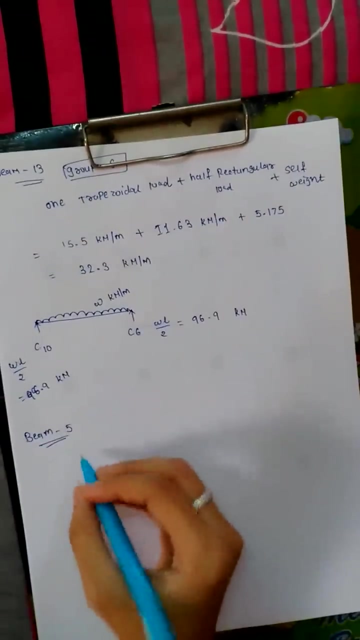 triangular load plus beam number 14. subject: there, with one point load. you can see here beam number 14 is a secondary beam and its load is transfer as a point load on the beam number five. ok, so if we are understanding beam number five having one triangular load? 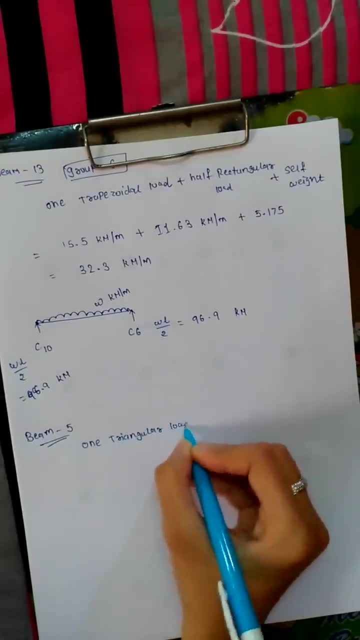 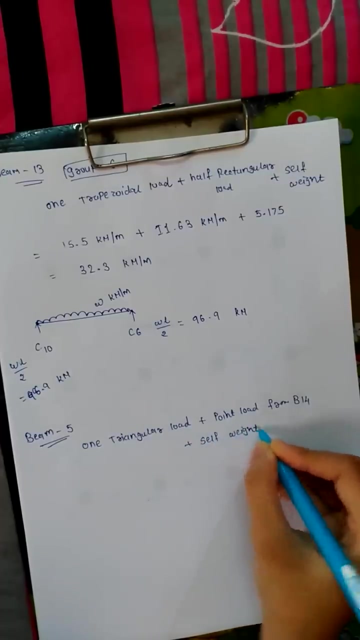 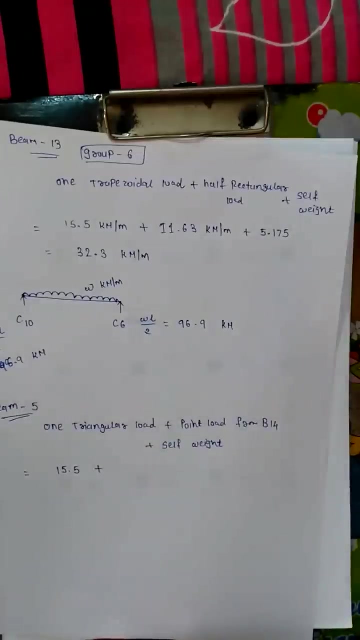 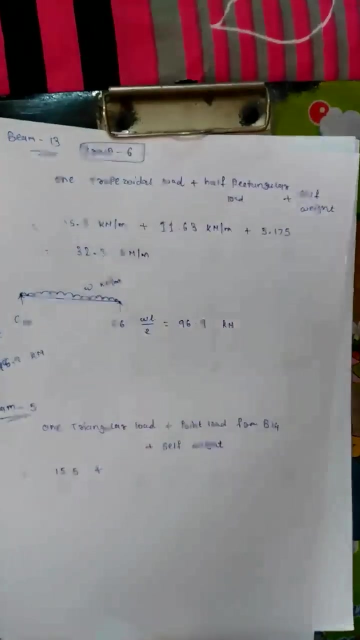 plus point load from B 14 plus its own self weight. now we have already calculated the triangular load is 15.5 plus the point load is from beam number B 14 reaction. I think we have already calculated the reaction for beam number 14 for group. 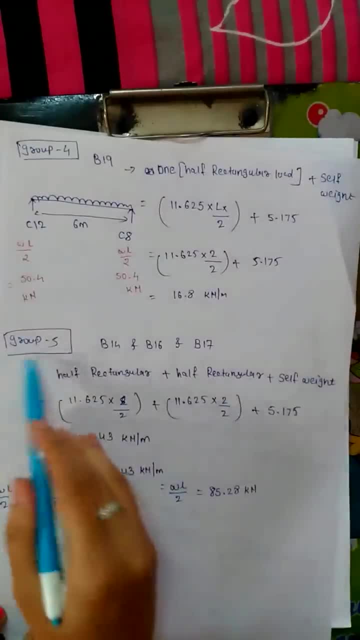 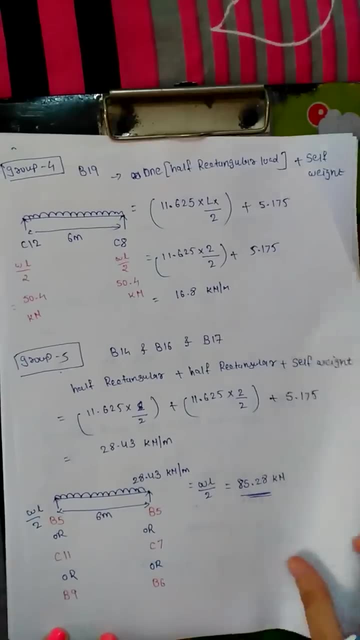 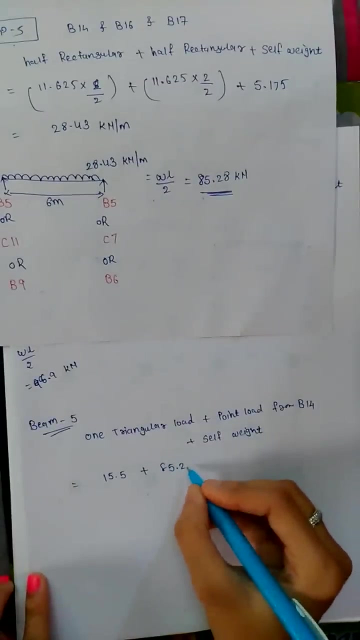 number five- and it is a reaction we already calculated- is 85.28, which is a reaction for beam number 14, and we just added 25.28 plus self weight of the beam is nothing but 5.175. so we are just adding the values. 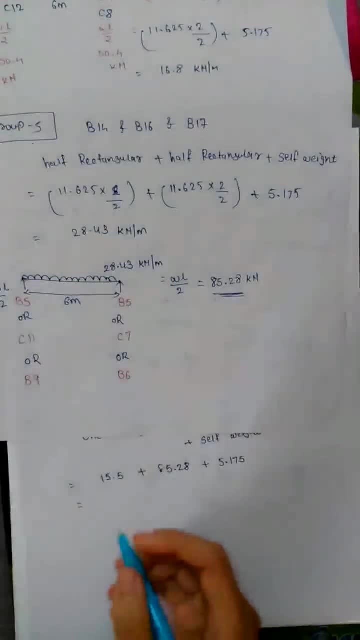 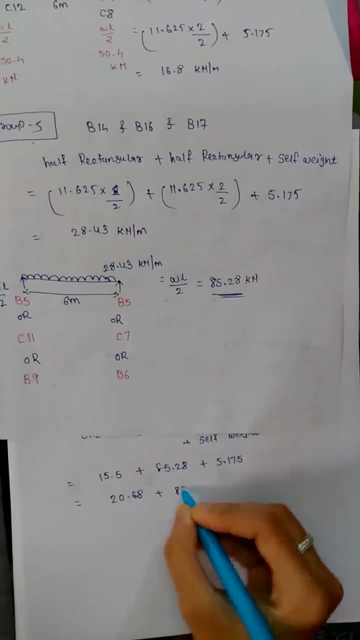 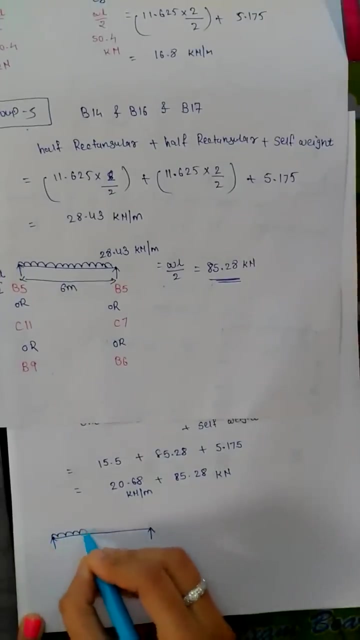 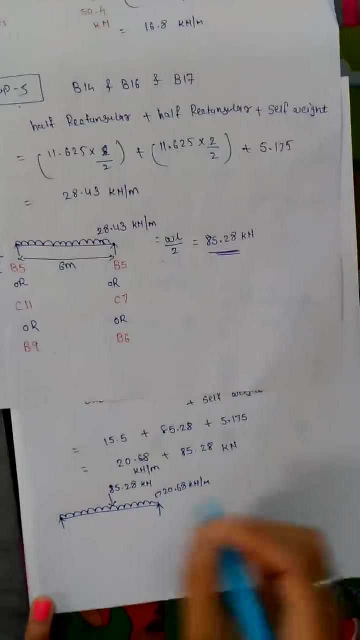 And it is the total UDL we are having 20.68, plus point load is 25.28. this unit is kN per meter, as it is UDL, and the unit of point load is kN. So let's draw the beam. it is subjected with UDL plus one point load, centrally loaded. the value of point load is 85.28 kN and the UDL having 20.68 kN per meter, and the reaction we will get is WL by 2 plus W by 2. similarly, for the right side, WL by 2, W by 2, and we know that the length of the beam is 4 meter. 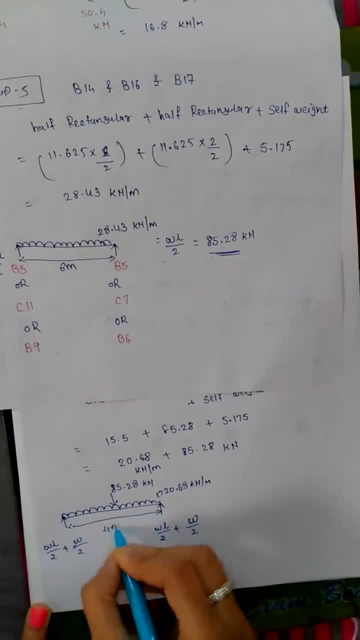 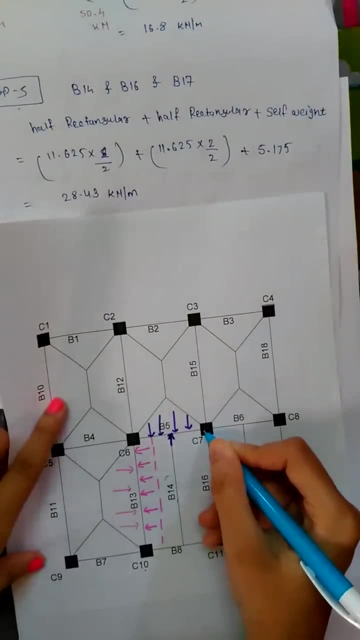 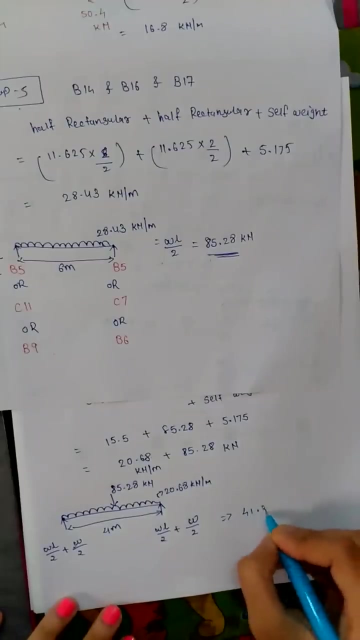 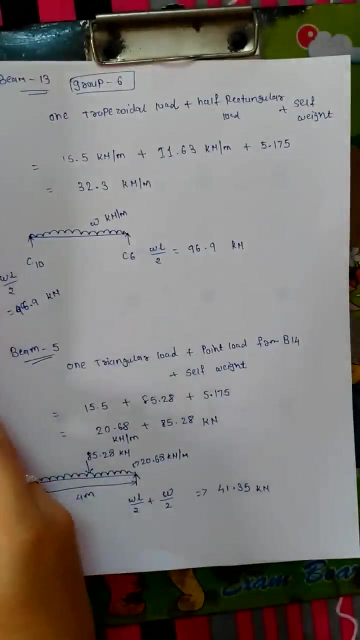 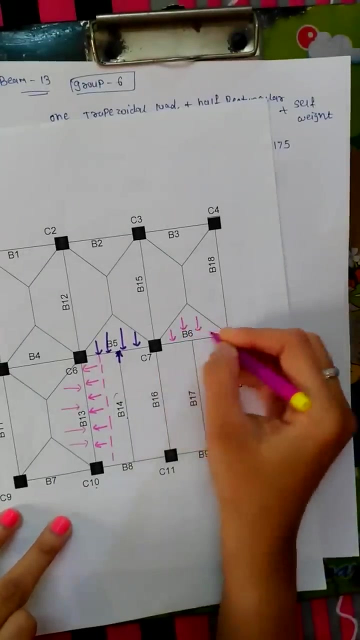 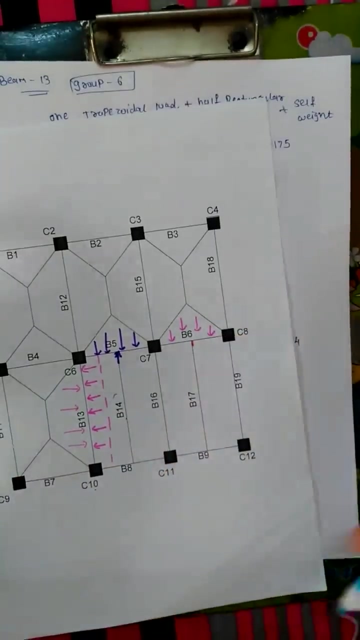 Okay, you can see this beam B5 having length is 4 meter. now we just calculate the reaction and they are 41.35, 41.35, right. so similar kind of loading is subjected to beam number B6. you can see here it is also subjected with one triangular load and one point load. so we can say that it is another group which is for beam B and beam number 5 and beam number 6.. 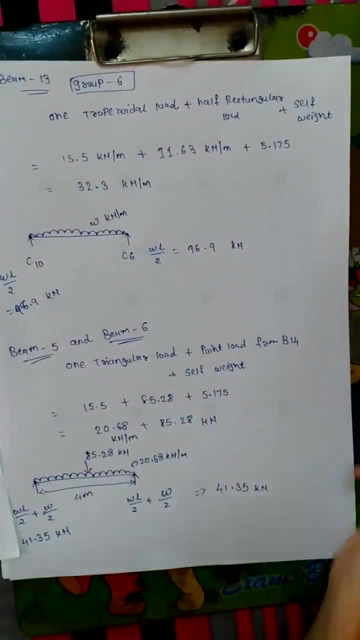 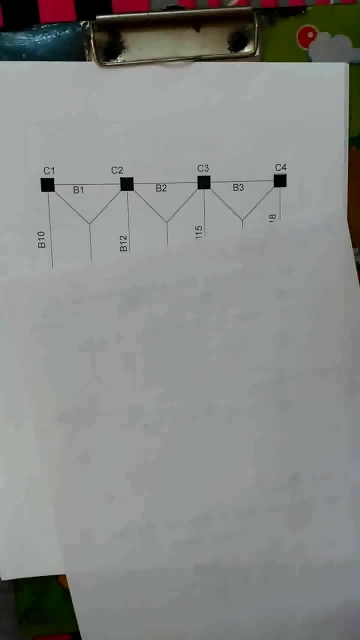 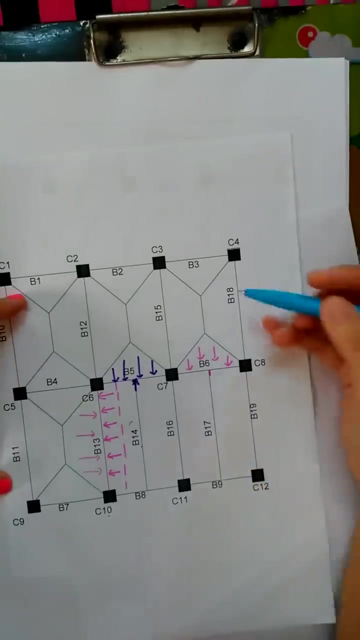 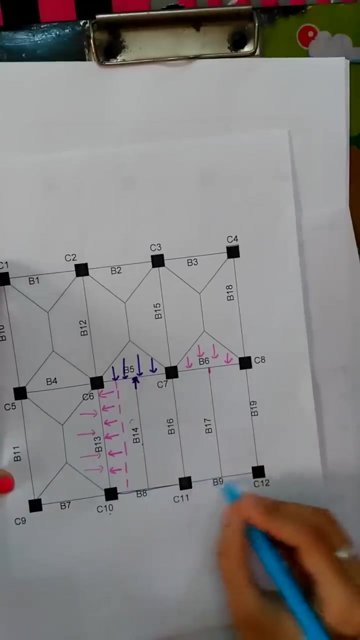 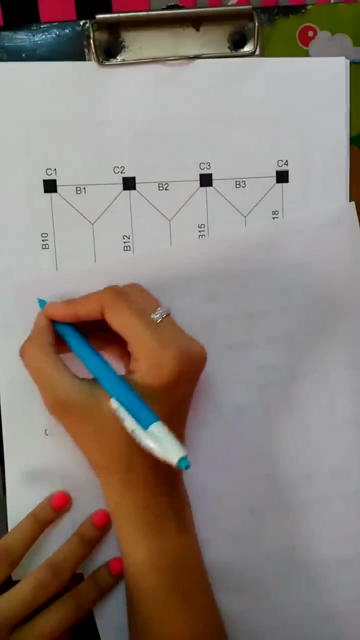 Now let's talk about another group, and they are, I think, other remaining. So if I'm not wrong, it is beam number 8, beam number 8, beam number 9, then beam number 12 and beam number 15. so let's calculate the load for beam number 8 and beam 9.. 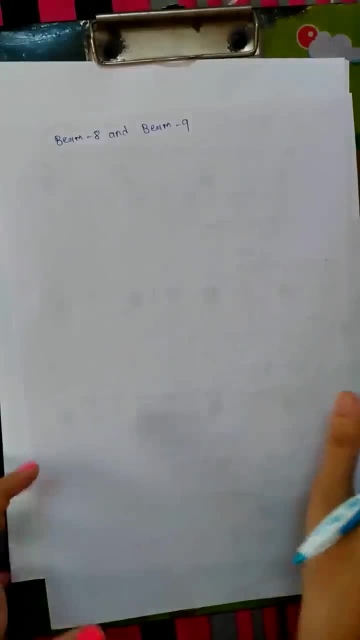 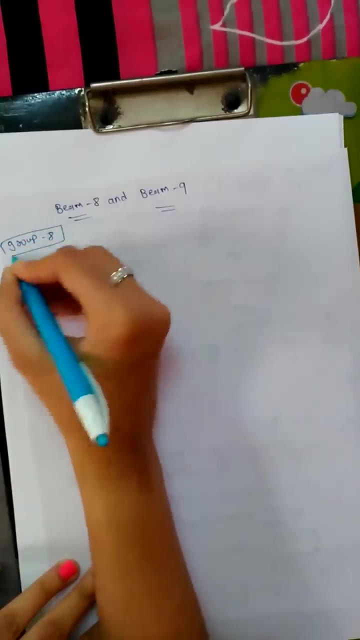 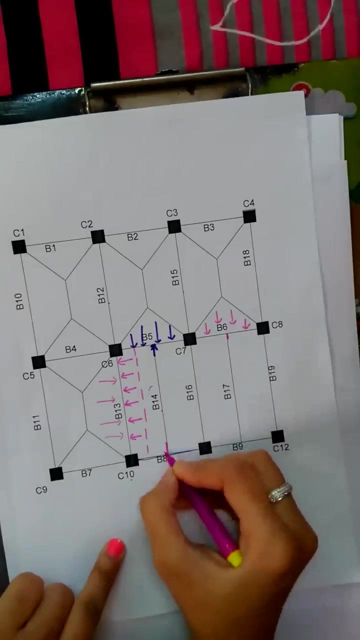 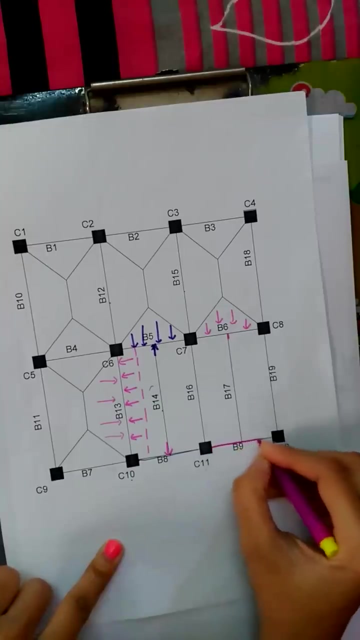 So I think it's a group number 8, so we can say that a beam number 8. it is subjected with only one point load, the reaction coming from B14, and similarly, beam 9 is also subjected with only centrally point loaded, which is a reaction coming from B17.. 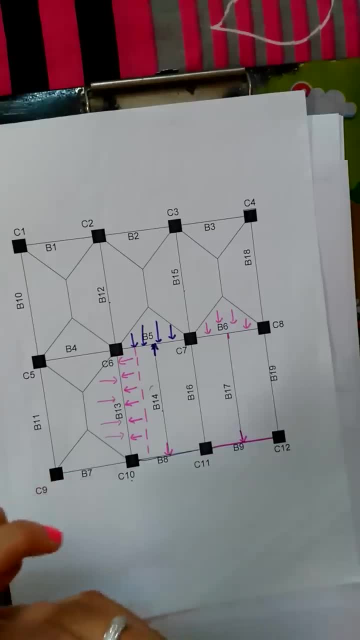 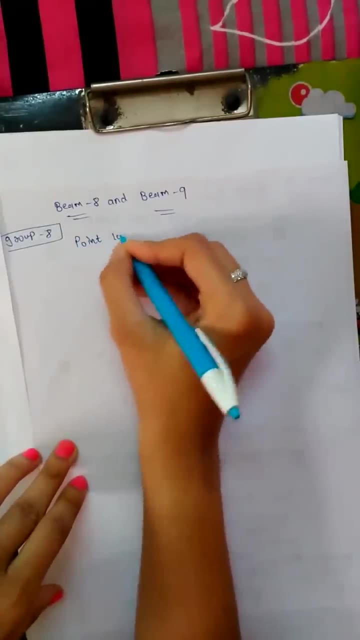 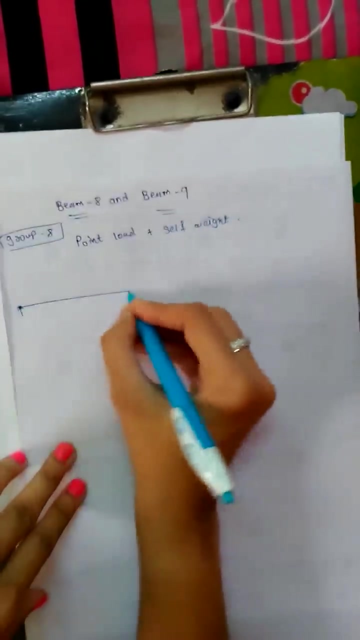 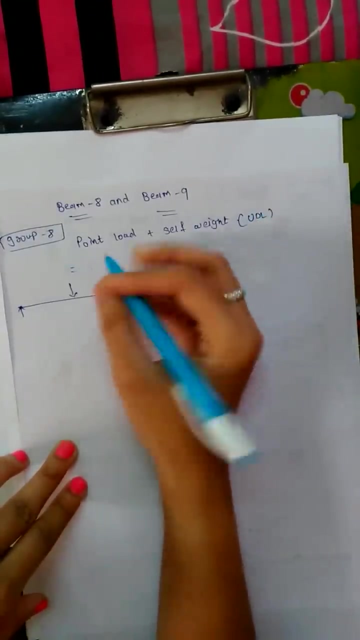 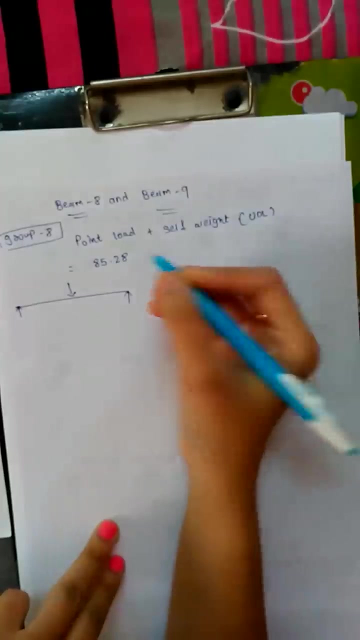 plus its own self weight is. it is always there. so beam number 8 and 9 subjected with point load plus self weight. okay, I think self weight is its UDL. so the point load value is 85.28 kilonewton plus 5.175 kilonewton per meter. 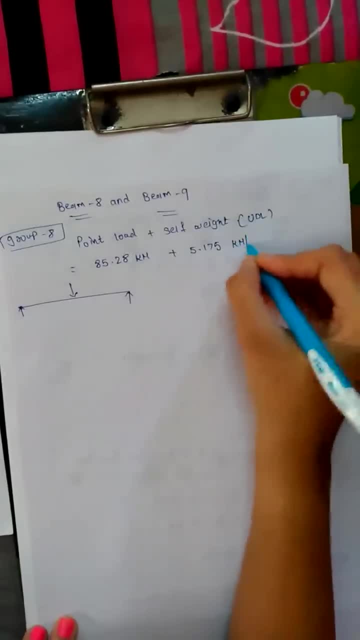 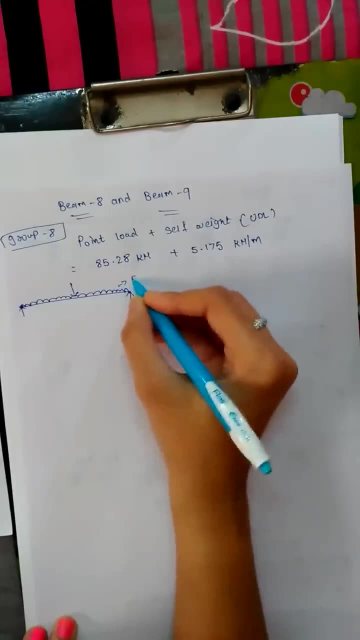 Okay, it is 5.175 kilonewton per meter and the point load is 85.28 kilonewton. and similarly I have a reaction: WL by 2 plus W by 2, again WL by 2, W by 2.. 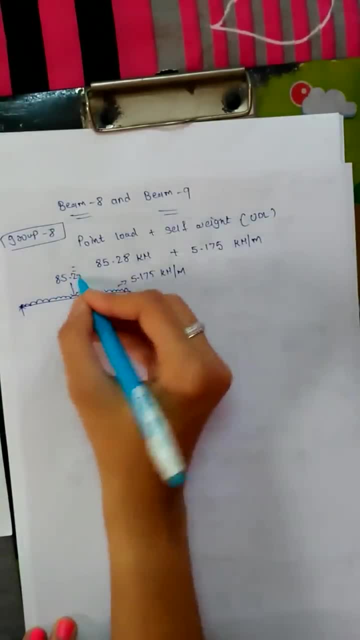 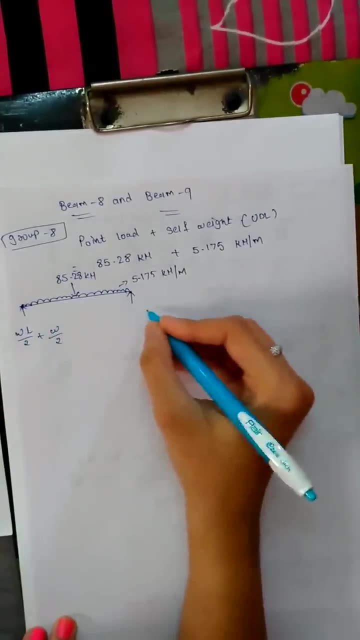 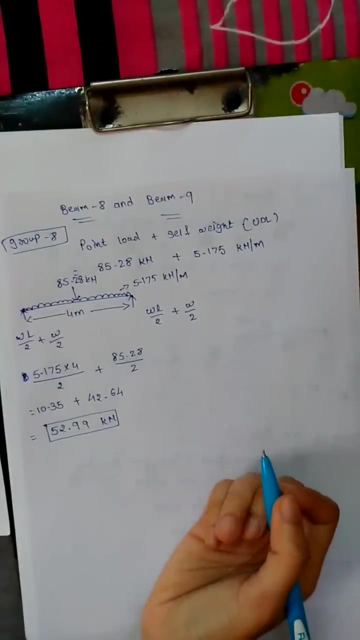 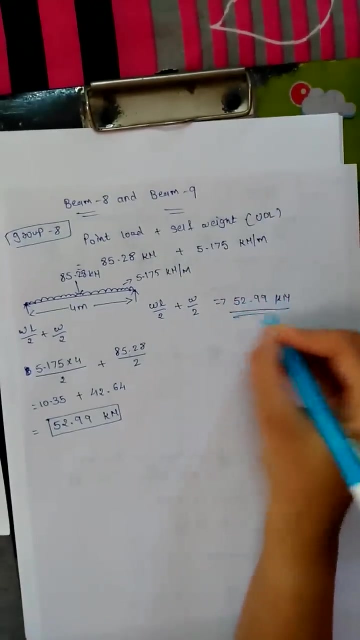 so the point load is 85.28 kilonewton and similarly I have a reaction: WL by 2 plus W by 2, again WL by 2, W by 2.. 2 and now we get the reaction for both side is 52.99 kN for beam 8 and beam 9.. 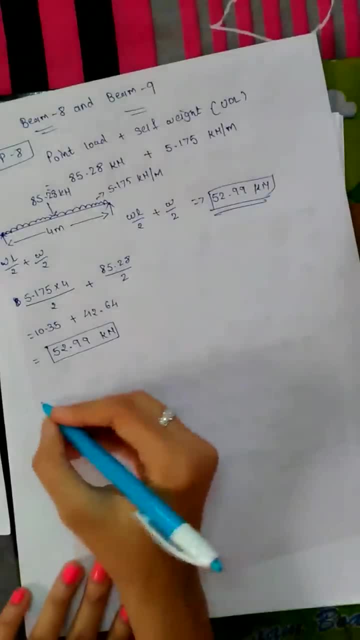 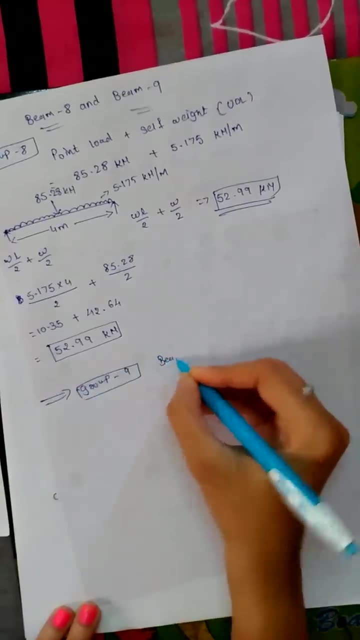 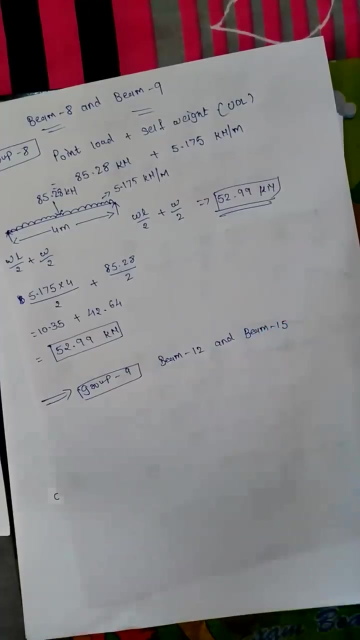 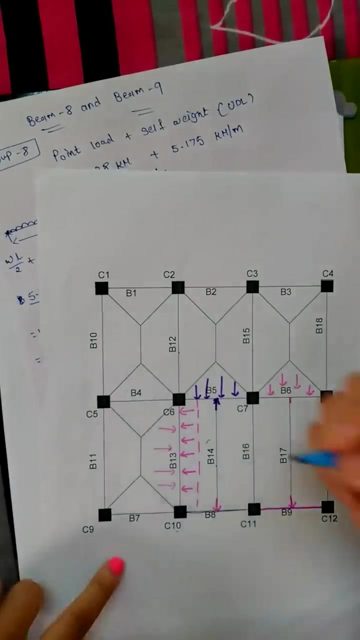 Now, lastly, talk about group number 9, and they are for beam 12 and beam 15.. As per the our plan and the distribution of load we can see here, beam number 12 is subjected with 2 trapezoidal load. Ok, 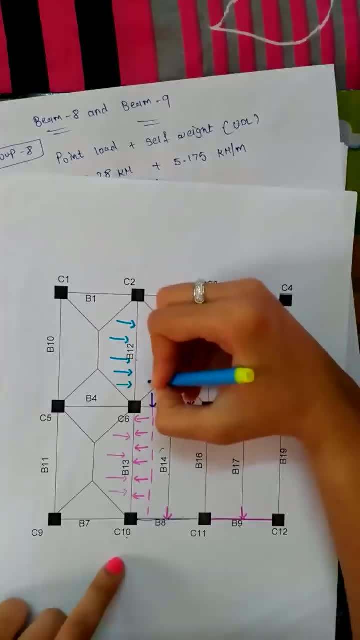 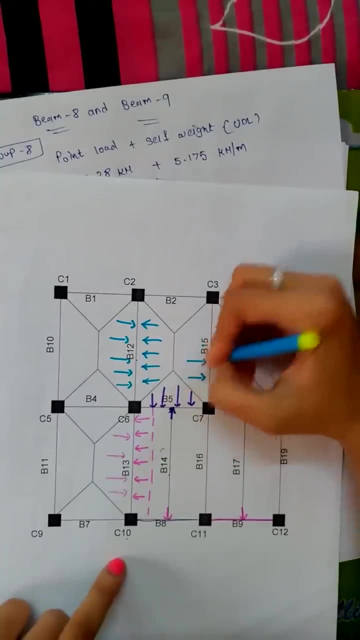 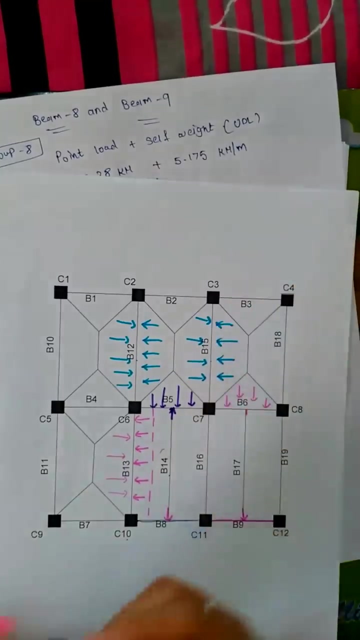 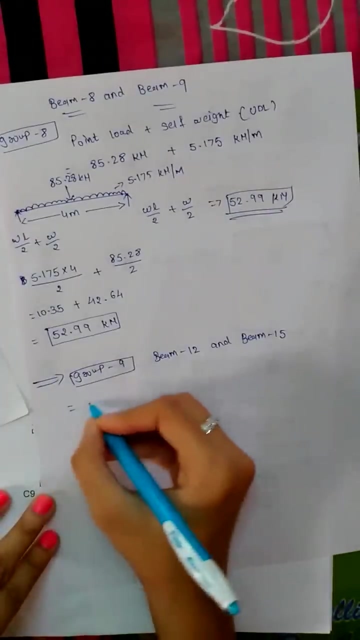 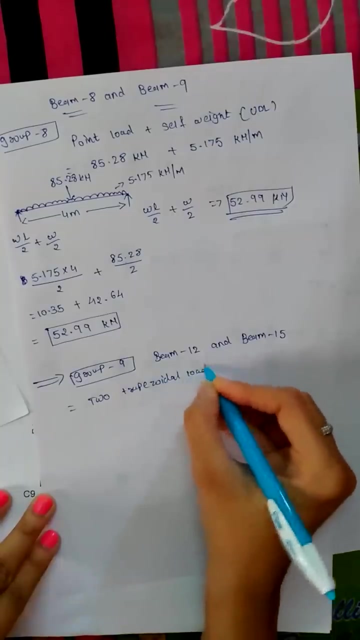 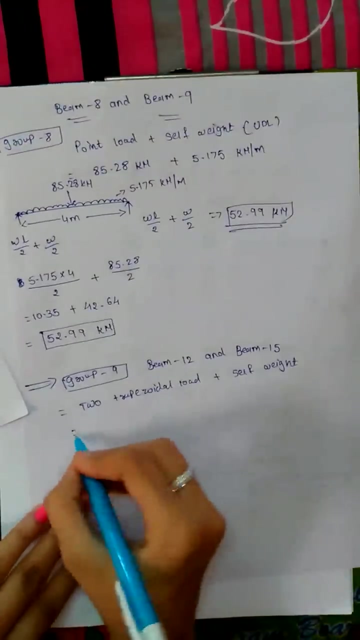 You can see by different color of arrows. ok, plus its own self weight. So let's calculate. It is subjected with 2 trapezoidal load Plus 2 self weight, And we know that trapezoidal load is 15.5 multiplied by 2 plus the self weight is 5.175. 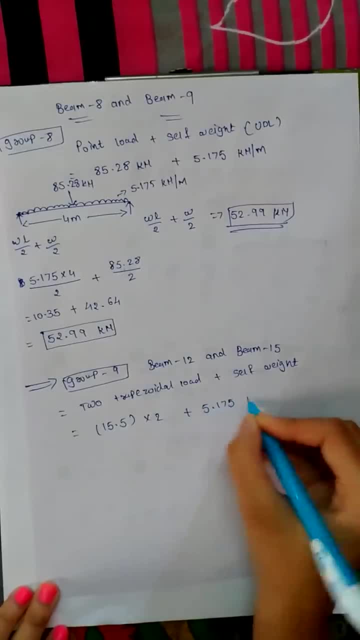 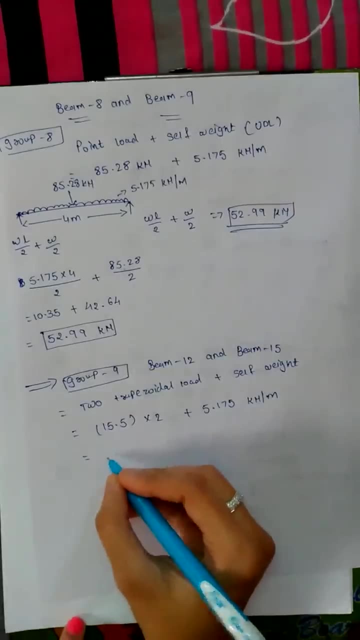 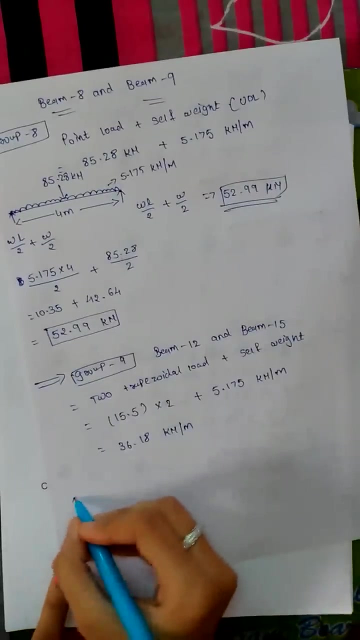 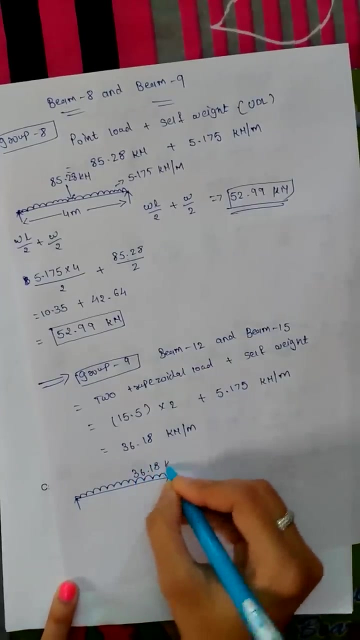 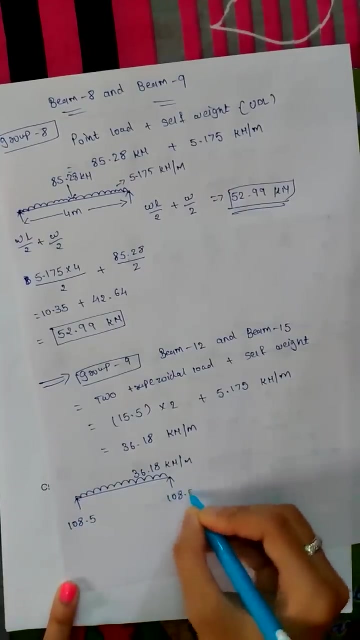 kN per meter and the total load is something 36.18 kN per meter, If I am not wrong. let's just draw: It is 36.18 kN per meter and the reaction we can get is 108.5, 108.5 kN, kN and similarly. 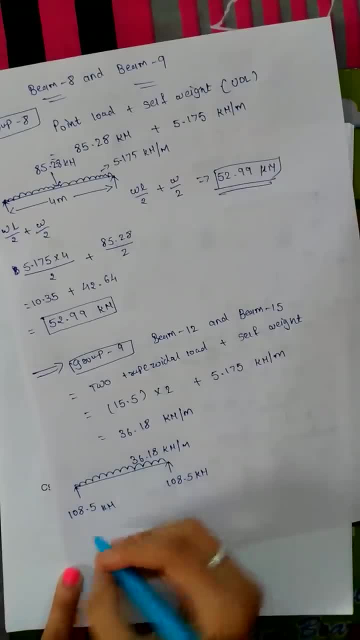 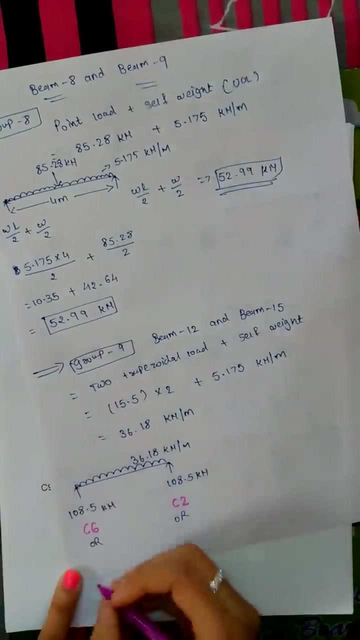 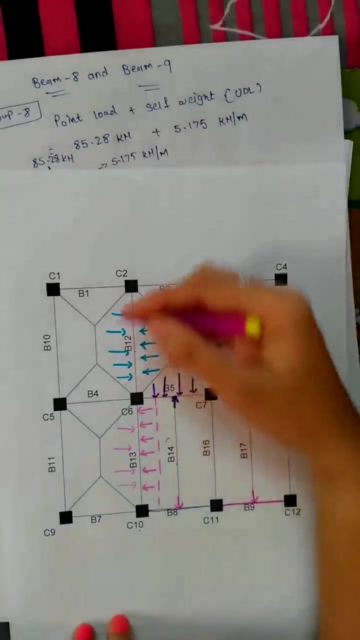 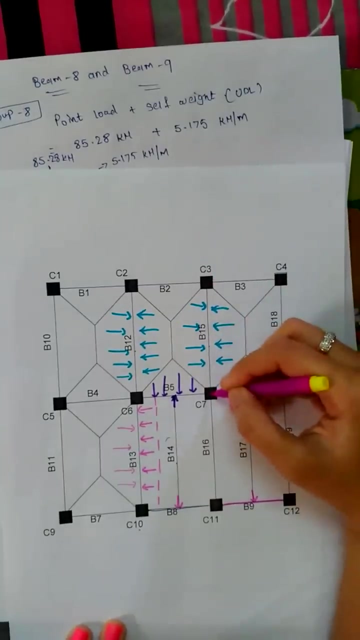 the support. supports for beam 12 and beam 15 is C6.. C2.. Ok, Ok, So it is a four or it is C7 and C3. Let's check in the drawing We are taking. supports for B12 is C2 and C6 and for B15 it is C3. 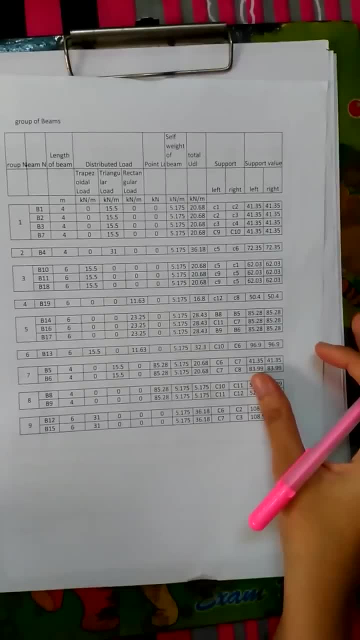 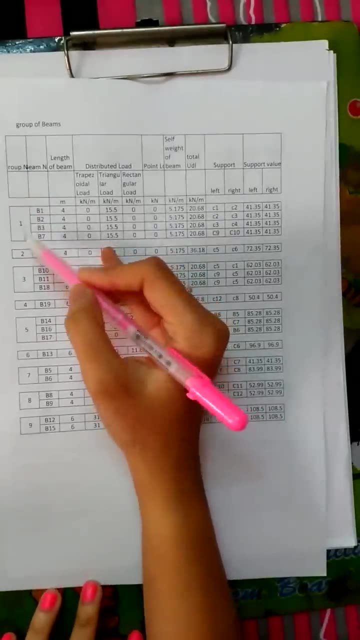 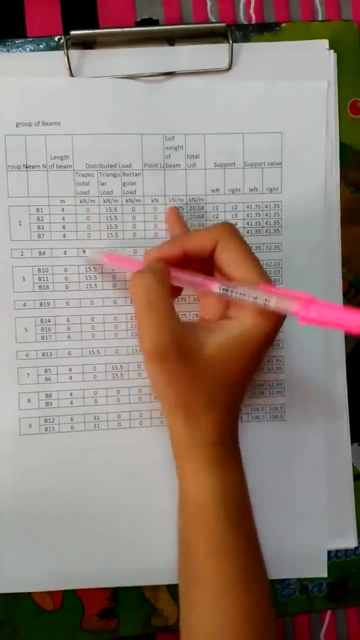 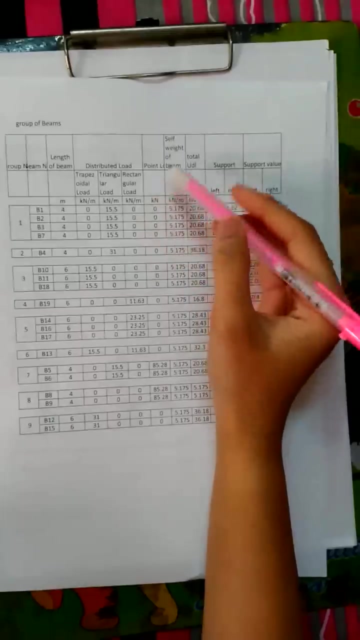 And C7.. Here I have prepared a table Which contains number of group of the beams, with name of a beam, with length, if it is subjected with a trapezoidal load. if it is, if it is subjected with triangular load, may be rectangular plus its point load, plus itself it, and it is total UDL. 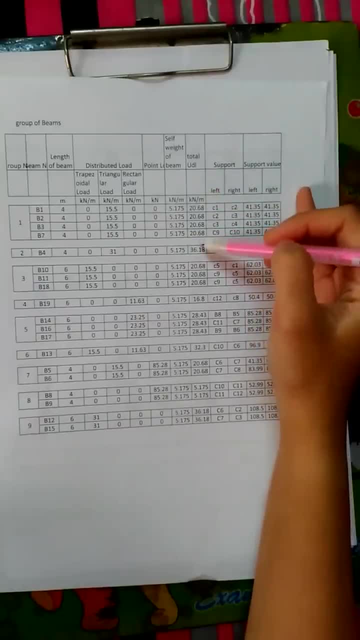 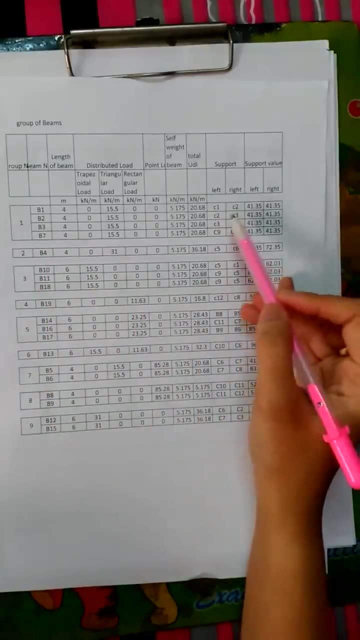 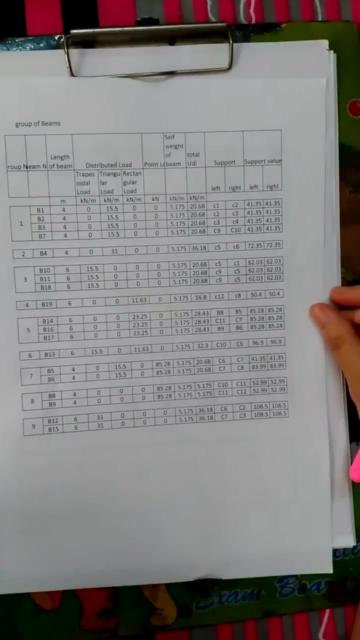 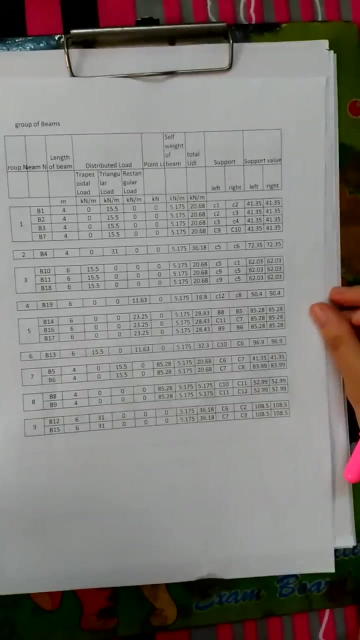 including supports, and which of the beam having which of the support from the right, right side and left left side, and the reaction. okay, you can see here the total beams having the distributed loads from the slabs. okay, and now, whatever reactions we are getting here for all, for the beams, which are nothing but the 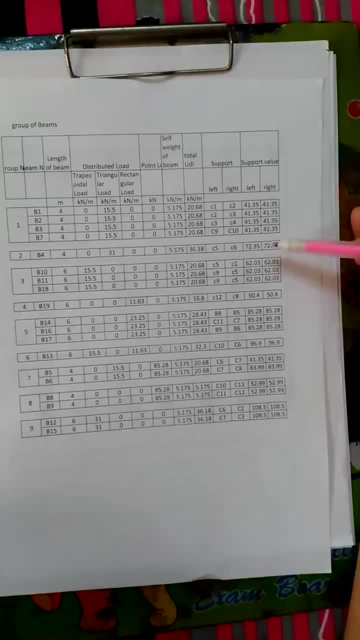 axial load which I we can say they are acting as an axial load on the columns and so far we can get approximate axial loads and so far we can get approximate axial loads and so far we can get approximate axial loads on the columns. I think we can also indicate like this: if I'm taking beam, 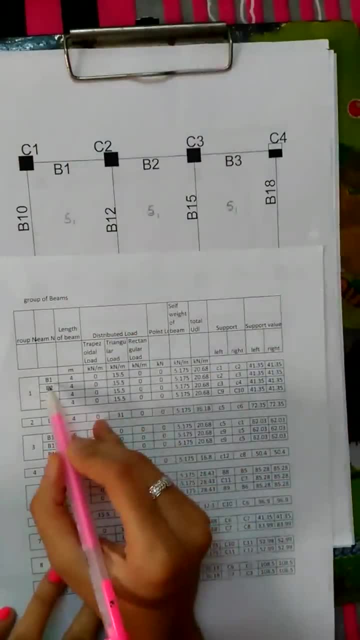 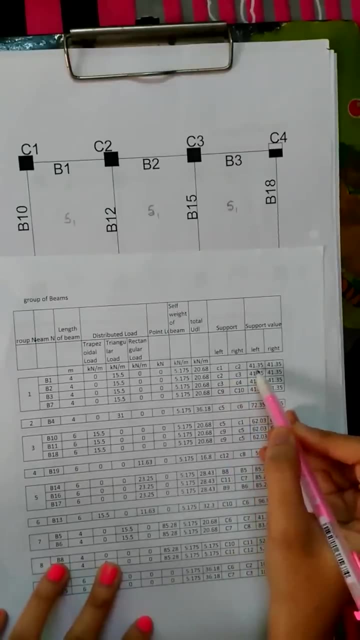 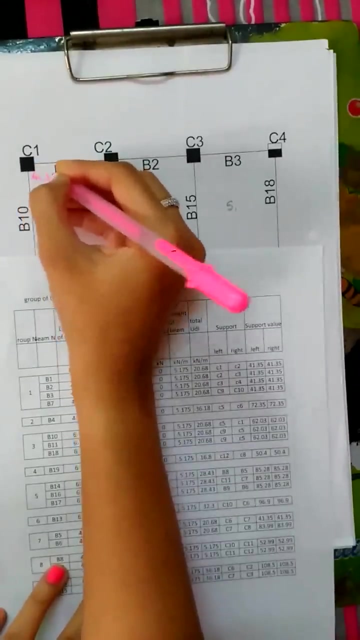 number B 1, which is having left side C 1 and C 2 having the reaction is 41 point 35. so I can write here: it is 41 point 35. similarly for C 2 it is 41 point 35, same if I am taking beam number B 2. B 2 having a. 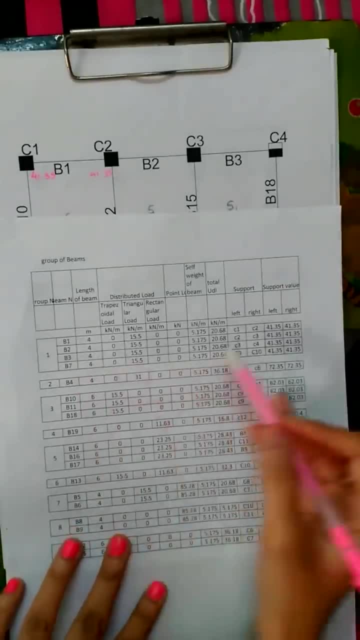 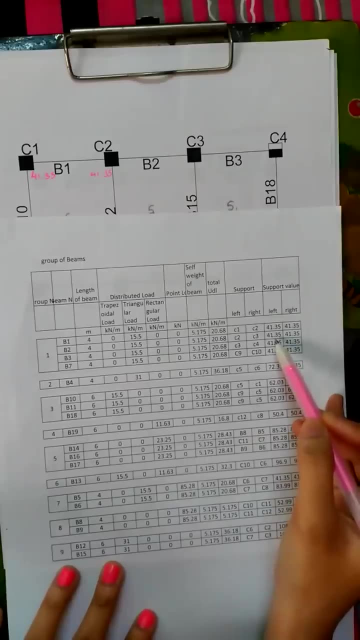 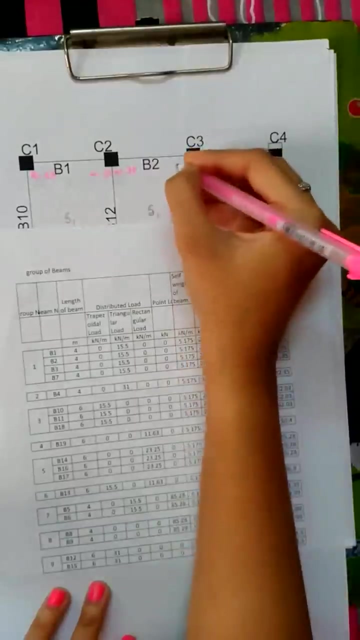 support C 2 and C 3 and same. it's a load. reactions are to 41 point 35 and 41 point 35. 41 point 35, 41 point 35, same if we are taking beam number B 10, it also having support with C 1. so let's find: for B 10 the support is C 1 and C 5. okay, so the beam number B 10, it also having